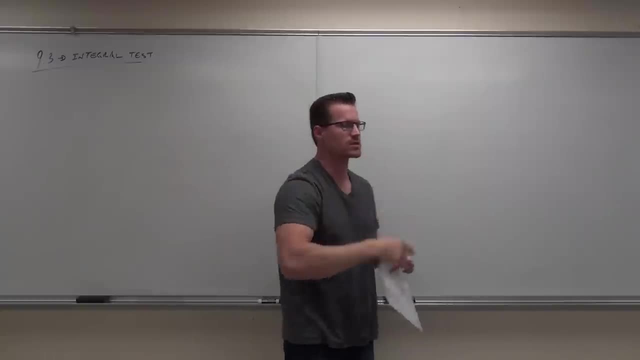 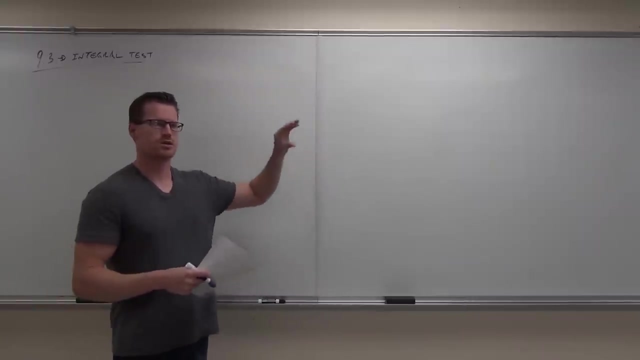 If you add up little area rectangles, well, that's an integral. That's what that means. So we're going to use an integral to say whether or not our series is going to a finite number, or whether our series is going to an infinity or whether it diverges. 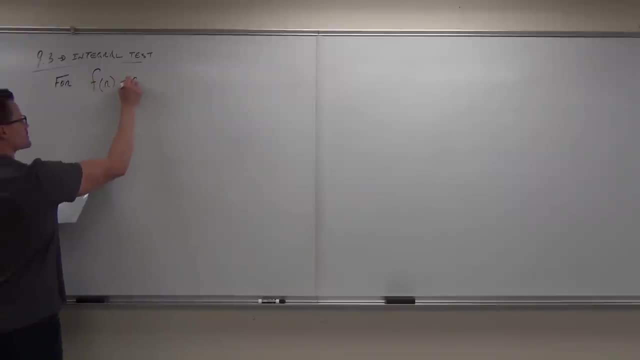 We pretend that our sequence is a function. Now I'm going to use x's in just a little bit. I'm just kind of giving you the brief outline here. So we let our sequence so the terms of our series. that's our sequence. We let our sequence be represented by some. 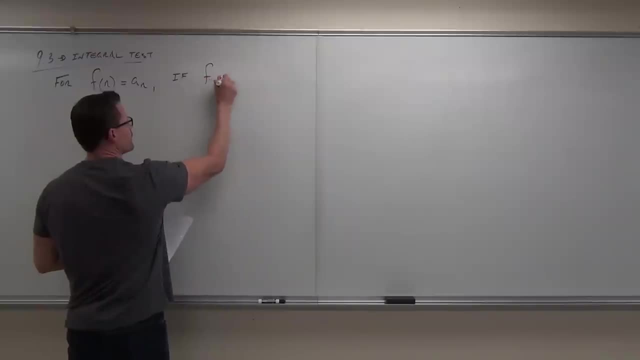 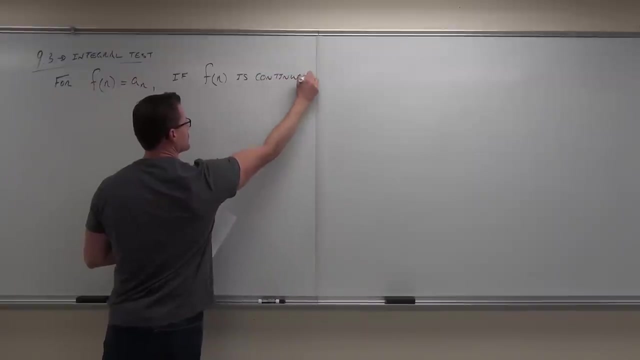 function. We say if f of n is continuous, It's got to be continuous. It's got to be continuous. It can't have any breaks. It can't go to infinity like this. It can't do that, It's got to be. 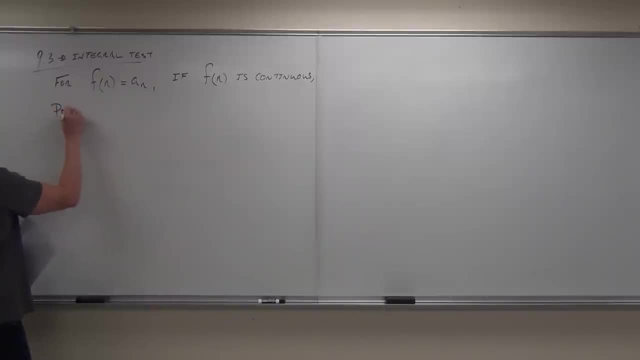 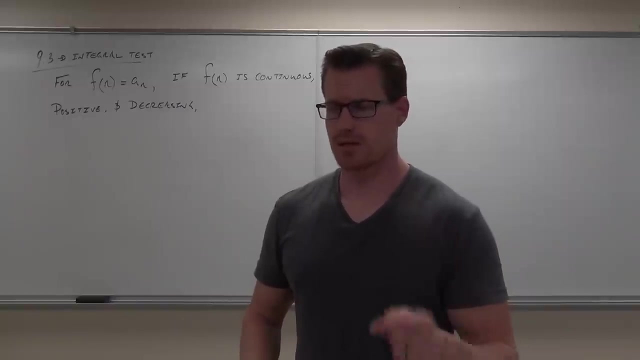 continuous. It's got to be positive And it must be decreasing. But if the function that we're using to represent the sequence from where we're getting our series is continuous, if it's positive, then it's continuous. If it's continuous, then it's continuous. 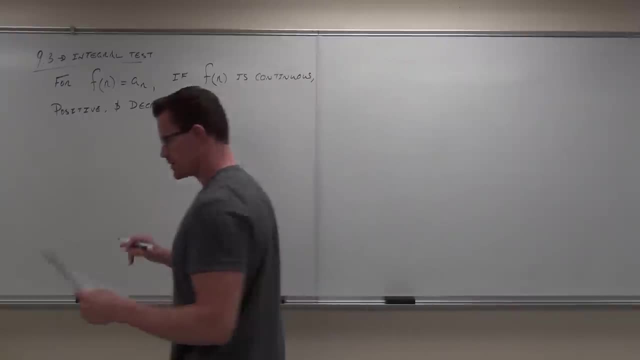 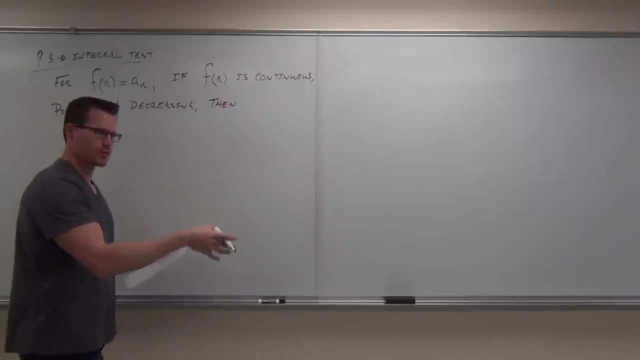 If it's continuous, then it's continuous. If it's continuous, then it's continuous. If it's positive and if it's decreasing, then we can use that integral to show convergence or divergence of our series. So, basically, then, this and this. This is where I'm making. 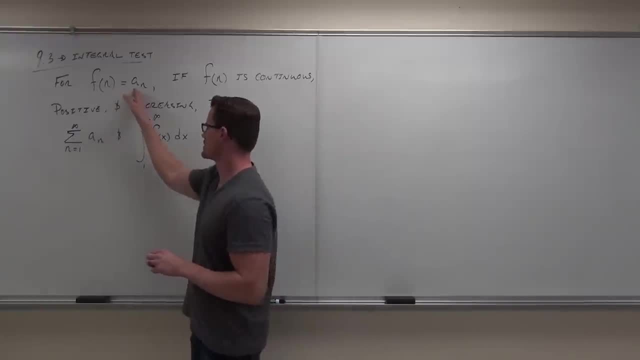 the difference. So I know I said f of n because it's based in terms of n, but really this would be a function in terms of x, Just like we did before. I forget what we did with that. We used a function in terms of x with a sequence before. We're going to do basically the same. 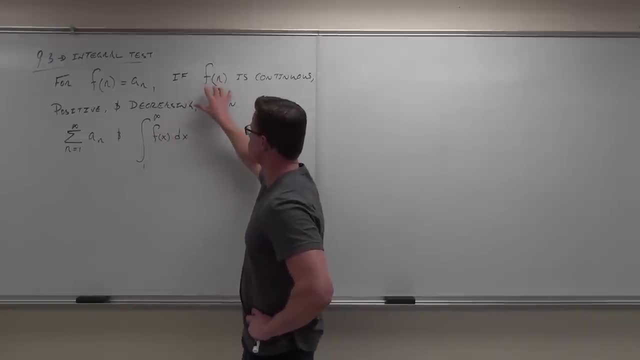 thing. here We say: hey, if this is true, if this function is continuous positive and decreasing, then this series of a sub n and this integral of f of x from 1 to infinity- if we start with 1 and go to infinity, then this integral will have the same result. 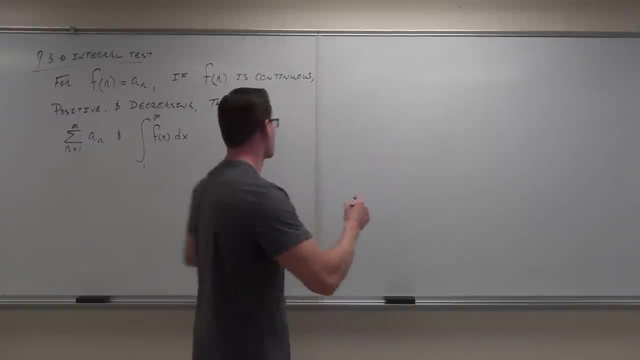 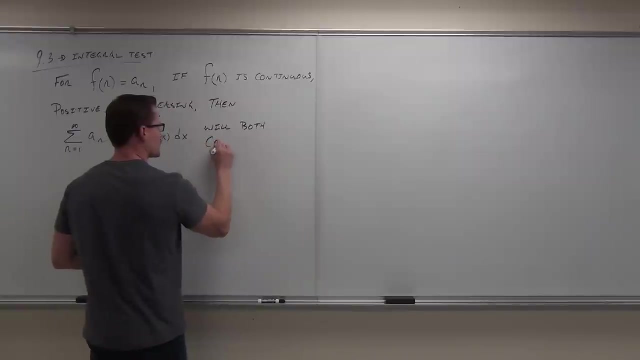 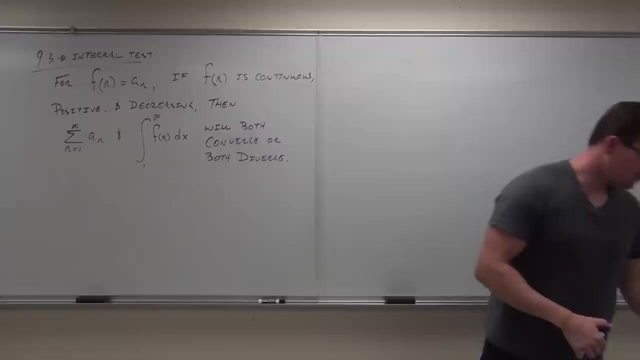 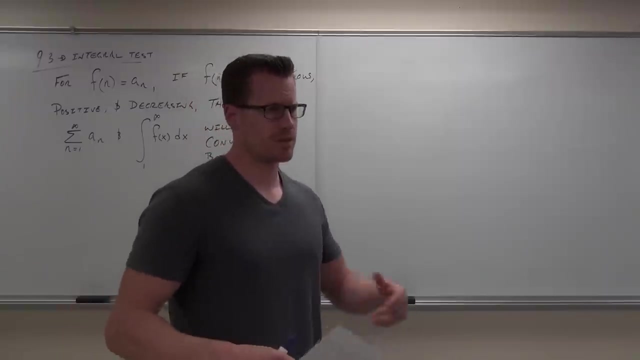 They will both converge or they will both diverge, But either way they will have the same result. So practically what we're doing is we're checking our integral to find out something about our series, which is a really nice idea. Again, the really basic idea is: well, integrals, add up stuff, right. 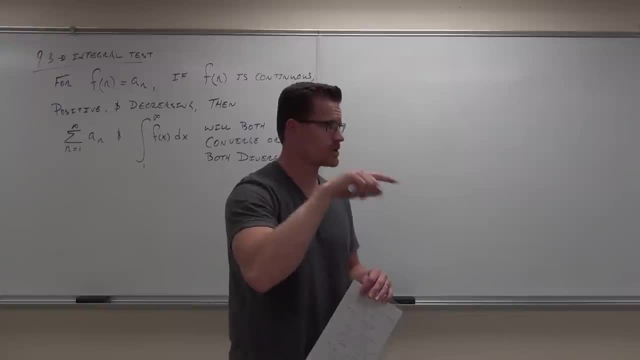 Series, add up stuff. Let's just model our integral after our series and add the stuff up. Yeah, we're not adding up everything in between because we're not talking about real numbers with our series. We're talking about just positive integers. but the idea is the same. 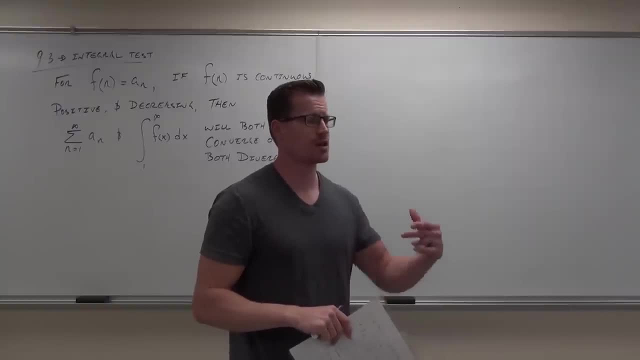 One more thing about this is the idea is the same, because I'll get to it in a minute. Another idea: practically what's happening is that our integral is acting as an upper bound for our series. That's practically what's happening If we know that our integral is going like this, so we can find the sum of this. 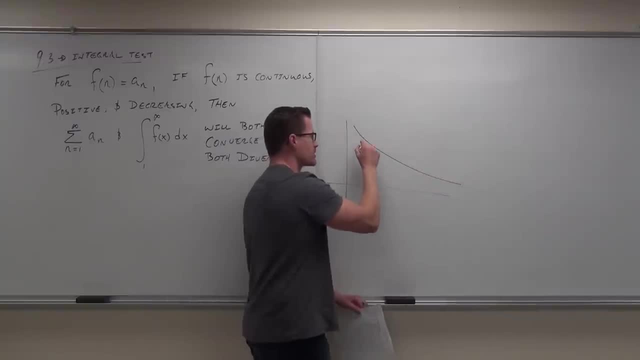 and it's a finite number, then naturally, if this is an upper bound for our series, our series is going to have to fit somewhere under here, right or on it, It doesn't matter, It doesn't really matter. But if our integral is an upper bound and that integral goes, converges, 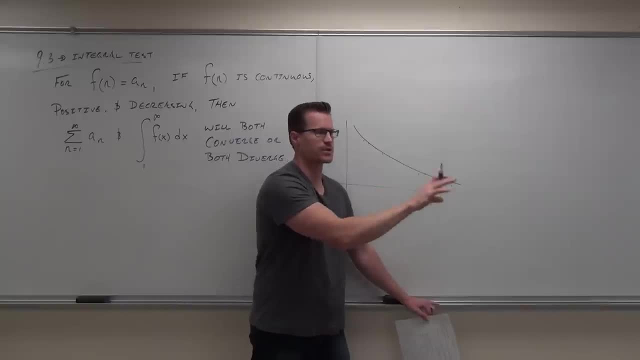 goes to an actual number. well then, our series must also The integral acts as an upper bound for our series if it's continuous positive and decreasing, So if any of you understand the concept behind this, Now a couple of key notes that I want to tell you about. 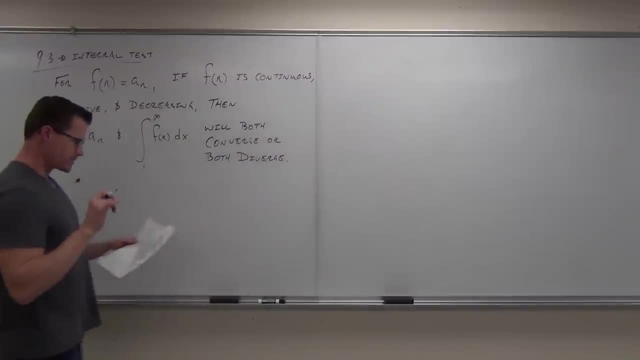 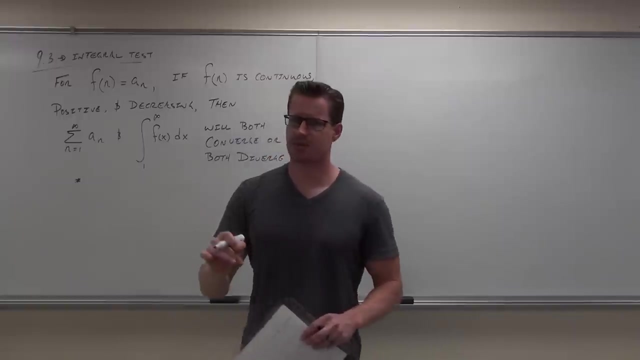 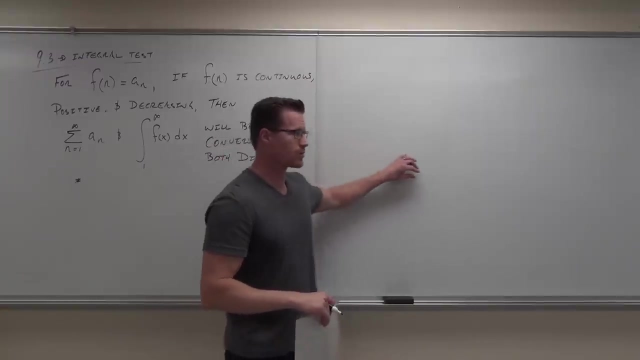 First key note: This will: This will tell you about convergence and divergence. if this is true, If this, if you make this happen, it will tell you about convergence or divergence, but it will not necessarily give you the sum. So if you do the integral and the integral equals some number, you go hey, hey, it converges. 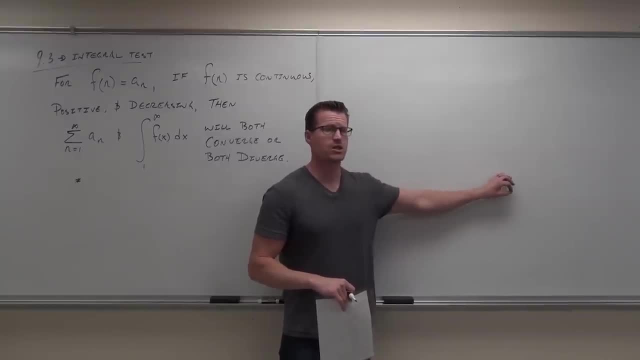 That's great. Is the number? it converges to the sum of your series? No, it's not. It just tells you that the series also converges, but it doesn't tell you what the sum is Does is. are you very clear on that? 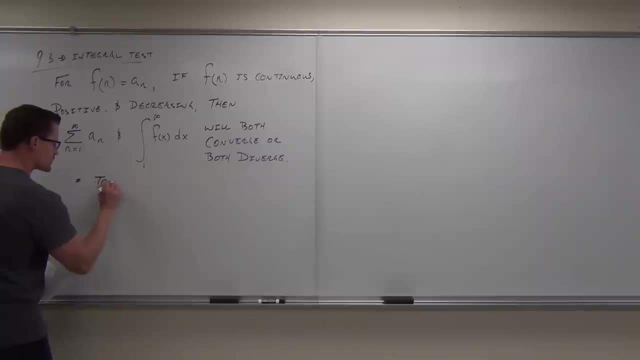 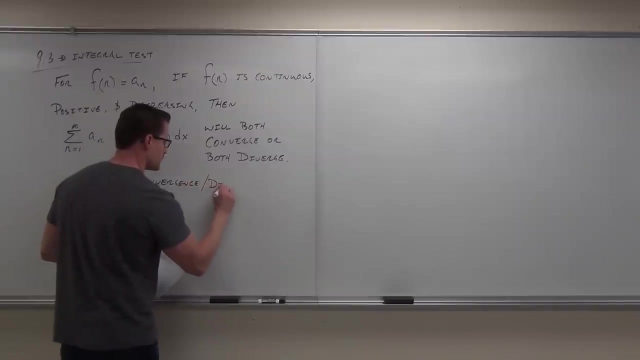 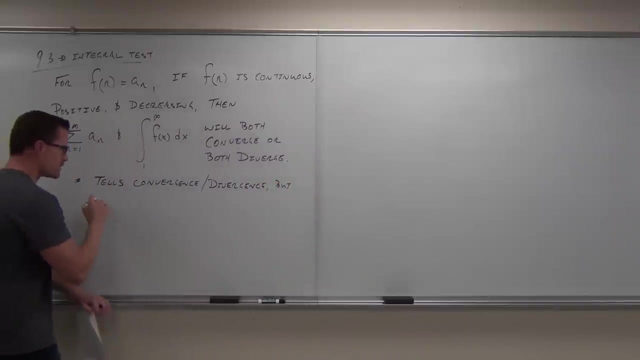 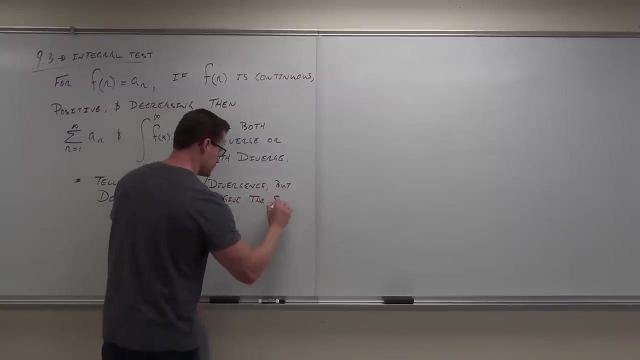 Okay, So this will tell convergence. So this will tell convergence or divergence, But it does not necessarily give the sum Of this series, That's right. Secondly, Say what It sometimes can be the sum, Sometimes, But not necessarily. 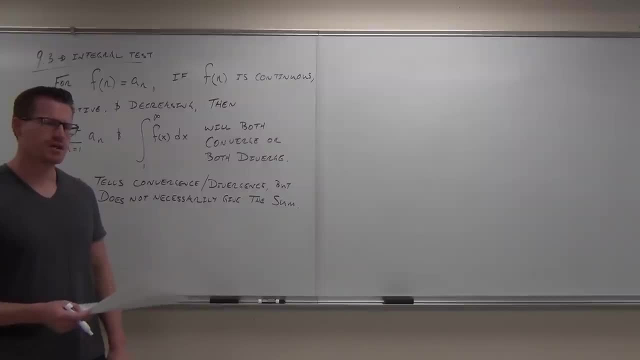 What is kind of cool And we get this from this. We can sometimes cheat at this a little bit. You see, convergence or divergence is not affected by the addition or subtraction of a finite number of terms of your series degrees. So if I take out the first few terms or add to it some terms in the middle: convergence, 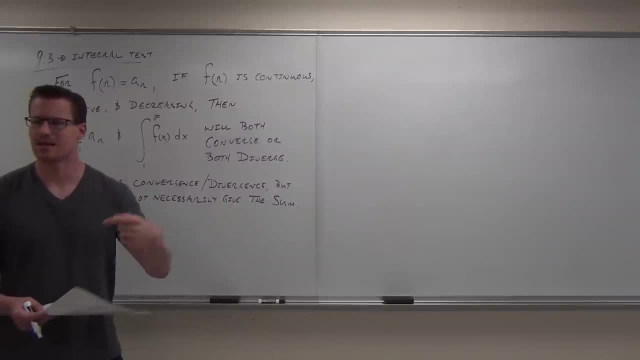 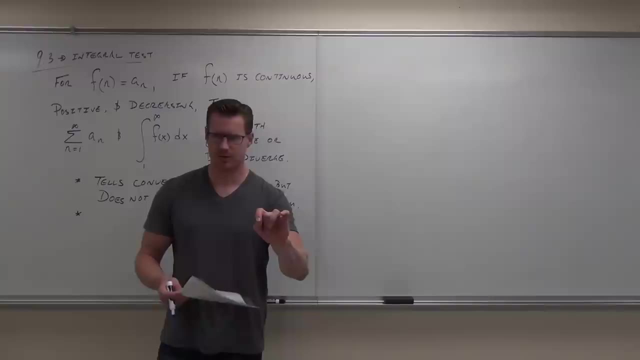 is not affected towards infinity as long as it's a finite number of terms. I can't add an infinite number. but if I say let's add five terms or let's subtract the first ten terms, the sum would be different. Are you listening? The sum would be different. 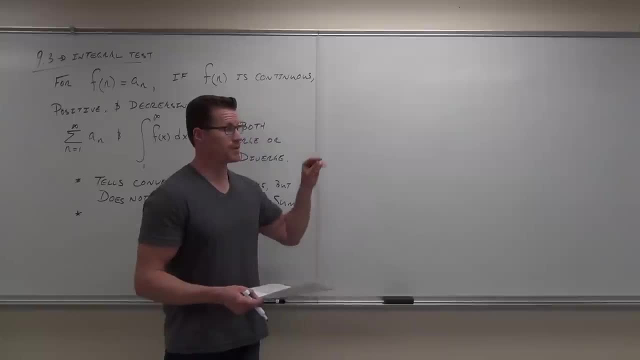 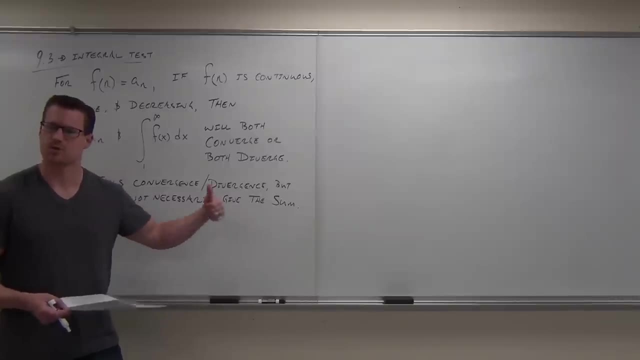 because obviously I'm adding or subtracting. Yes, it's going to be a little different, but the convergence will not be different. And since this doesn't tell us about the sum, anyway, who cares? It's going to tell us whether it converges or diverges. It's not telling. 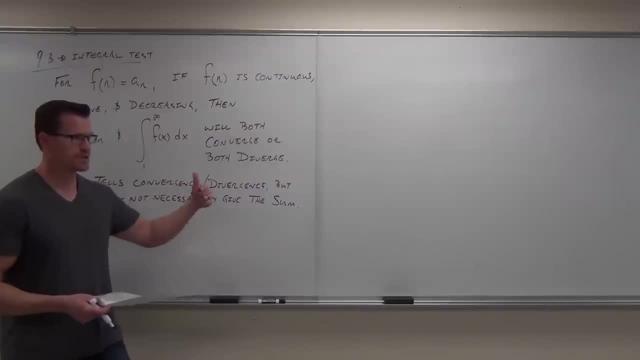 us the sum anyway. so, whether we subtract or add a few terms, to tell us whether we can go to the right number, tell us whether our integral is going to converge or not, to tell us whether our series converges or not. that's what we're looking at, So we can sometimes 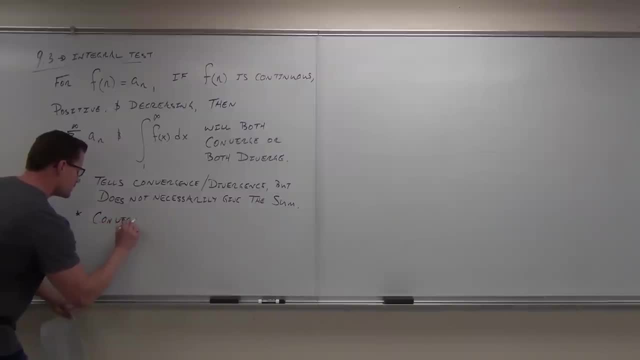 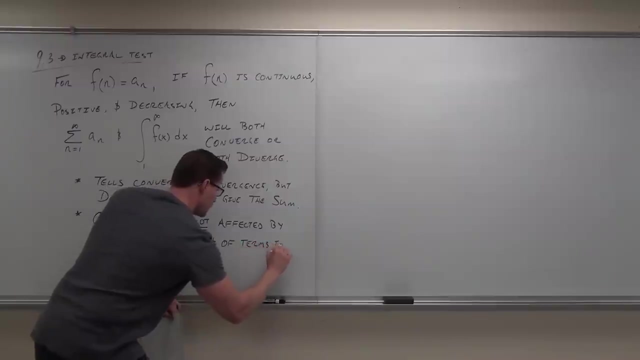 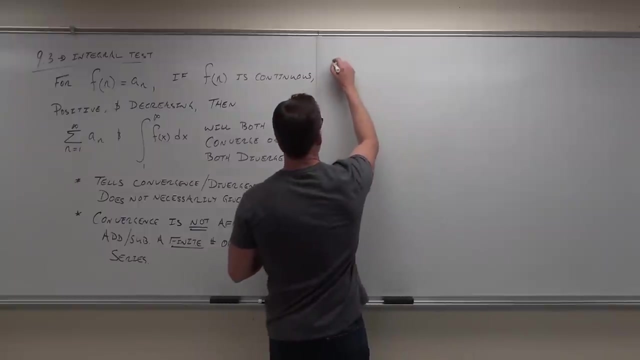 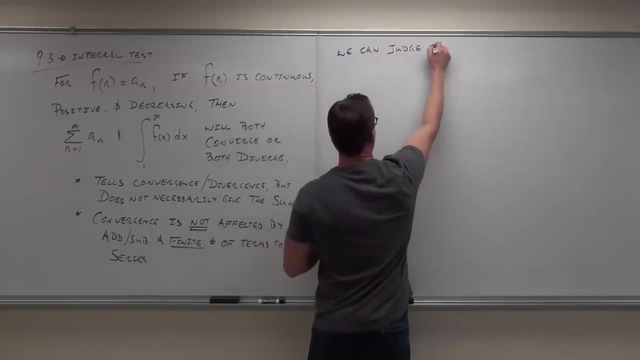 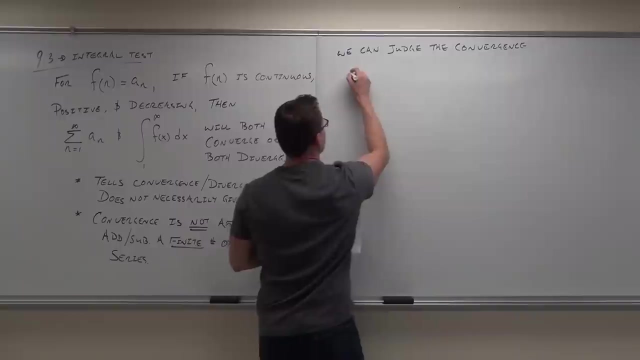 cheat at this, because convergence is not affected by the addition or subtraction of the sum. It's not affected by the addition or subtraction of a finite number of terms of our series. So, basically, here's what this is saying. It says we can judge the convergence. 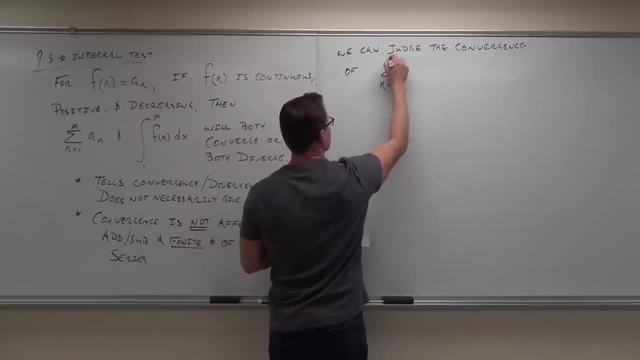 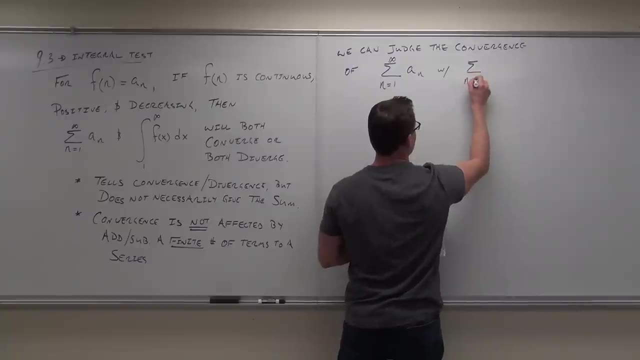 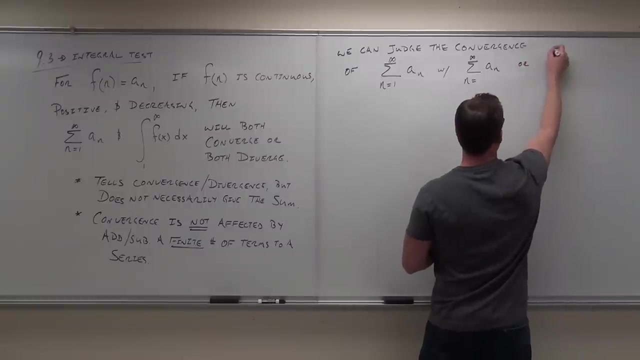 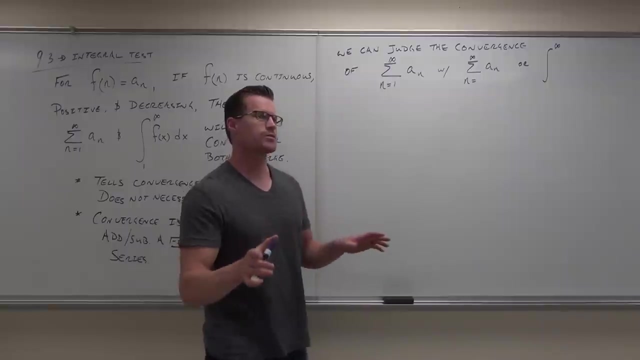 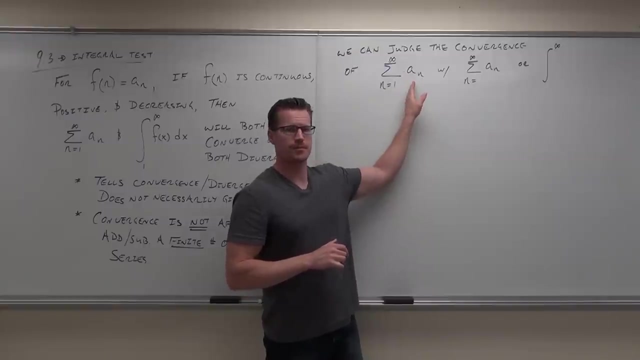 of this series between with this series. Here's what I'm talking about, so hopefully you understand this. Let's say that the first few terms of this series- are you listening? The first few terms of this series don't really mesh up real well with our integral. 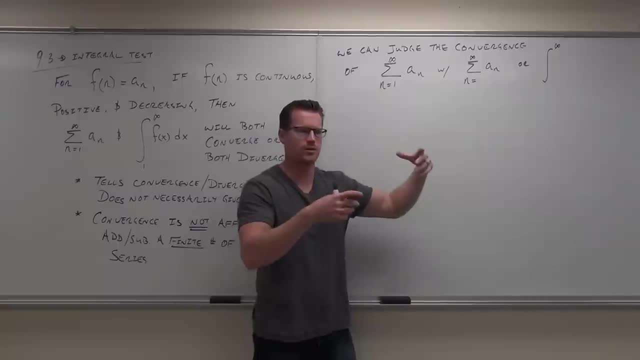 We've got a problem there or something I don't know, just because of continuity or positive or decreasing whatever. Specifically, the decreasing part is what we go with Typically. the continuity is not a problem with our interval. Typically, if it was, our series wouldn't happen. 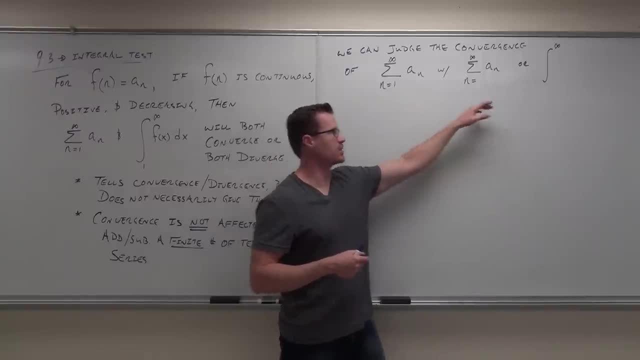 because if we had that issue, if we had a discontinuity here, we'd probably have a discontinuity somewhere in our series. Those terms don't even make sense, But usually for us it's going to be decreasing, And sometimes this decreasing idea doesn't work so well with these exact terms. 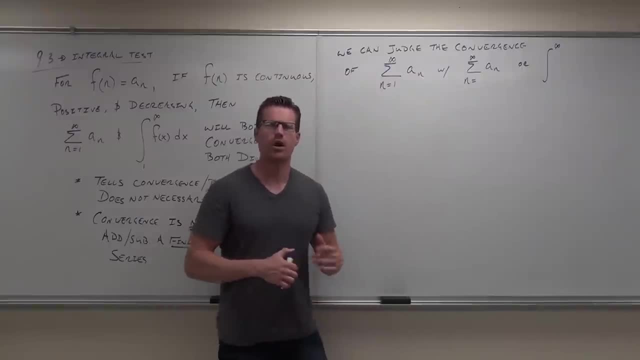 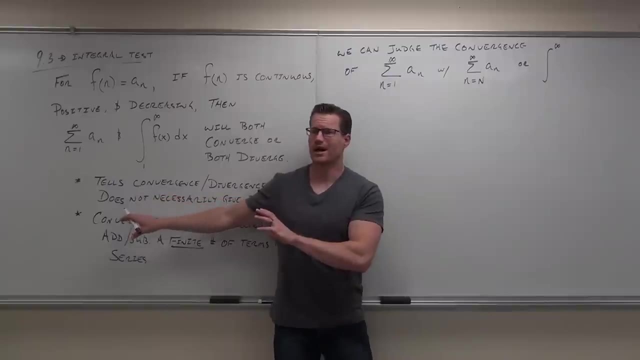 So we say, well, let's forget the first few, Maybe we don't start at 1.. Maybe we start at n. Here's what this is saying, folks. It says: I don't care how many terms you subtract, You can't subtract all of them, okay. 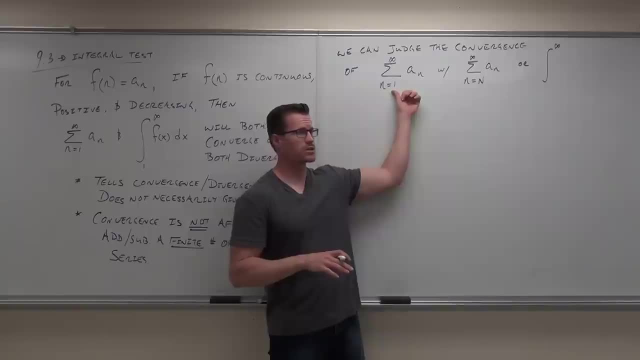 But if you subtract a finite number of terms, say, I don't want to start at the first term, I want to start at the third term. I don't want to start at the first term, I want to start at the seventh term. 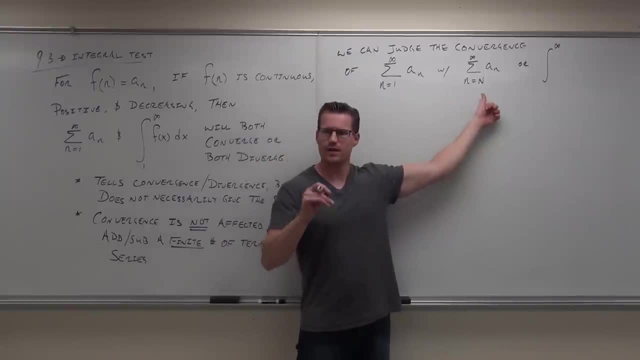 I want to start at the first term. I want to start at the whatever. I want to start at the seventh term, big M. What that says is that, yes, the sum will be different. The sum will be different, We don't care about that. 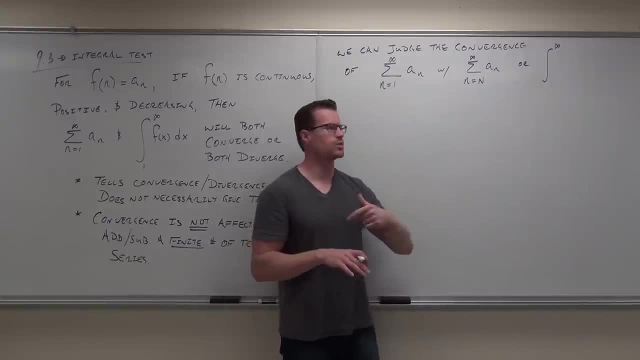 It's not going to give us a sum anyway, But the convergence or divergence will not be different. Does that make sense to you? This is the idea: Sum will be different, S-U-M sum will be different, But the convergence will not. 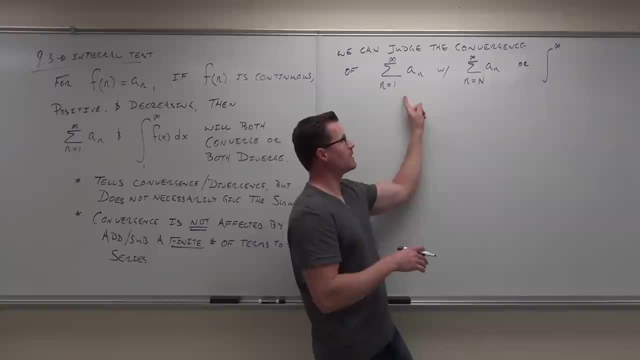 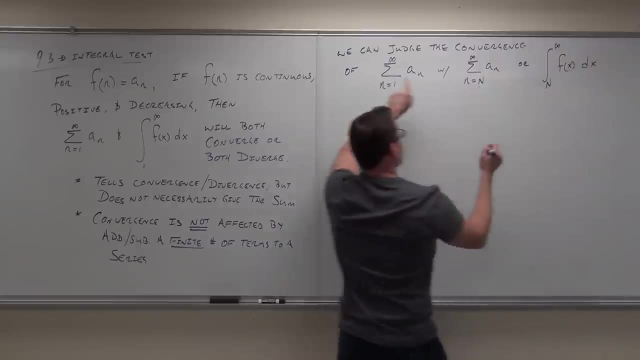 So if our integral is affected by this, we go. man, those terms aren't so great. Let's make it start at a certain place. Therefore, we can start our integral at a certain place and tell us something about our original series. 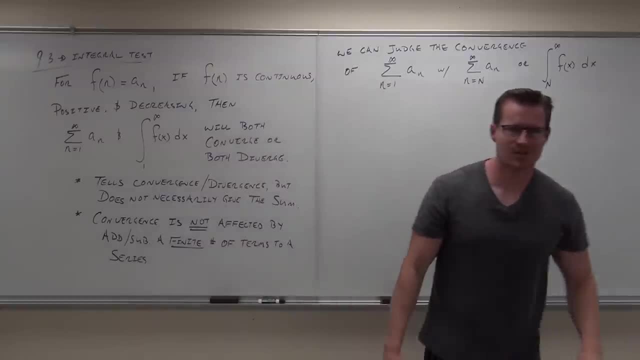 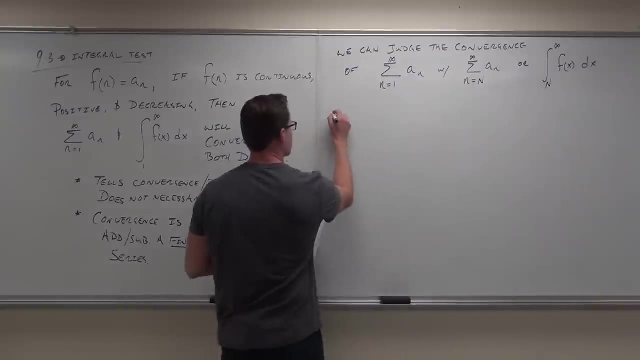 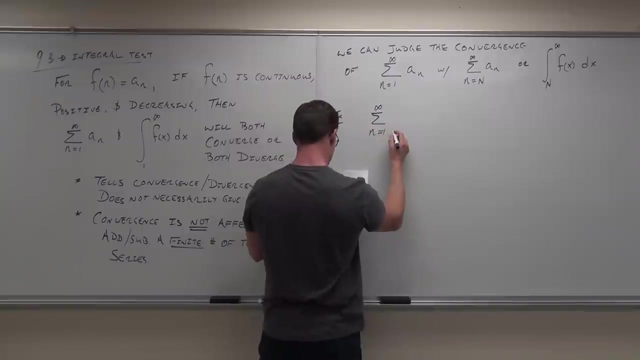 This is the plan. You guys want to see the plan in action. You want some examples. Does this make sense to you? the theory behind it? It's kind of interesting. right, Let's do a couple of real fast ones, just to get our feet wet. 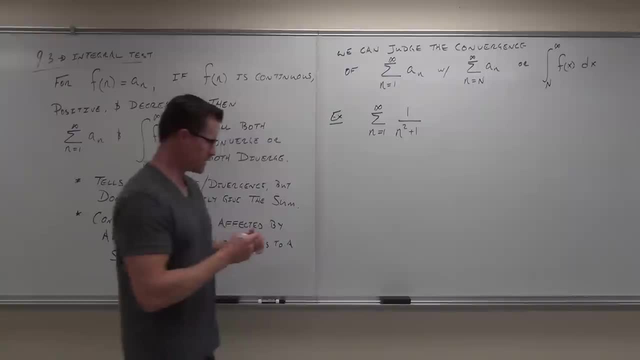 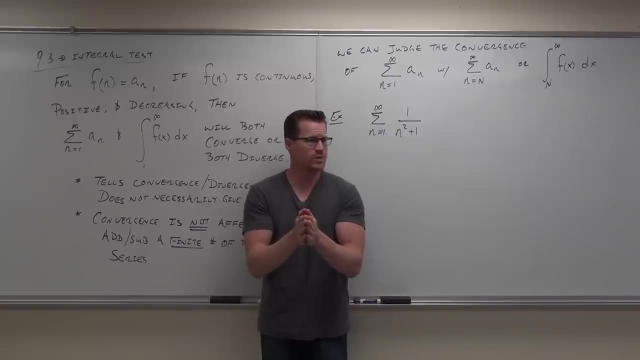 Okay, one more recommendation. I know I've said this before, but I'm going to say it Again and again: please do not forget about the divergence test. Now, none of these, for us, are going to be divergent by the divergence test. 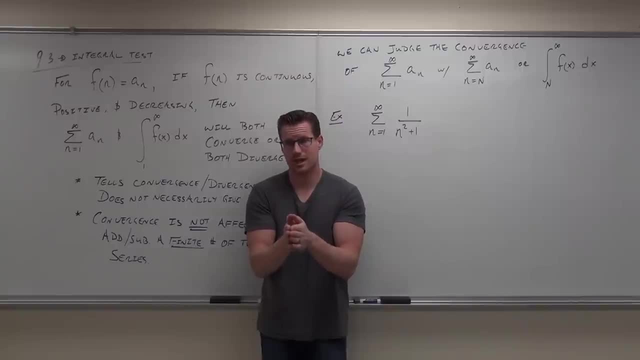 because that's too easy for us at this point. but don't forget about that, Because on a test or a quiz or your homework or something, you look at that and you go: okay, the first thing I'm doing, first thing, right off the bat, I'm taking the limit of this. 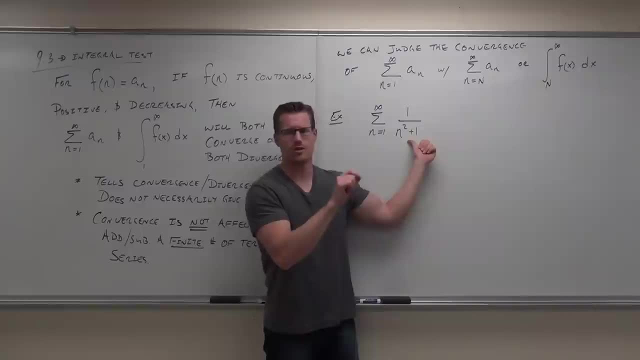 If the limit of this as n approaches infinity, does not equal 0,. what do I know about this series? It's divergent. Don't even have to worry about it. There's not going to be a sum. You don't have to worry about the integral, because it's divergent already. 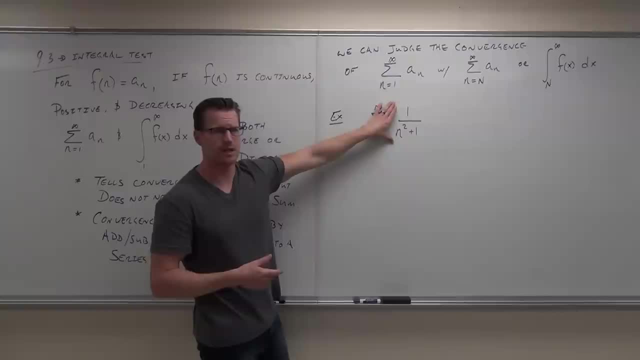 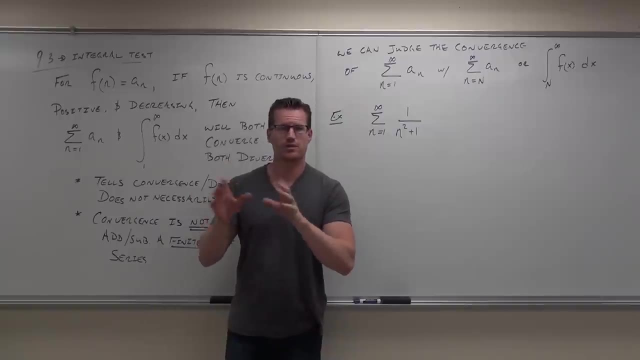 Here. so we take the limit. Is the limit of 1 over n, squared plus 1, equal to 0?? Yes, So it says we're not sure whether it's convergent or divergent, but it fails the divergence test. It's not divergent by the divergence test. 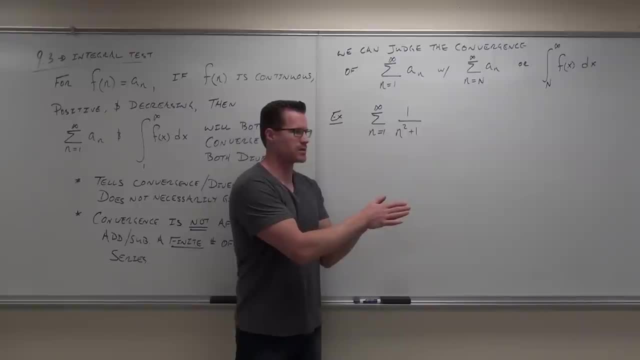 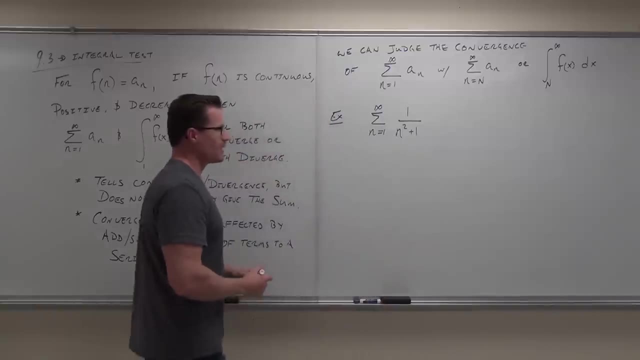 It might be divergent some other way, but not by that. Does that make sense? Do we know it's convergent? No, we don't know that. It's basically inconclusive. So here's what we do. The first thing is: okay, well, it's not telescoping. 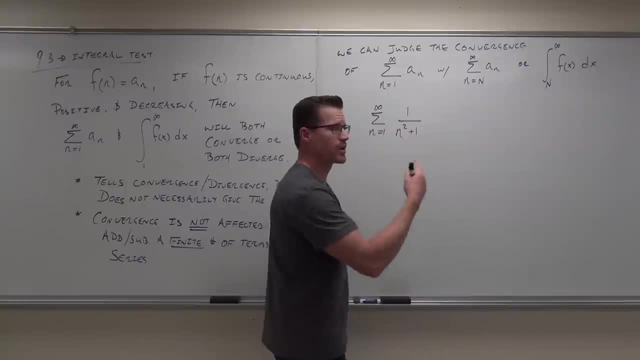 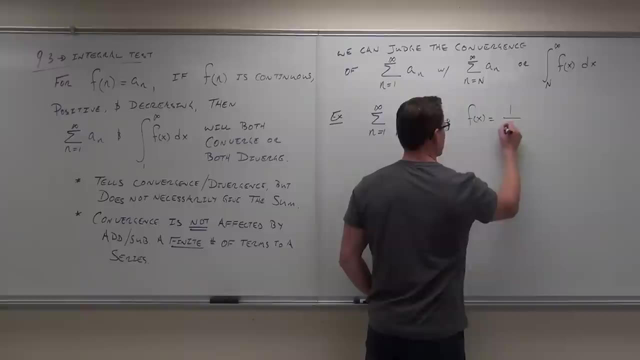 You can't factor it. so it's definitely not that You can't break that up. Then we try the integral test, because you know what I see? I see, let's look at: f of x equals 1 over x squared plus 1.. 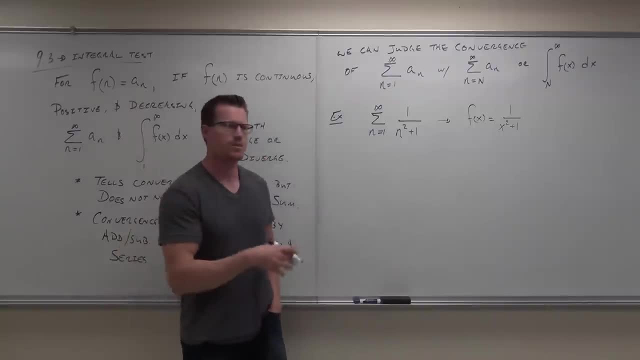 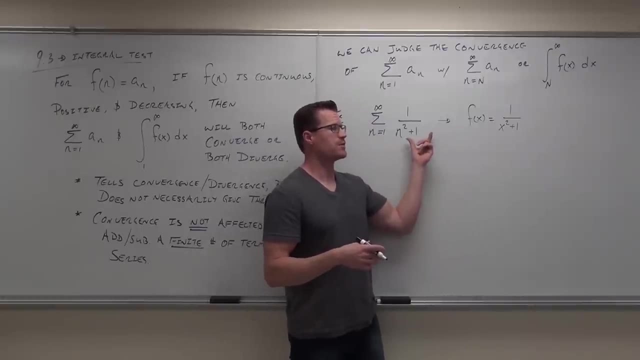 I'm not using n. I know I did up here, but I'm not using n. I'm using the function in terms of x, because what we're doing is we're modeling this function after this sequence. Okay, Basically every term of this sequence is in here somewhere. 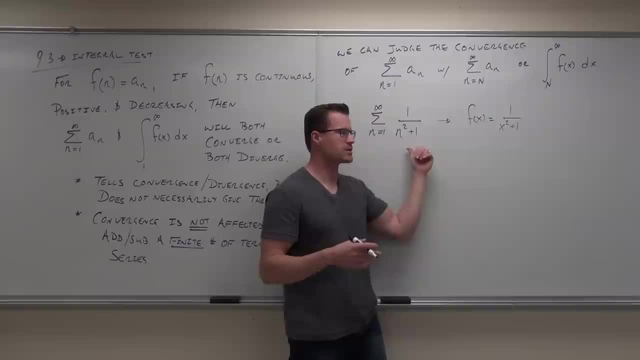 A lot more terms besides. these terms are in here. yes, but at least this contains all of these terms. Does that make sense to you? Yeah, So we're going to say: if this contains all these terms, this will act as an upper bound for this sequence, provided it is positive. 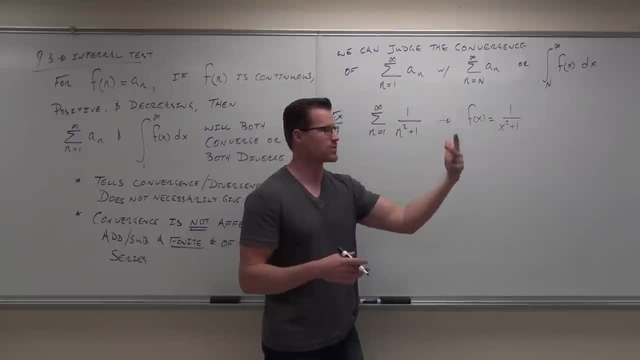 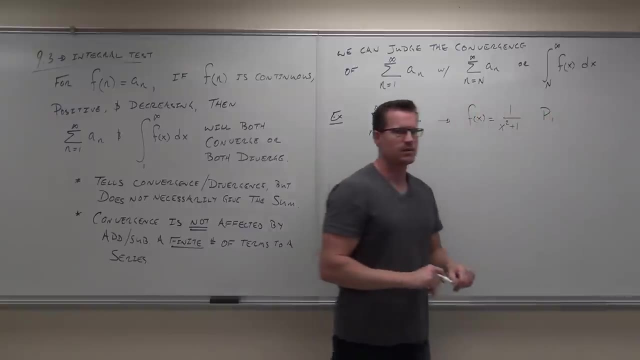 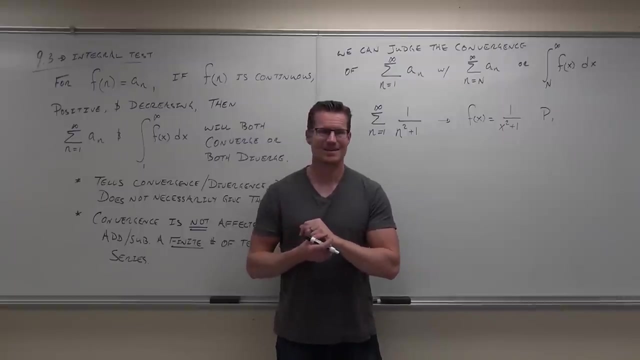 provided it is continuous, provided it is decreasing. So let's think about this: Is this always positive? Yes, Absolutely. It's x squared plus 1.. Is it continuous? Yes, Since it's always positive. well, yeah, it's actually always continuous. 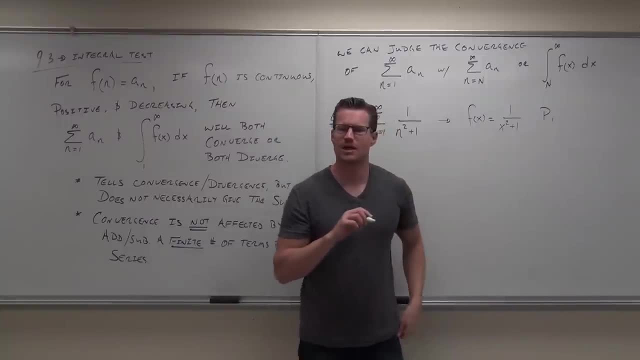 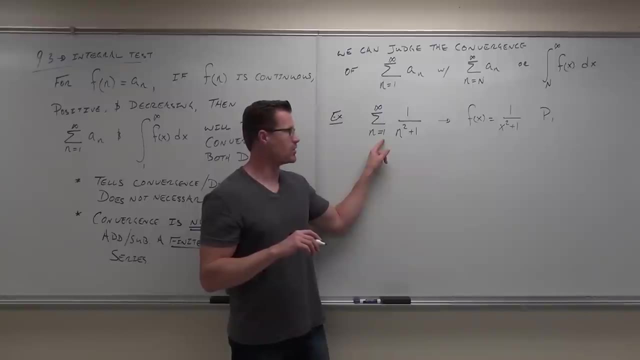 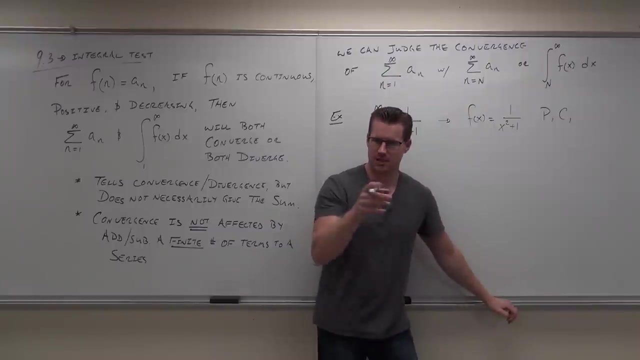 Oh, but wait one thing. Do we have to be continuous everywhere? We actually only have to be continuous on that interval right there. So it's continuous. Yeah, Is it decreasing? Yes, It keeps getting smaller. It does keep getting smaller, because this is a constant, isn't it? 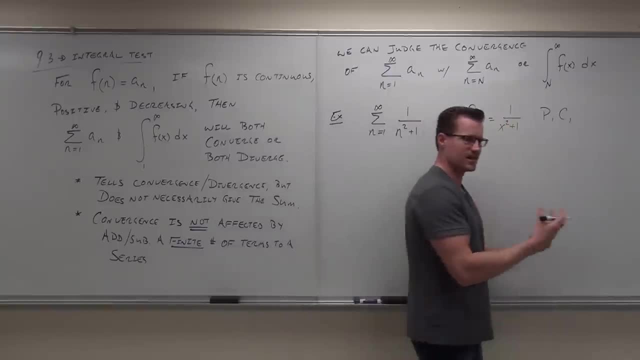 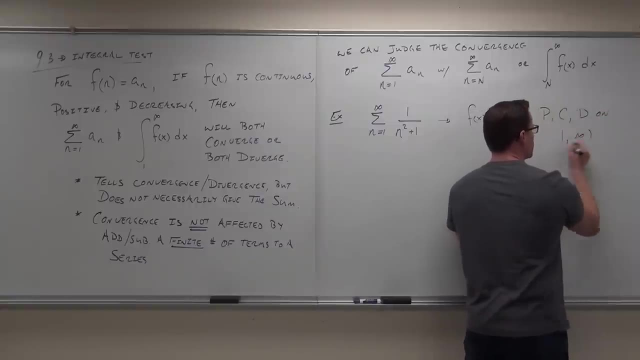 Yes, So a constant by something that's going 1,, 2,, 3,, 4,, 5 is decreasing, obviously decreasing. Now we're going to state this on the interval 1 to infinity, because we don't care about anything else. 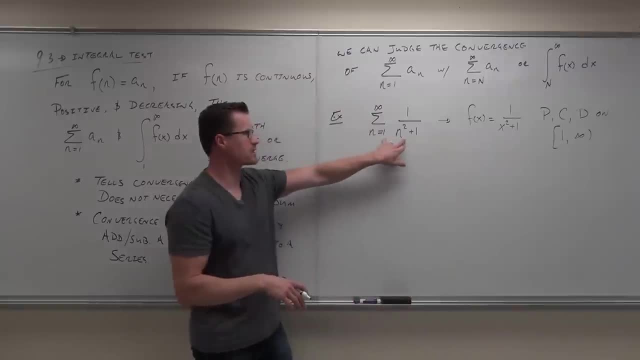 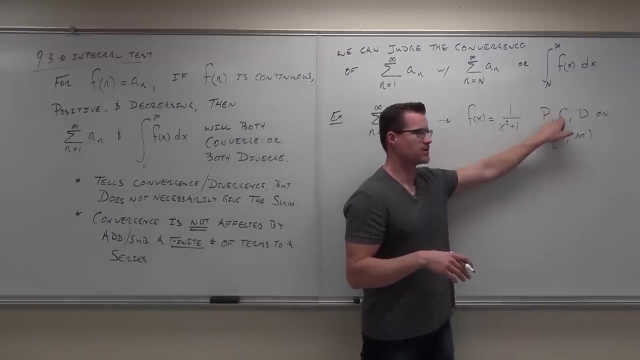 We don't care about anything else, because what we're trying to do is model this function on this series. This series starts at: hey, where does this series start? at 1, 4, 5.. So as long as this function is positive, continuous and decreasing on 1 to infinity, we are good to go. 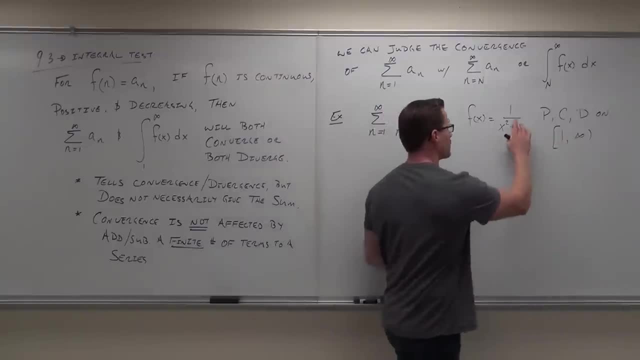 Show if you can understand that concept. So even if this had been like: oh, now this is going to change something a little bit, minus 1.. I'll show you something here real quick. Is this positive? Not all the time, yeah. 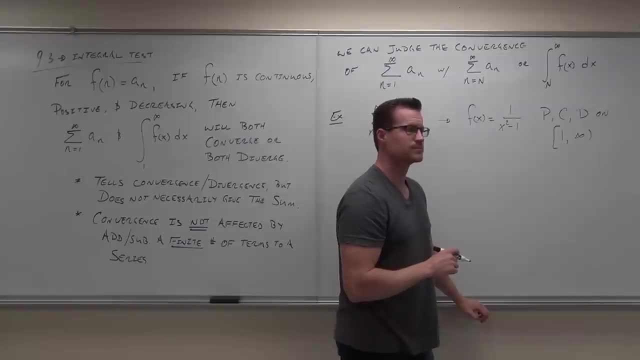 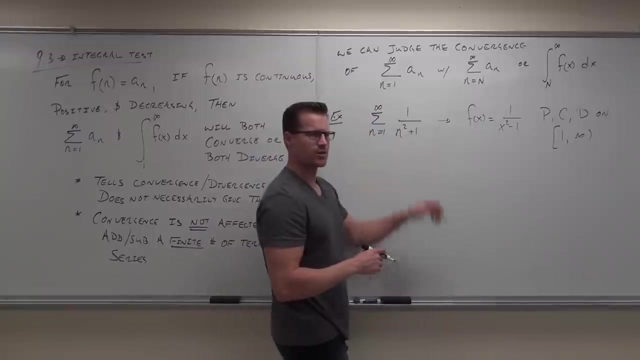 Is it positive on 1 to infinity? No, not on infinity, Because you plug it into 1.1? It's positive. Is it continuous? No, not at 1.. So what you do is you go. hey, can I subtract a finite number of terms? 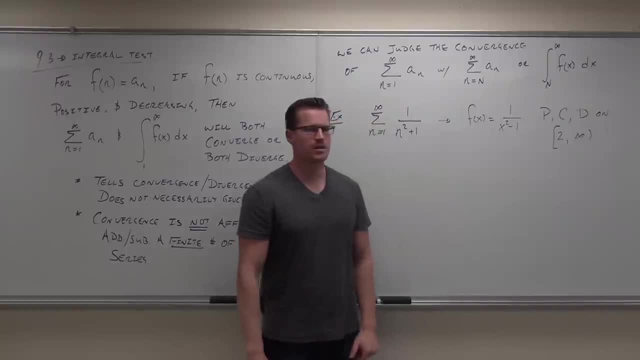 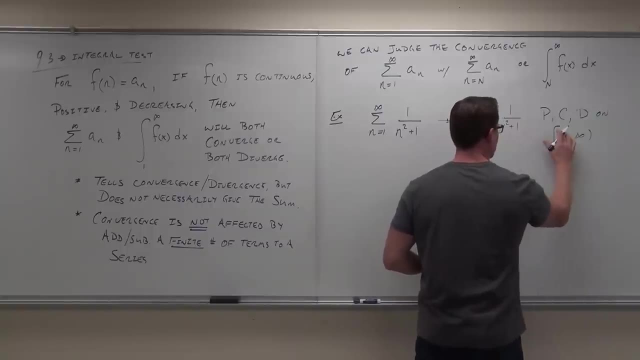 Heck, yeah, Let's start at 2.. There you go. Is it positive, continuous and decreasing Done? OK, So we can do things like this. Now, we're not there yet. We're going to get there in the next couple examples. 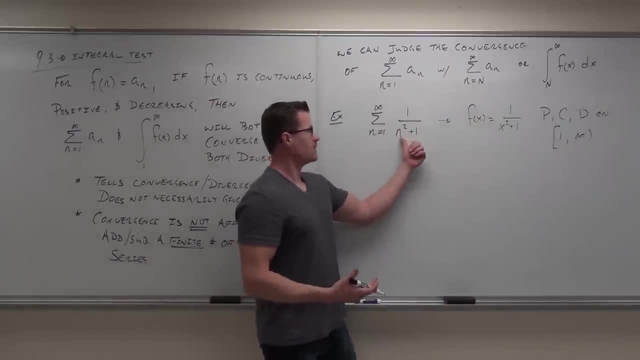 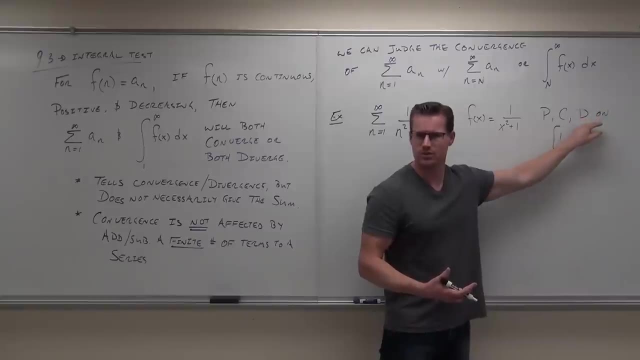 So the next idea is: shoot. if you know how to model this series on a function and you know it's positive, continuous and decreasing, do you need to check for this every time? You certainly do. You have to show each one of them. 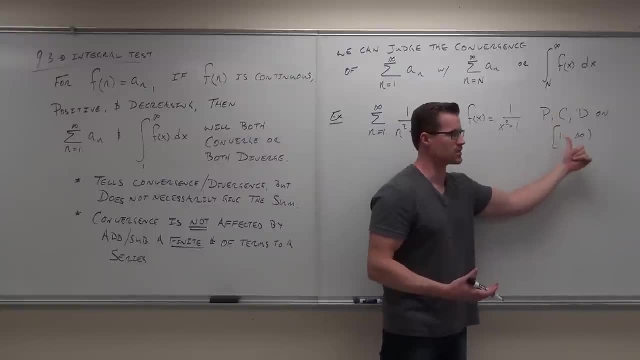 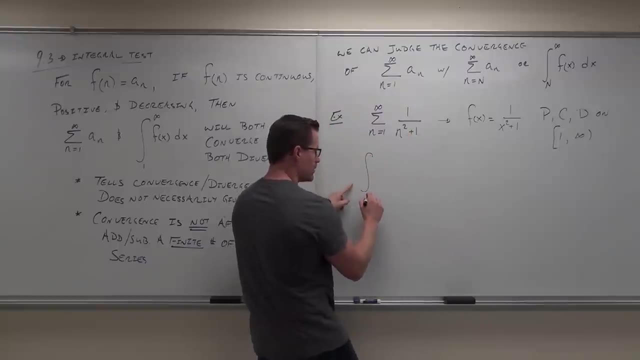 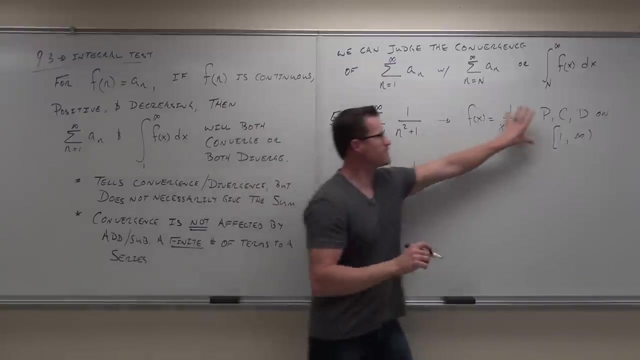 Some are obvious. This is obviously positive, obviously continuous and obviously decreasing. OK, Then, what we say is: then this series and this integral, from where to where, 1 to infinity Of 1 over x squared plus 1 dx, these two things because of this statement. 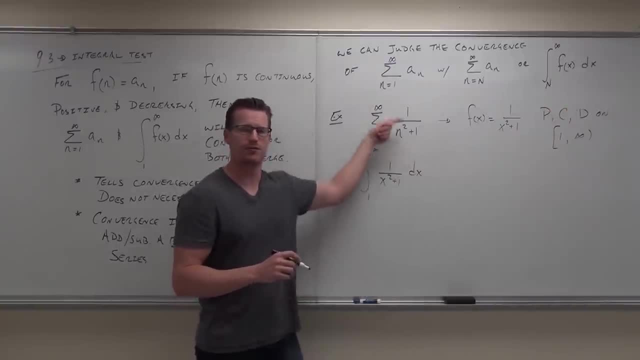 these two things will either both converge or they will both diverge. That's what this says. If this diverges, this diverges. If this converges, this converges. Do I know the sum? No, OK, But it converges. 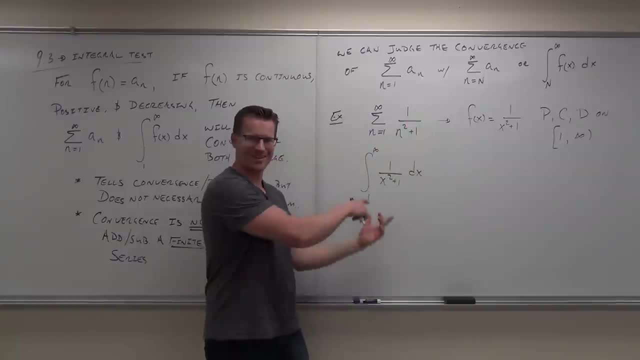 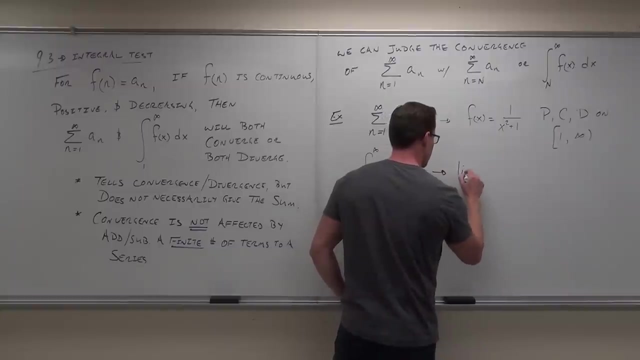 Don't know what to, but it converges, Do you see it? That's why we did the last chapter. What is that? Oh, no, no, no, no, no, It's an improper integral. It's an improper integral which you must show me appropriately. 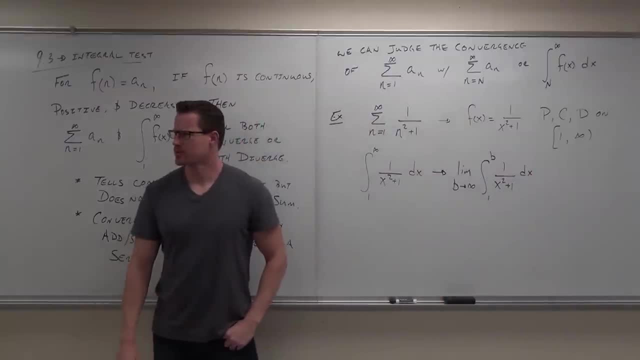 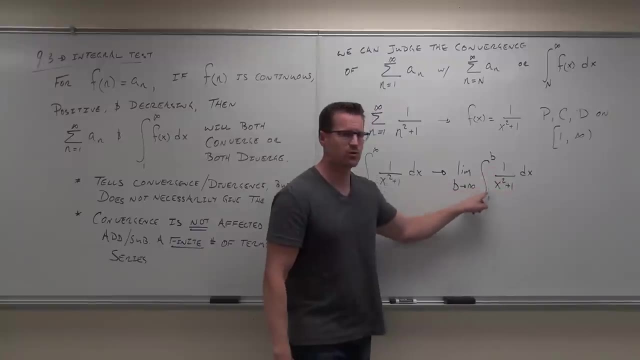 How do you solve it? Do you remember anything about improper integrals? That's an infinite interval: 1 to infinity. We say, hey, b goes to infinity, take a limit of that, No problem. Do we know how to do the integral of 1 over x squared? 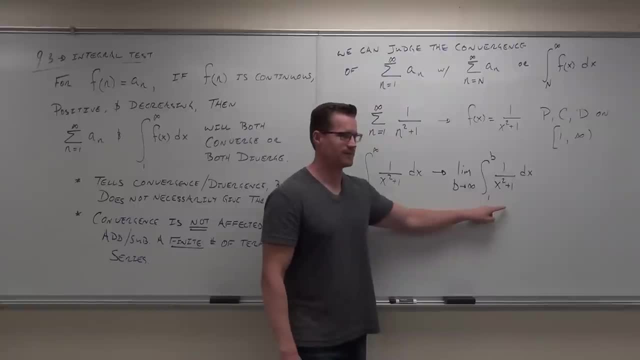 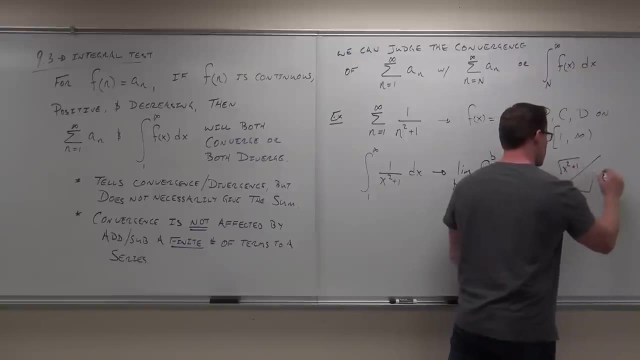 How much is the integral of 1 over x squared plus 1?? It's tan inverse. If you didn't know that, you could do your triangle x squared plus 1.. You could do your x over 1.. Hey, tangent. 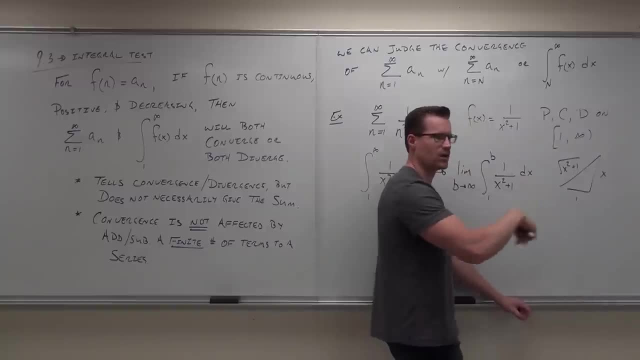 Look at that Tangent. You'd have a secant squared in there somewhere. It's simplified: 1, that integral of 1 would be theta. Theta would be tan inverse of x. You can look that up for our. I've done that example several times, so look that up in the video or in your notes. 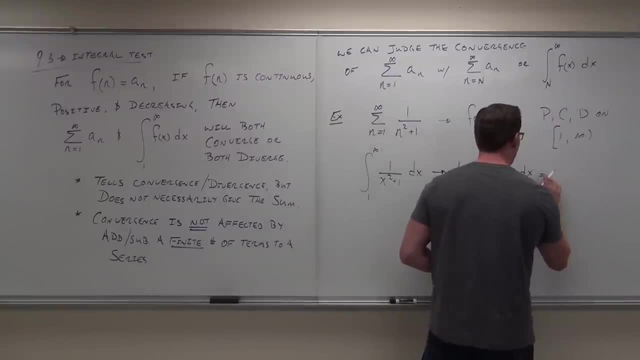 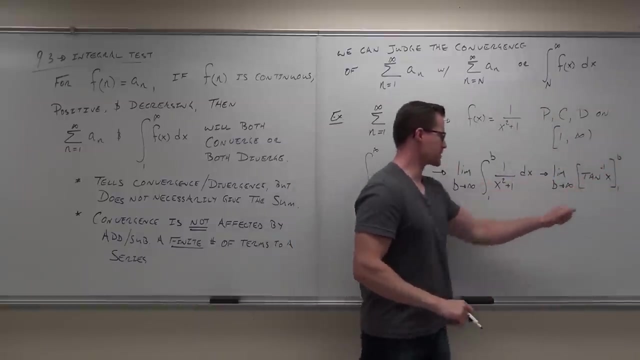 This right here is the limit as b approaches infinity, of tan inverse x from 1 to b. Integral of this is tan inverse x. It's going from 1 to b. No problem, We have a limit still. Yeah, of course we have a limit still. 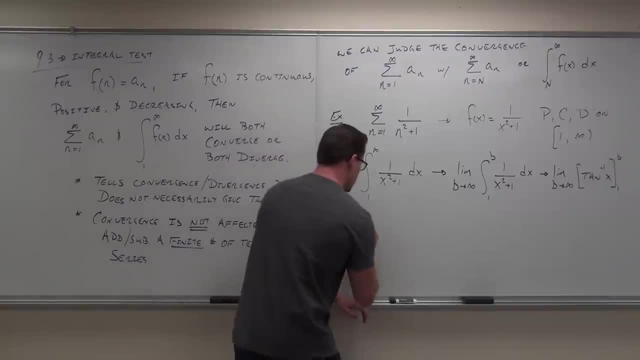 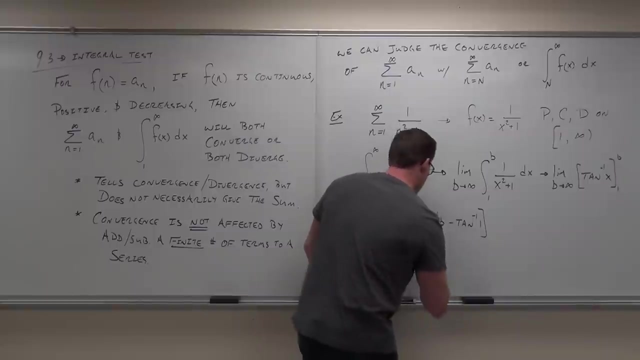 What's the next step? What are we going to do? Evaluate it, Plug it in. Plug it in. Sure, we've got tan inverse of b minus tan inverse of 1.. Now you better be able to tell me what tan inverse of b and what tan inverse of 1 are. 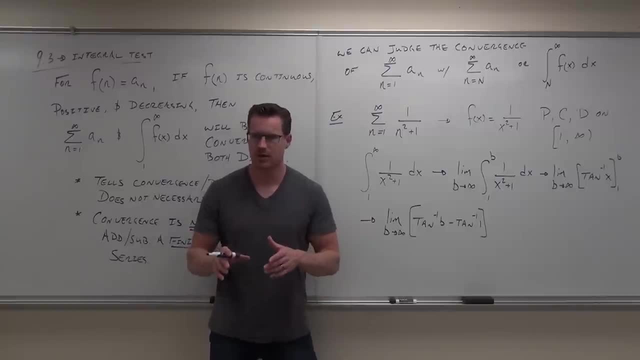 You might want to have your unit circle out or have something out there. It lets you see this pretty easy. For me it's no big deal because of course you know. I know this in my head. If you don't know it in your head, have a little cheat sheet when you're doing some of these problems, especially with our tangents. 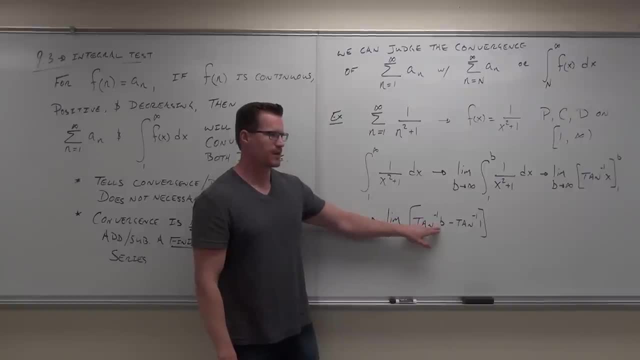 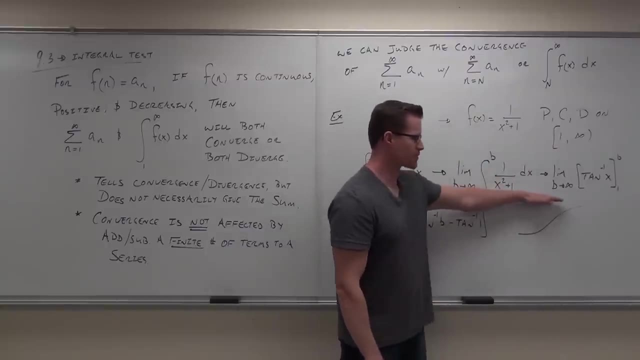 So let's think about tan inverse of b. as b goes to infinity, Tan inverse looks like this, Tan inverse looks like that, where you have a horizontal asymptote here at pi over 2 and a horizontal asymptote here at negative pi over 2.. 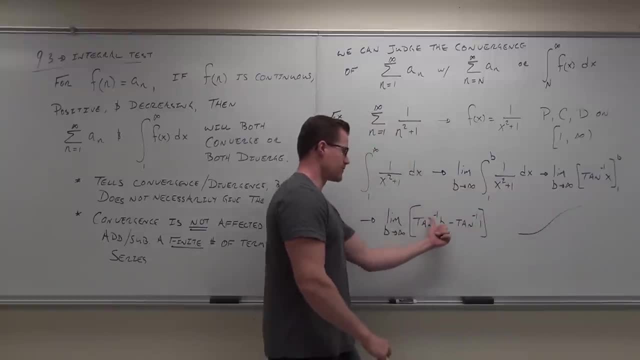 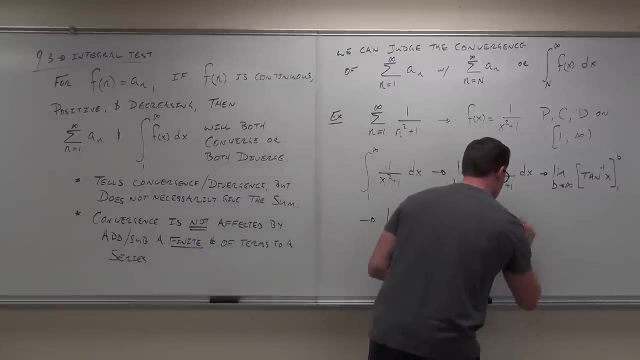 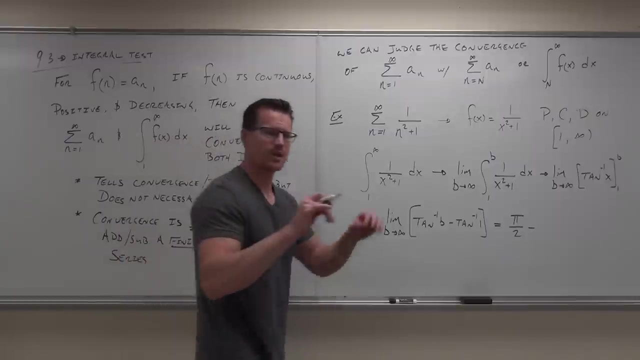 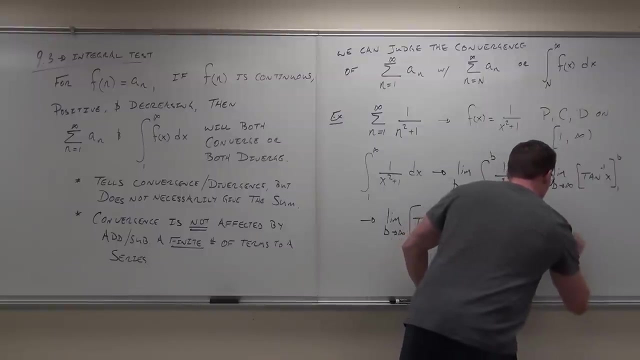 So this is pi over 2.. As tan inverse approaches, sorry, as b approaches infinity, tan inverse of b approaches pi over 2, minus tan inverse of 1. That's pi over 4.. Because tangent of pi over 4 equals 1, tan inverse of 1 equals pi over 4.. 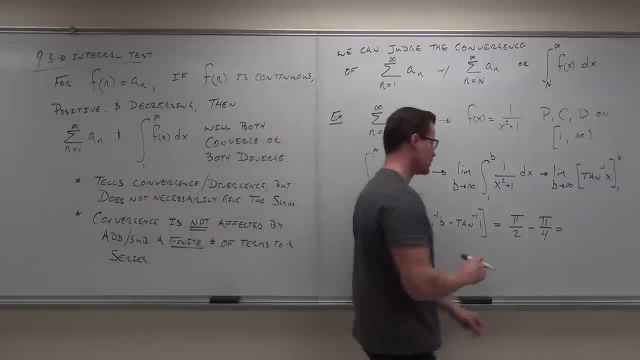 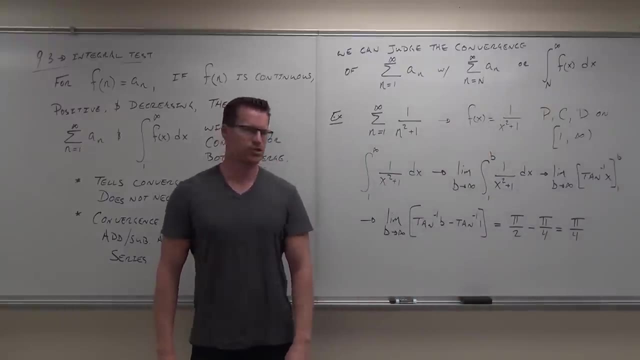 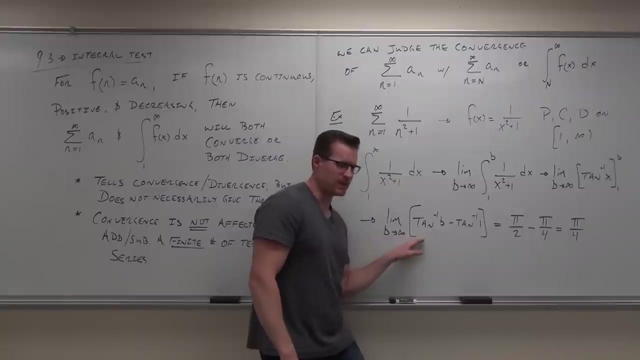 Equals pi over 4.. Now Question: Did we get a number? Yes, This limit, This limit. This is why the limits are important. This limit tells you that the limit exists. right, This says the limit exists. Therefore, this improper integral was convergent. 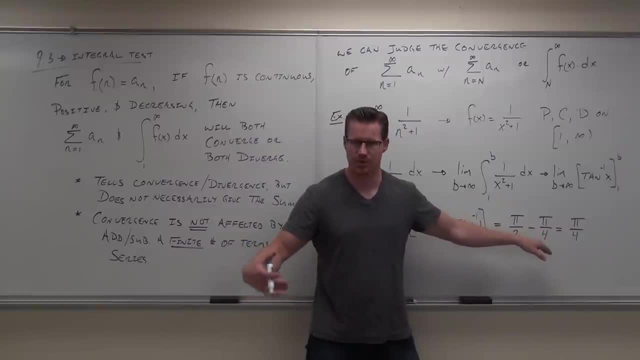 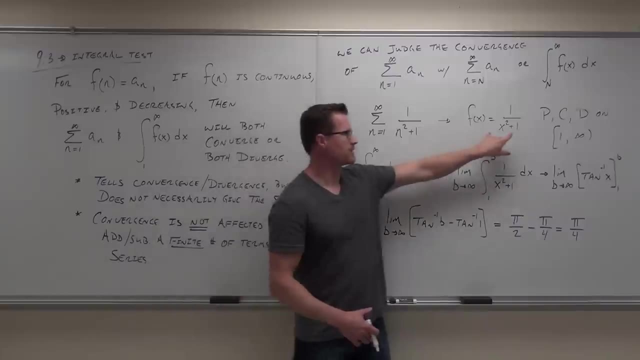 That's where we had the convergent, the first word right. The first time we had that was in improper integrals, Because the limit exists. the integral is convergent Because the integral was convergent based on this function, which was positive, continuous and decreasing. 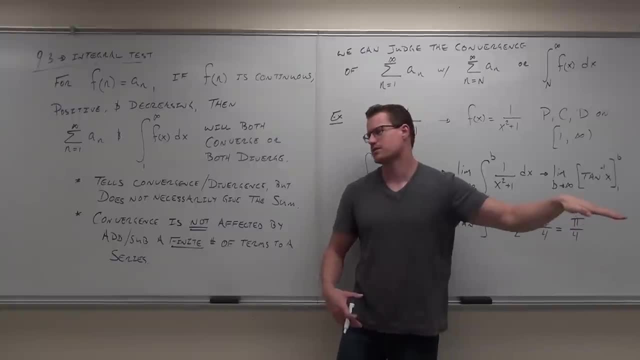 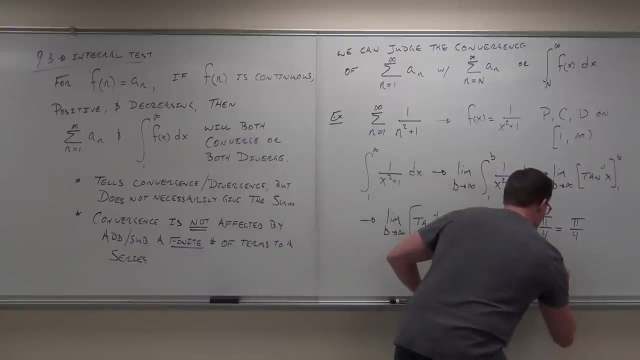 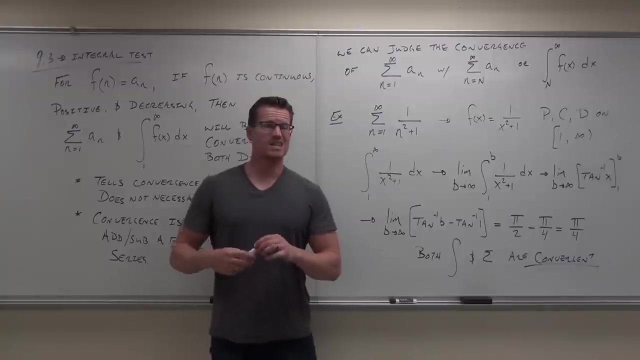 Which acted as an upper bound for our series. If this thing is convergent, tell me something about our series. Convergent, Good, So both the integral and the series are convergent. Do I know what the sum of my series is? 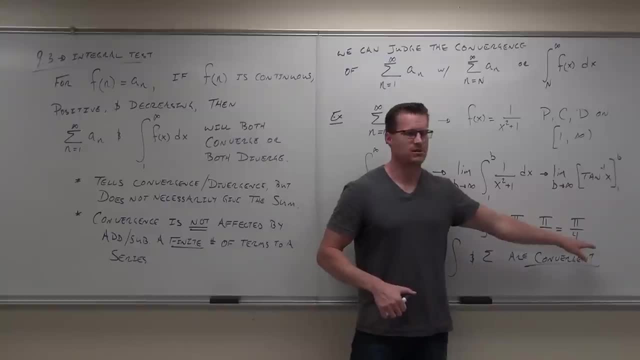 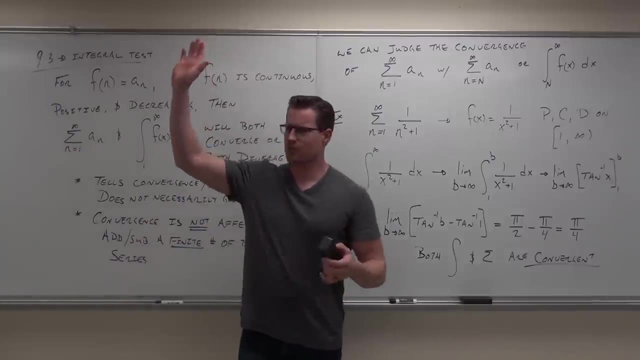 No, Is this the sum of my series? No, I'm sure I don't know, But we know that that series converges. Show of hands. if you understand the idea of this Kind of a cool idea, right, Let's practice. a couple more examples. 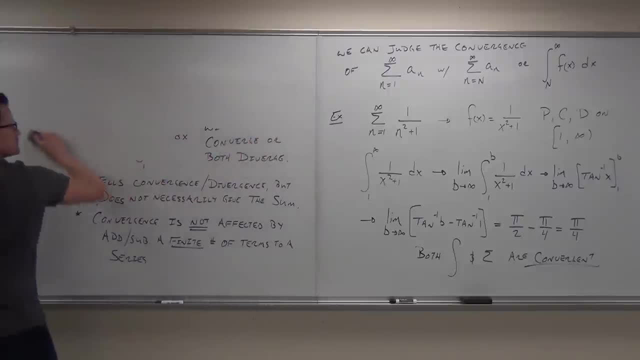 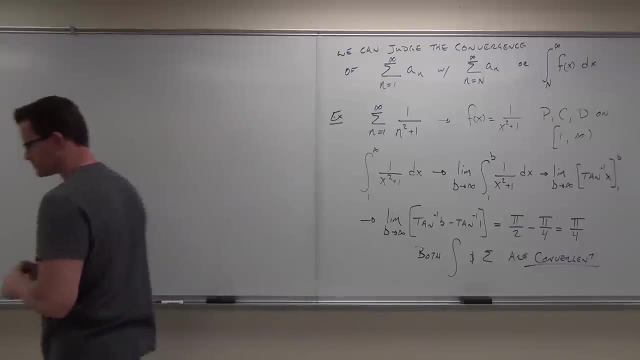 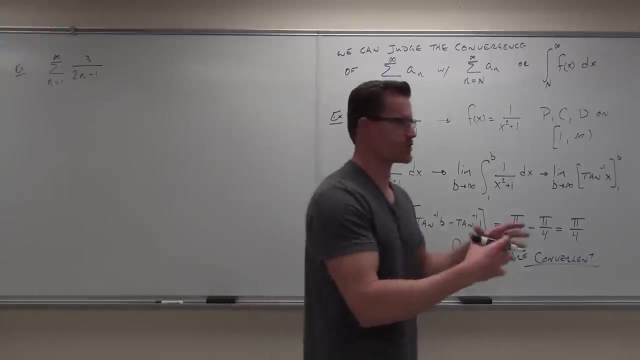 Get right into it. I'll try to do as many as possible in our time allowed here for you. Okay, so I'm still going to walk you through this, because I know you guys are fresh at this. We only have one example, So the first thing we do, 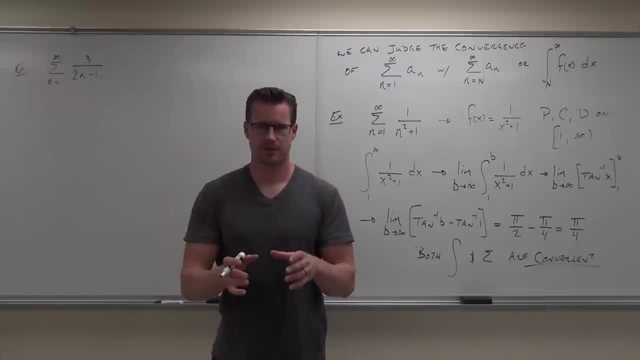 First thing is: my goodness, take a limit. Take a limit. If the limit does not equal zero, the series diverges. Now, most of these I'm giving you here, they're not going to. that's not going to happen. 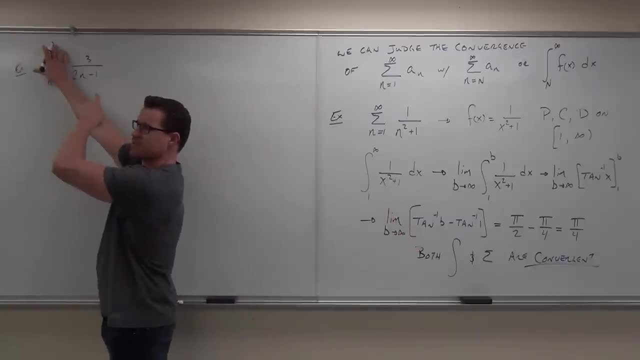 But I want you to get in the habit of that. Is the limit of this thing zero as it approaches infinity? Yes, Yes, it is Constant over infinity is infinity. So the limit is zero. Does that make sense? That means we've got to keep going with something. 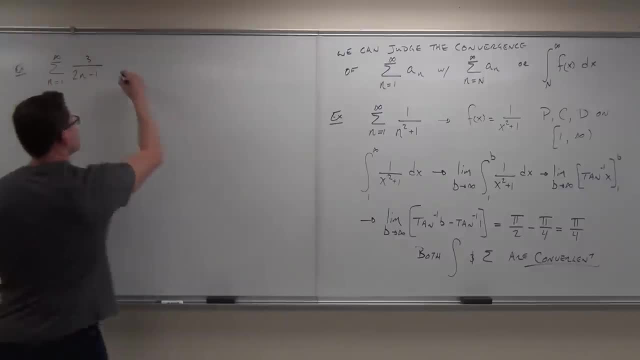 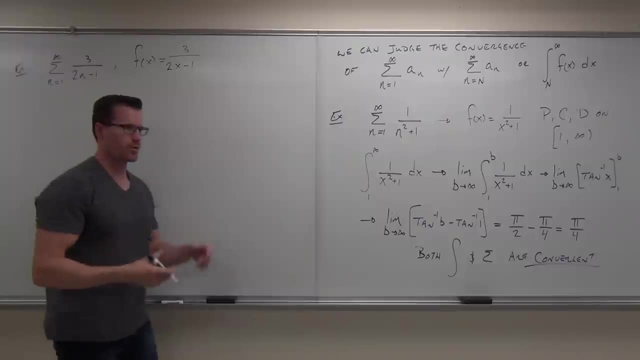 The something here is going to be our integral test, So we're going to base our function on our series in terms of x, of course. Then we're going to check for three things. What are the three things we must check for for the integral test to work? 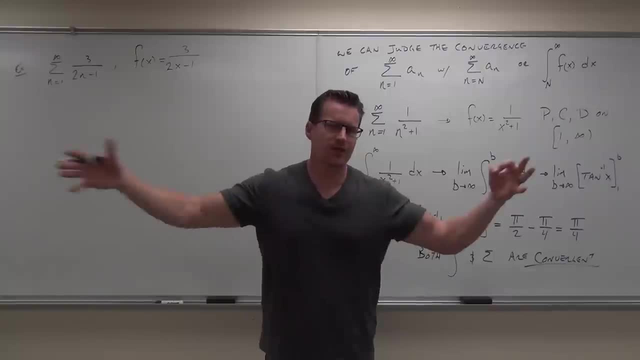 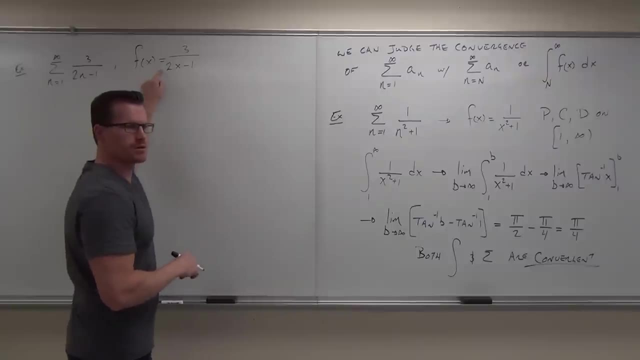 Positive, continuous and increasing For everything, or just a certain interval, A certain interval? Aha, Is this positive? Yes, Yes, Not always, Not always, But I don't care about that. Is it positive? on where am I starting? 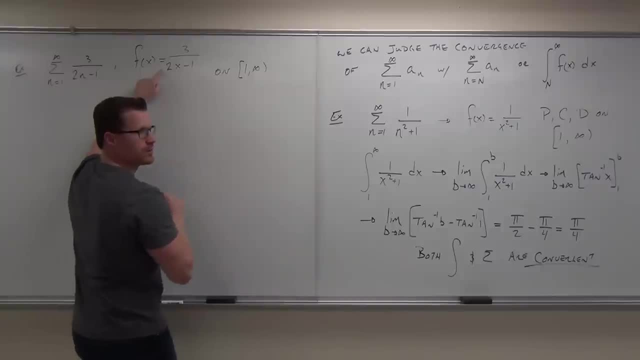 One half. Is it positive on this interval? Yes, Yes, Is it continuous on this interval? Yes, Notice that one half would be a discontinuity. Does that make sense? Yes, Is one half in my interval? Yes, Then I do not care. 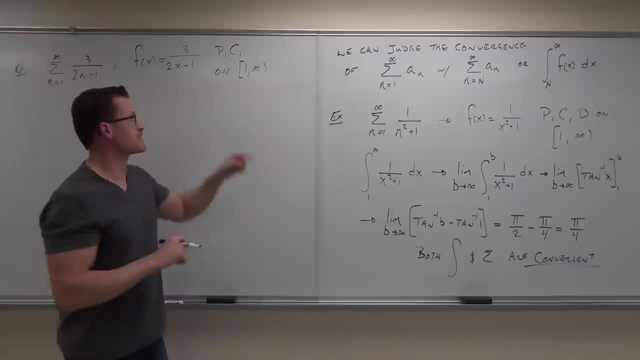 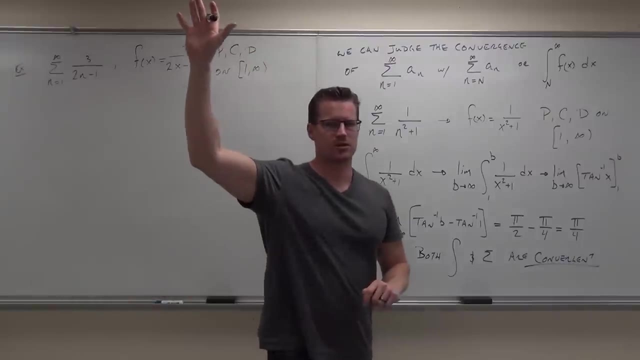 Is it decreasing on my interval? Yes, Yes, That's a constant over a variable that is growing. Yes, That's a constant over a variable that is growing bigger, Decreasing. So if I feel okay with that positive, continuous decreasing. 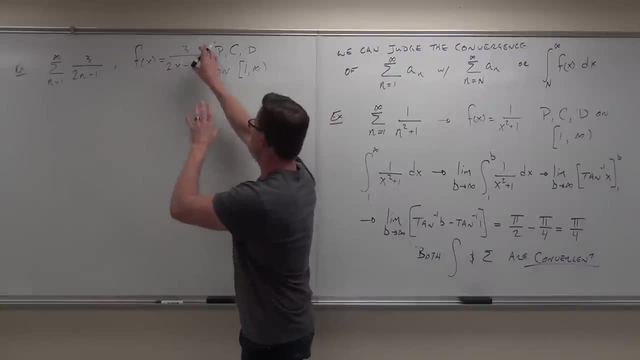 Well then, what we're going to do is say: since this function is positive, continuous and decreasing on my interval- the same interval as my series- I'm going to take an integral of this. The integral will act as an upper bound for my sum, my series. 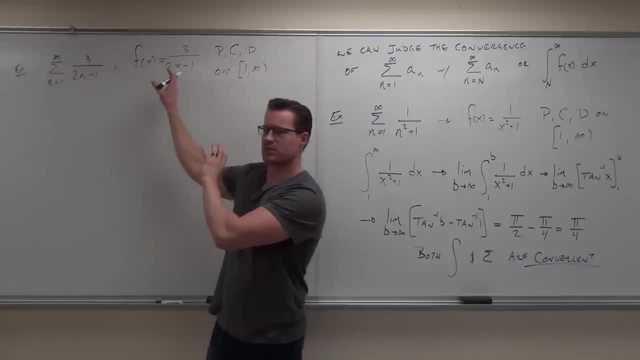 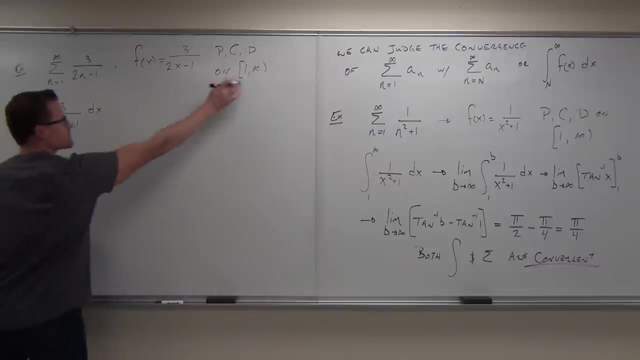 If the integral converges, this thing converges. If the integral diverges, this thing diverges. So Let's take our integral. Where does our integral start? One to infinity, Yes, Same thing as this. One to infinity. 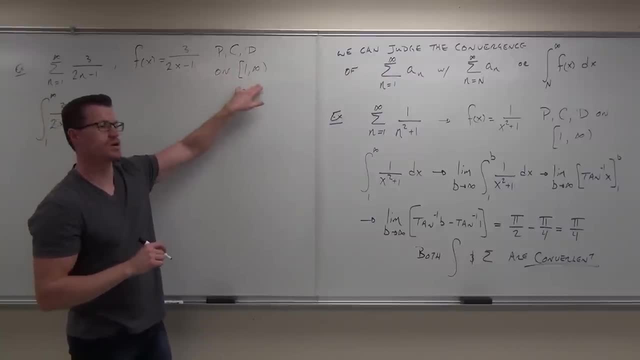 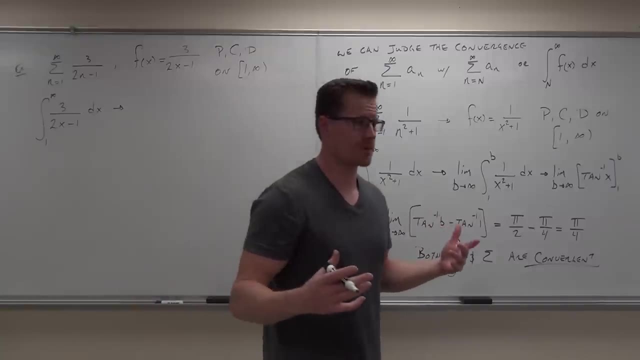 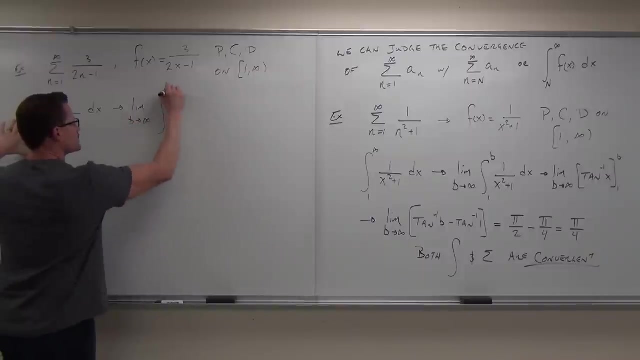 So wherever this function is positive, continuous and decreasing, that's where you integrate. Do you guys see how many times you're going to be using limits here? These are all going to be improper integrals, So we're going to have a limit as b approaches infinity, from one to b of three. 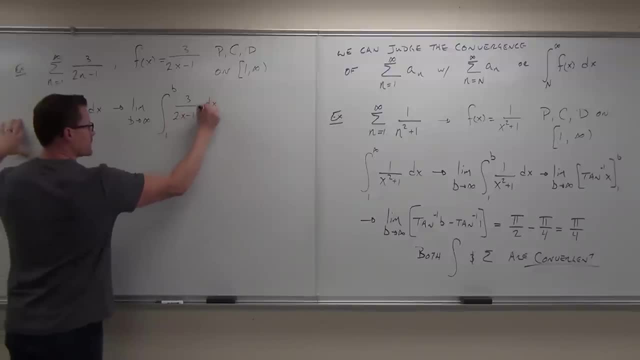 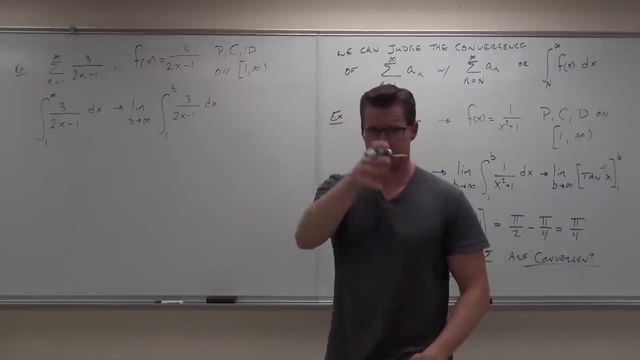 Of three over two x minus one, dx. Oh my gosh, It's an easy one. Tell me what we should do with the integral of three over two x minus one. Pull three out. Substitute: Pull three out. Do a u sub. 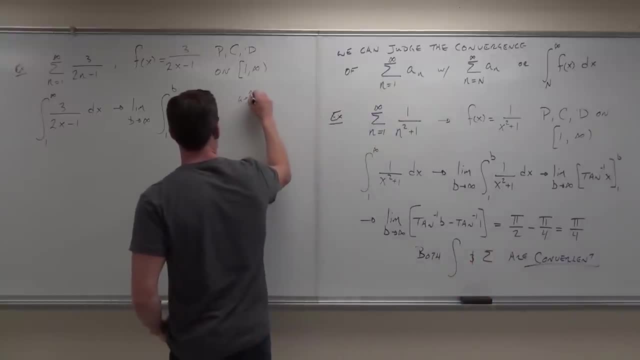 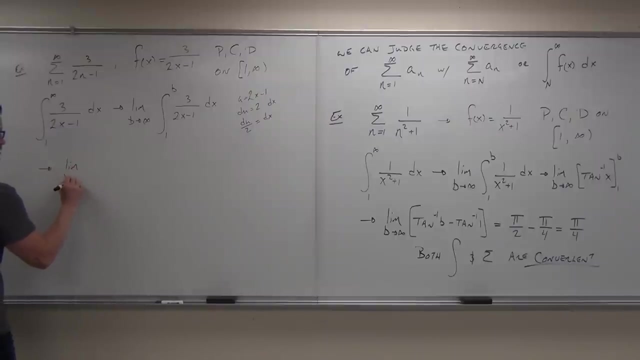 Very easy. If we do a u sub, we're going to get u equals two x minus one Du equals two x dx. Sorry, Two dx Du over two equals dx. So long story made real short. we have a limit as b approaches infinity. 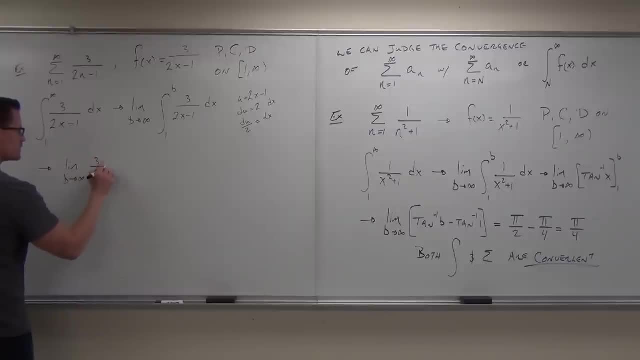 Of three halves integral, one over u du. Well, that's a limit. I'm going fast here. Is that okay with you that I'm doing these integrals really quickly? Yes, Just because. well, frankly, I mean, we should know how to do all those anyway. 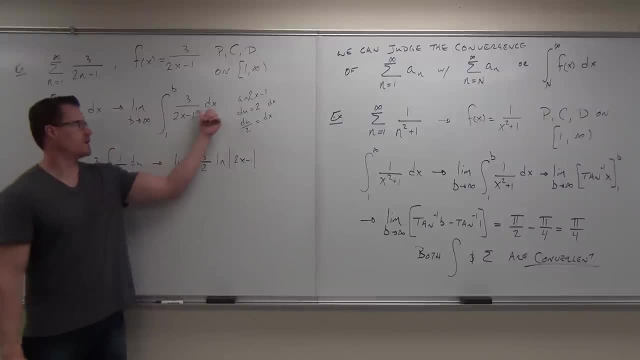 You guys? okay with this one. so far We go. hey, you know what? Two x minus one is our u, So we have three halves. Pull it up front. Integral of one over u: No problem, Du. Integral of one over u is ln absolute value of u. 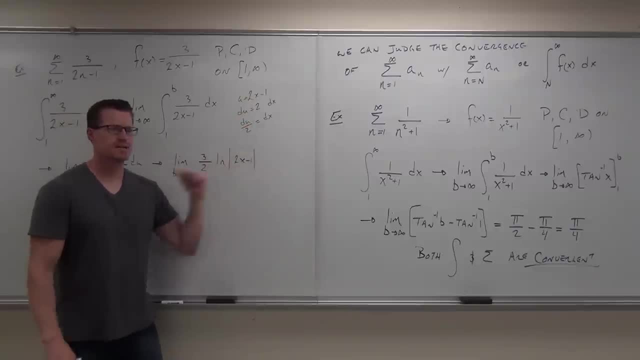 Now tell me something When I plug in my two x minus one. do I need the absolute value here? Yes, Well, from ones that are always positive, Think about my interval. Do I need the absolute value here? No, No. 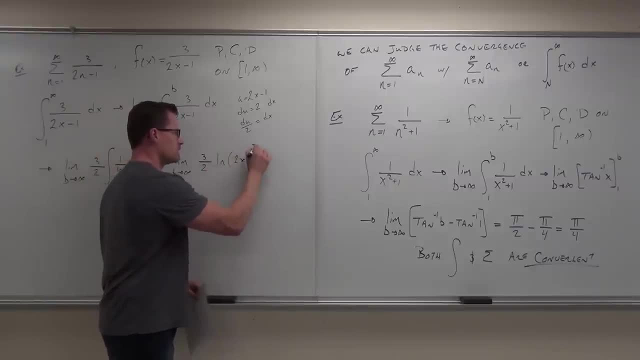 I don't. What I do need to do is evaluate from one to b and then take my limit. So let's do that. This would be a limit, as b approaches infinity, of three halves. You know what you can do. You can even pull the three halves all the way up front if you want to. 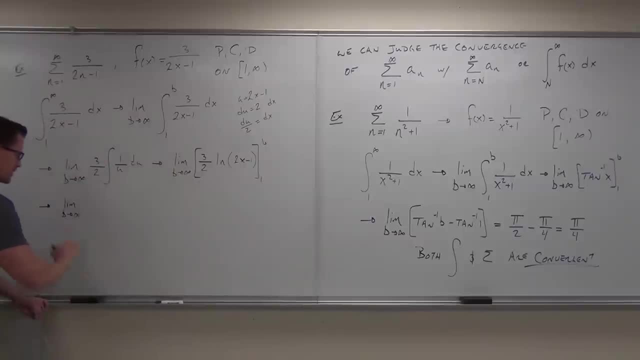 You don't even need it here. The constant can be pulled out in front of the limit. So let's do that. Let's have three halves up front. We'll have ln of two b minus one minus ln of two minus one. I'm going to make sure you guys are OK with this before we go any further. 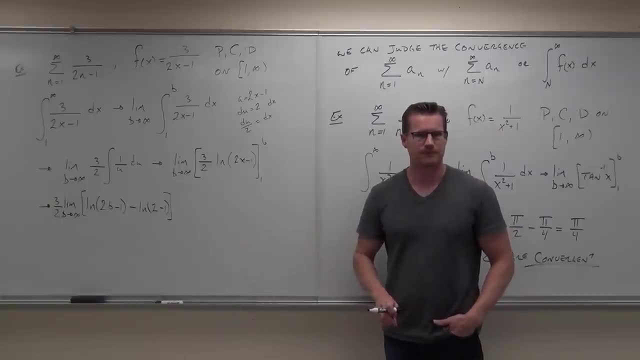 Are you guys OK with this one, Patrick, Because it's always positive. don't we never need the absolute values on it? Don't we never need? I don't know how that ends in English class. You know I'm not going to make an absolute statement there. 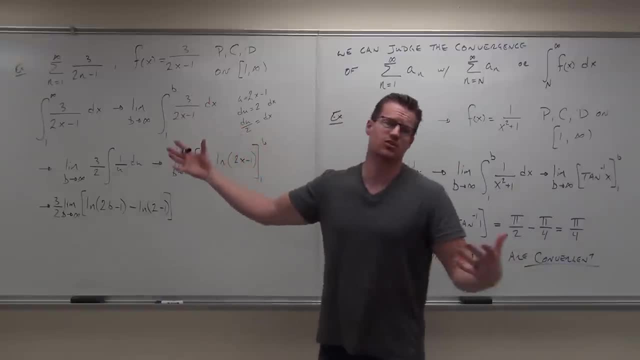 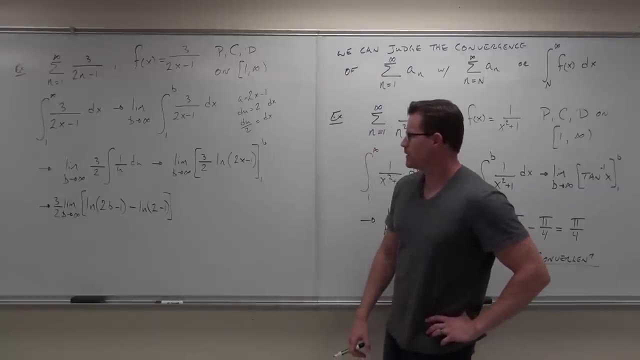 It's going to have to depend on what you have. What if you had x's over x's? I'm not sure. OK, I don't know how that's going to work there. I'm not going to make an answer. I don't know. 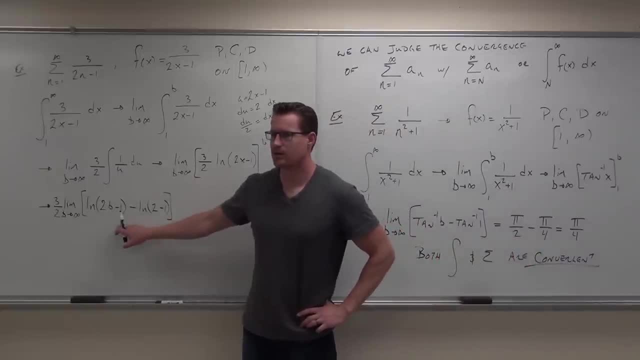 What I want to know is: are you okay making it this far? Yes, This is exactly the same stuff that we've done already in this class. Let's see what pull out- three halves, of course, That's you know. we've been doing that for a while. 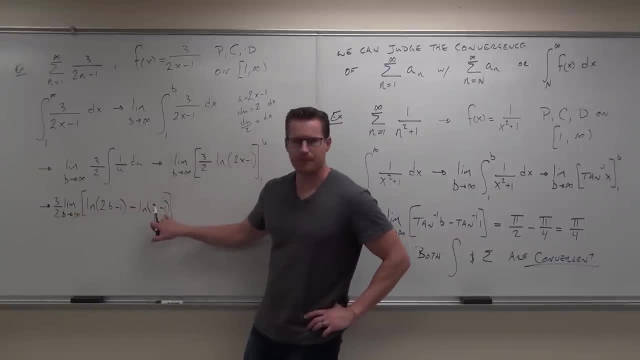 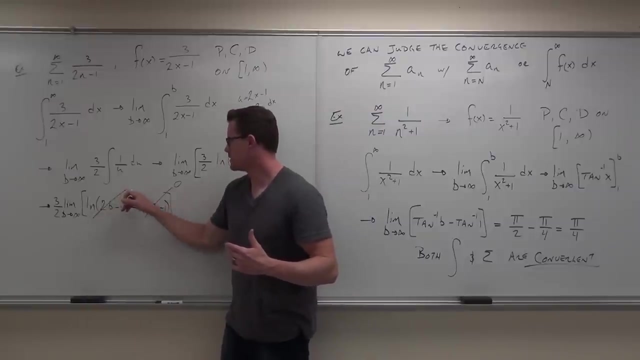 So three halves up front. Tell me what's two minus one. What's ln of one Zero. What's b here? Go to infinity. What's two times infinity? Infinity minus one: What's ln of infinity? Is this integral, convergent or divergent? 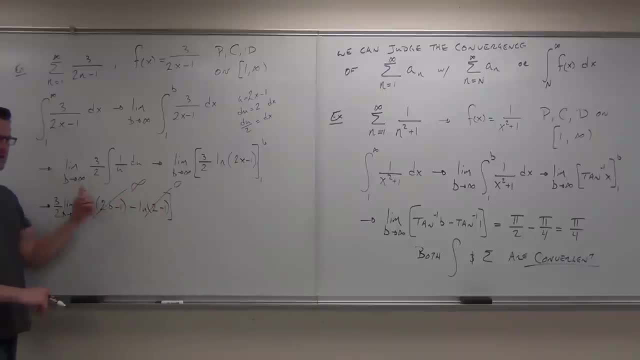 Divergent. This thing is infinity minus zero. That's infinity times three halves. This is infinity. Therefore, this integral is divergent. Tell me something about the series. Is the series going to be divergent or convergent? Divergent. 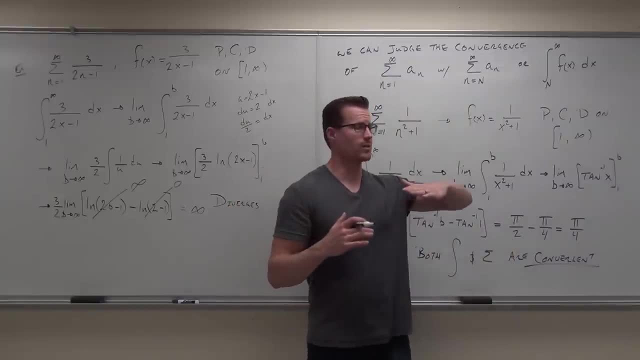 This is interesting because it said the integral acts as an upper bound. It also says it's an upper bound, It acts as a lower bound, It acts as a bound. So the integral is the bound for our series. It's either an upper bound if it converges or a lower bound if it diverges, which is 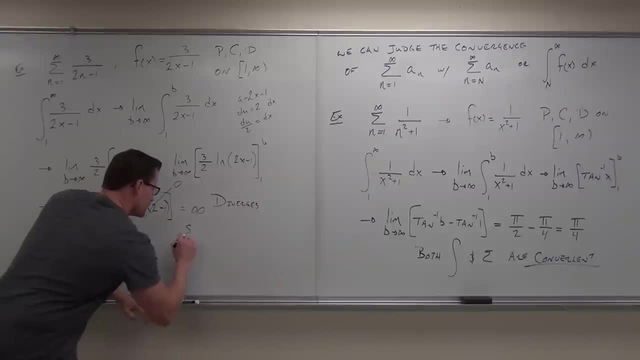 really neat. Therefore the series also diverges. And this is exactly the way you state it on your homework and your test. You say: the integral diverges. Therefore the series also diverges. You don't just end it with diverges. 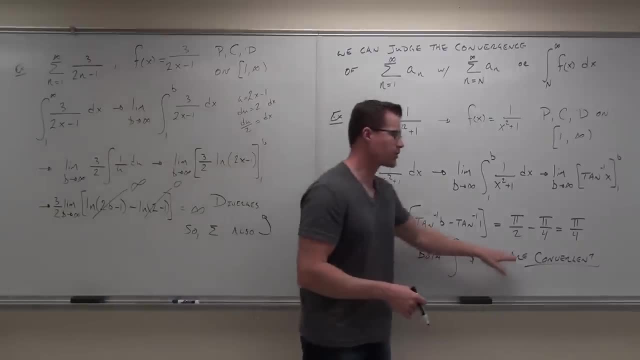 You make a statement about the series, You say okay, so they're both convergent, or they're both divergent. You say, because this one diverges, the other one diverges. Make some sort of a statement like that: Do some of you feel okay with this one? 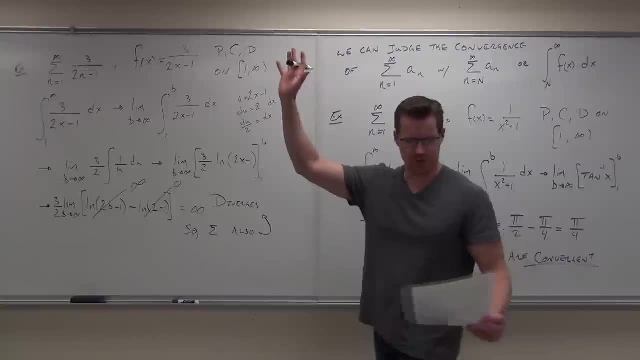 Tell you what I'm going to talk about. one more thing: We're not going to finish this, but I want to show you something while we're super fresh on this material: Minty fresh, Calculus fresh, Aqua fresh. 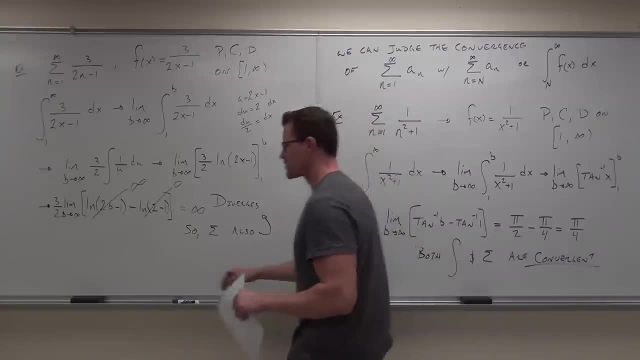 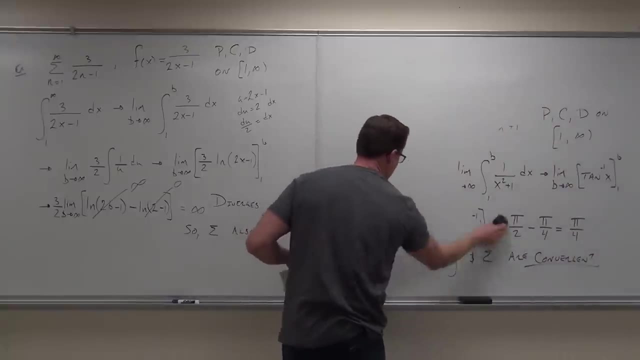 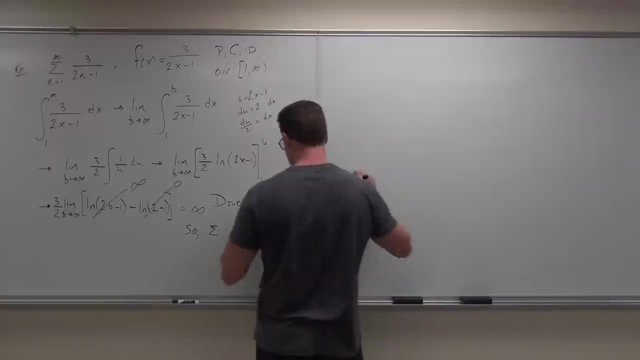 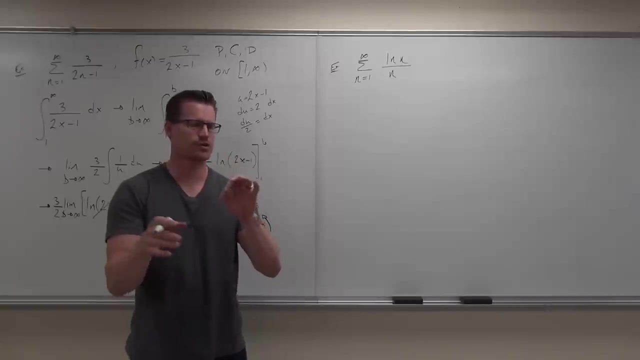 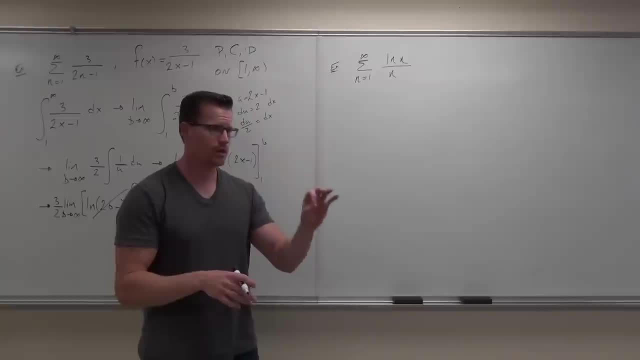 over an N. The first thing you would do here check your limit. Now, if you did lobe Victauls, you're going to find out that this limit does equal zero. but you'd check by the divergences test first. 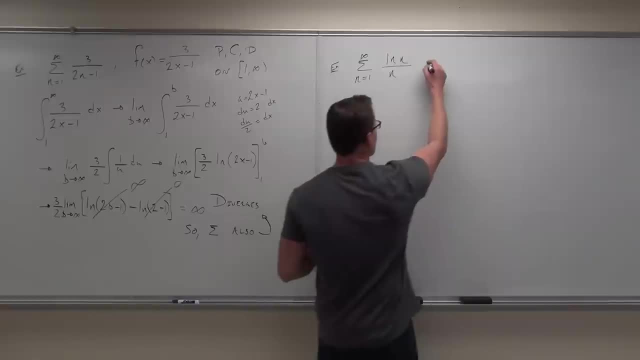 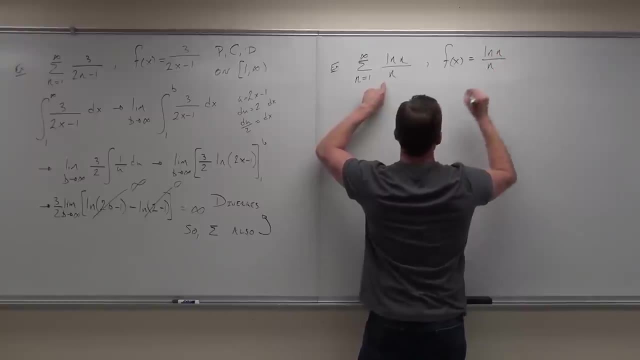 First, are you with me on that one? Always check that. Secondly, you go okay. well, you know what? I know that this series, if I model this function after that sequence, after this sequence, and I determine that the integral of this function, 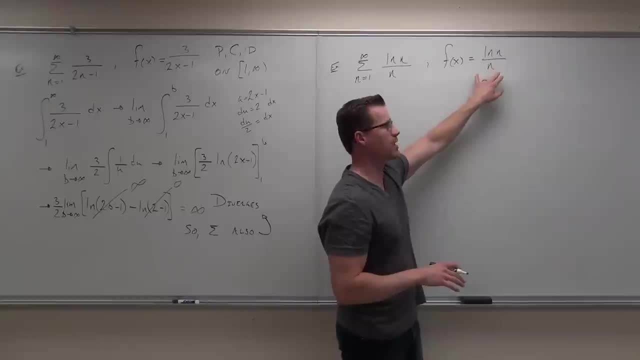 is convergent, this series convergent, divergent, this series divergent. as long as this is positive, continuous and decreasing. Now let's talk about those three things and then we'll end for today. okay, So is this positive? 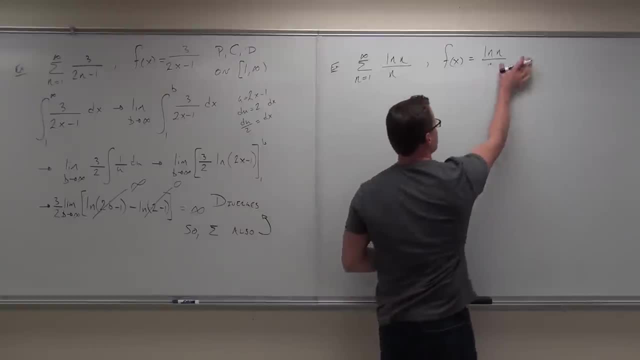 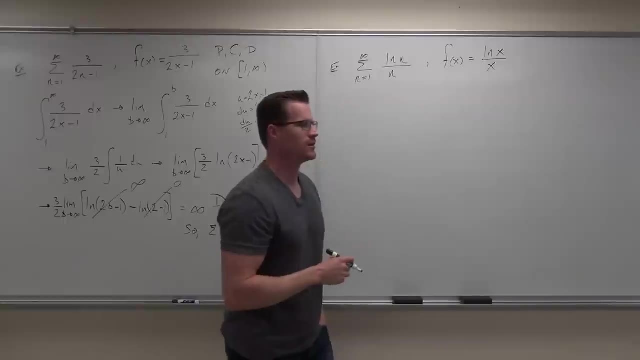 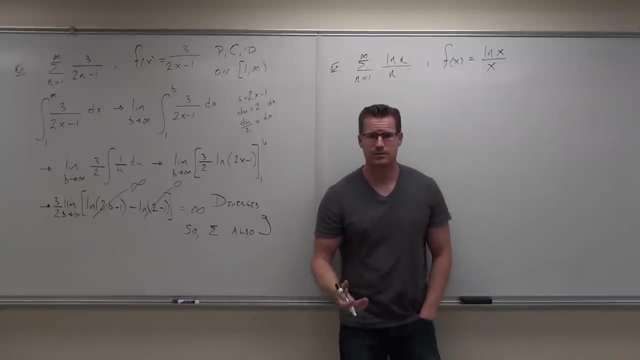 Your n should be x's. Oh, I'm sorry, thank you. Yeah, my bad good save, good catch. Not minty question anymore Tepid and rancid whatever. f of x equals ln, x over x. is it positive? 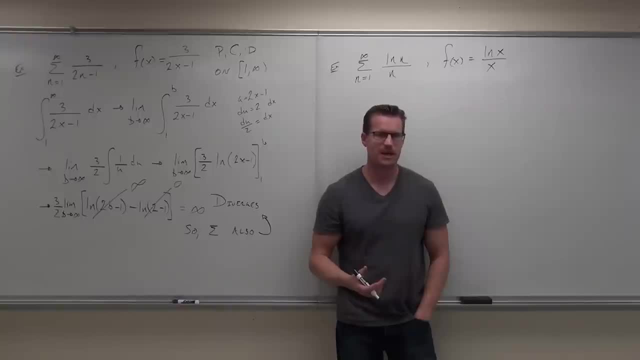 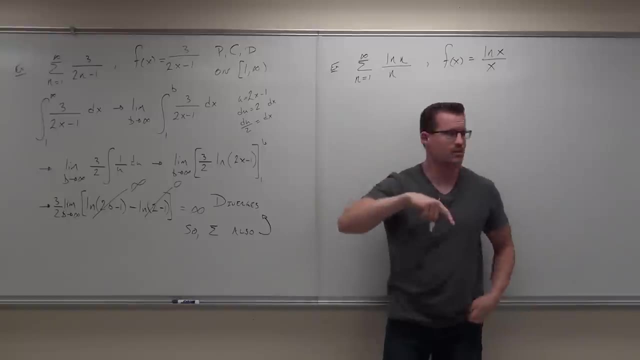 Yes, Is it always positive? No, No. Is it positive on this integral, Yes, Yes, after one, ln of one is zero. after that it's positive over something that's always positive. After one, you'd have something that is positive. 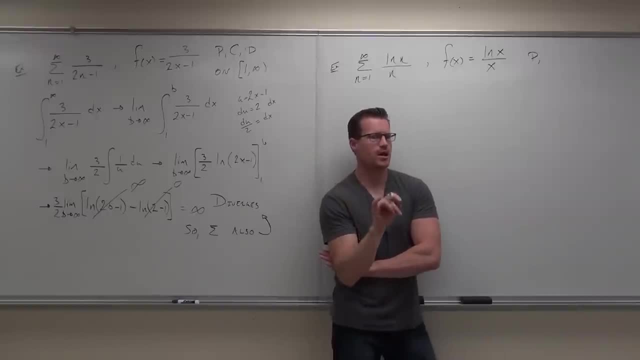 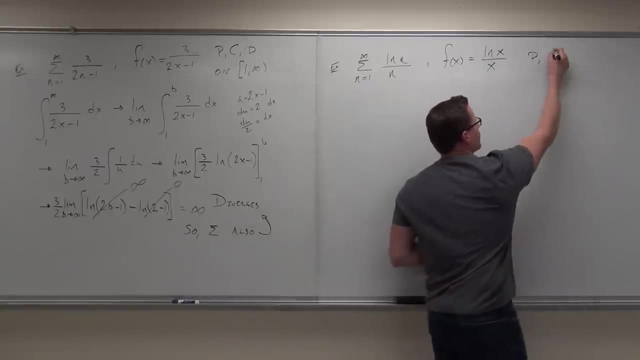 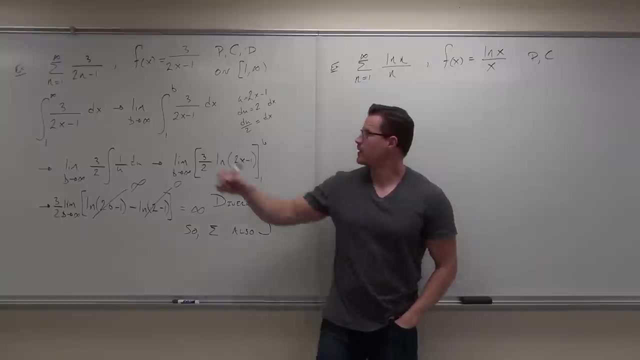 Is it continuous? No, The only discontinuity here would exist at x. equals what Zero? That would be discontinuous for both of them. actually, After that, it's continuous. Is it decreasing? No, This is not an obvious one. 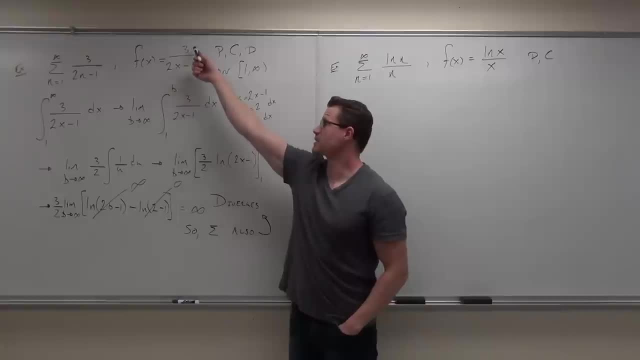 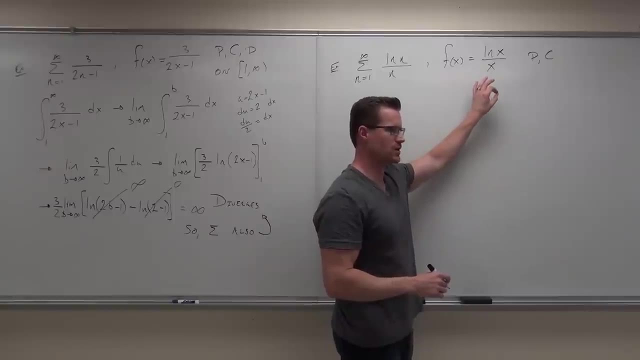 Obviously decreasing. that's a constant, that's over a number that's growing. that's decreasing. This one not so obvious. This time you're going to have to check for decreasing. So here's our check for decreasing. You must show these things, show decreasing. 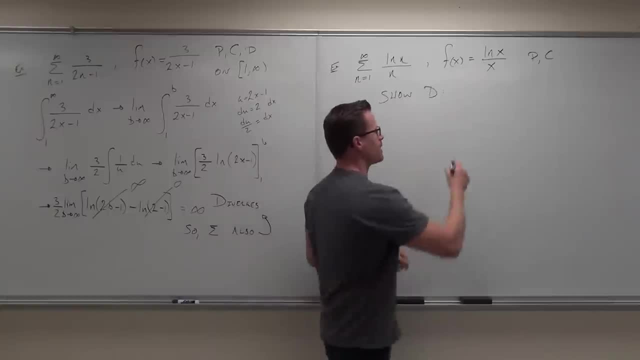 How I would show decreasing with a function. man, I would take the derivative of that function. Do you remember doing that? No, we just did that stuff right to show that this is decreasing. If it's decreasing, the derivative has to be negative. 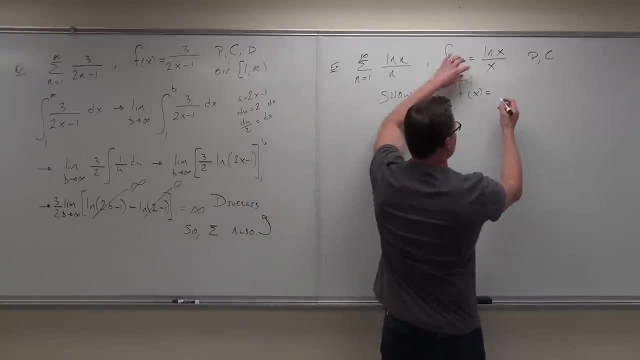 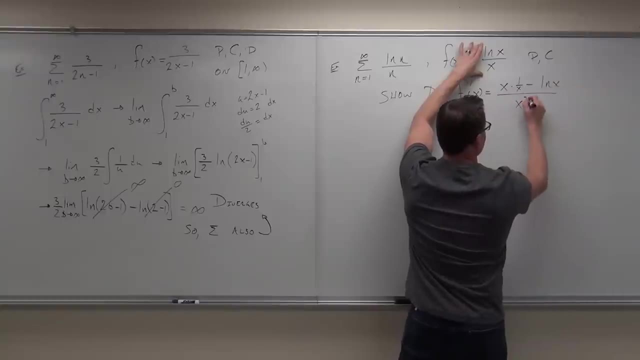 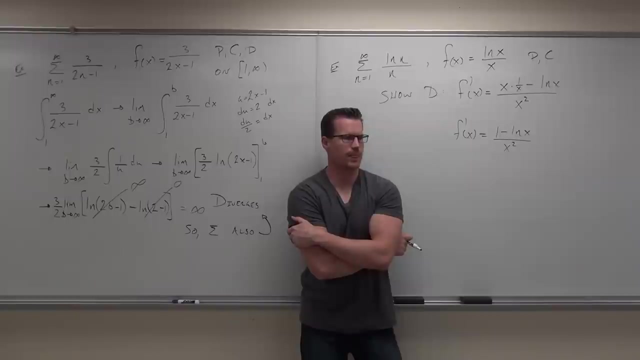 Decreasing means the derivative is negative. So if we do the derivative, it's low d, high minus high d, low, square the bottom and away we go. So our first derivative is one minus ln x over x, squared. You guys okay with that so far. 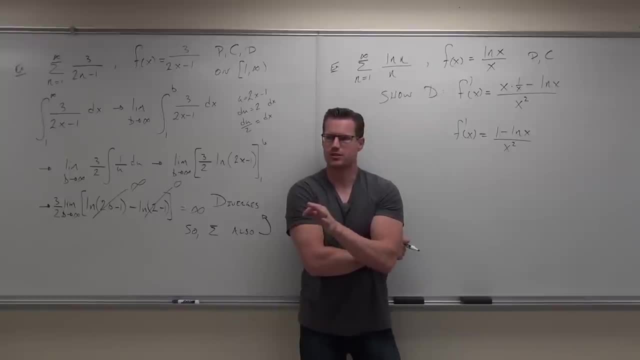 Well, here's the whole thing. We're trying to show decreasing, correct. We're trying to show when this thing is less than or equal to zero. That's what we're trying to show Now. here's the whole point. Is x squared ever negative? 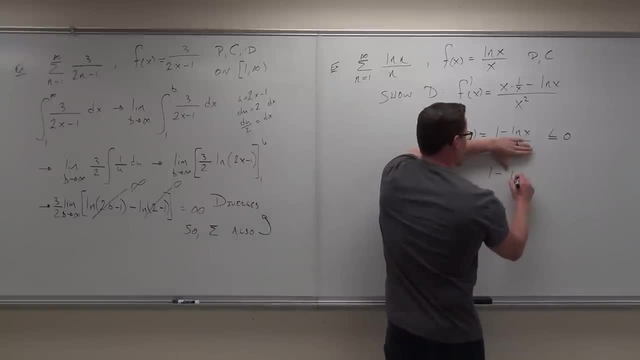 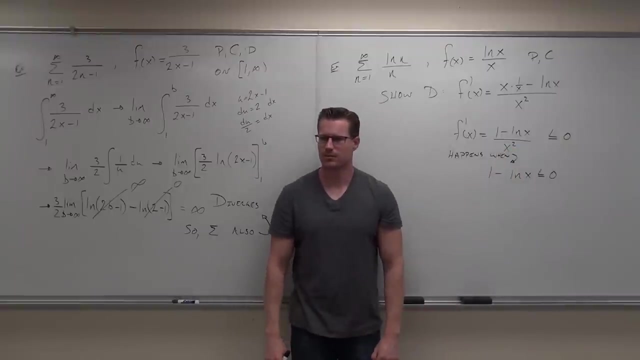 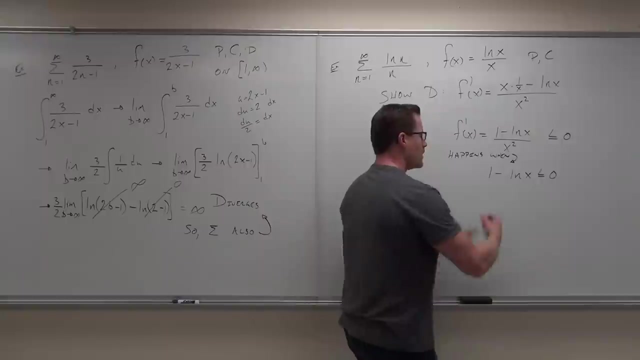 No, Then this'll only be negative. when one minus ln x is negative. This happens, when this happens, You guys okay with that one? Yes, no, Are you sure? Yes, sir, Yes, yes, If I solve for this, I get one is less than or equal to L and X. 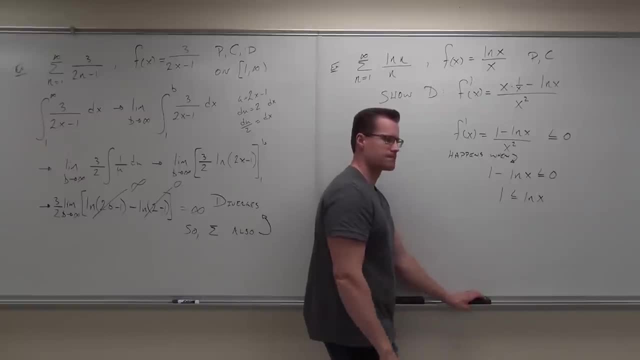 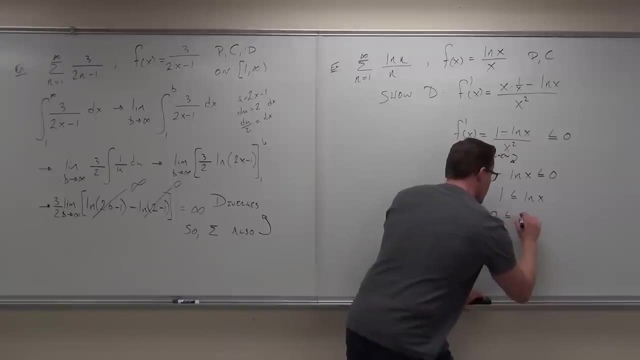 That's not good enough. I want to solve for X. Well, if I take both sides as an exponent of E, E to the first would be less than X, E to the L and X is X. So take E on both sides. 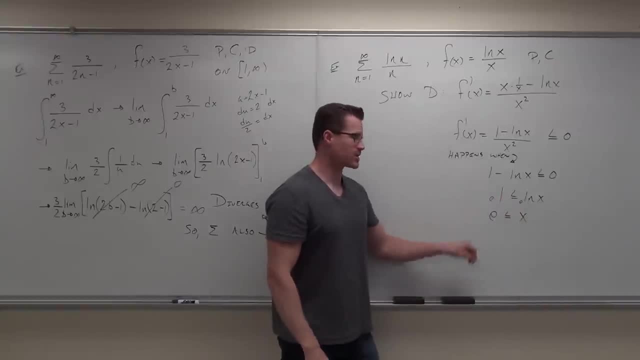 Don't take E, that's bad for you, But put E on both sides. this is the exponent of E. Here's what this says to me and hopefully to you. What it says is that this function is certainly positive. it's certainly continuous. 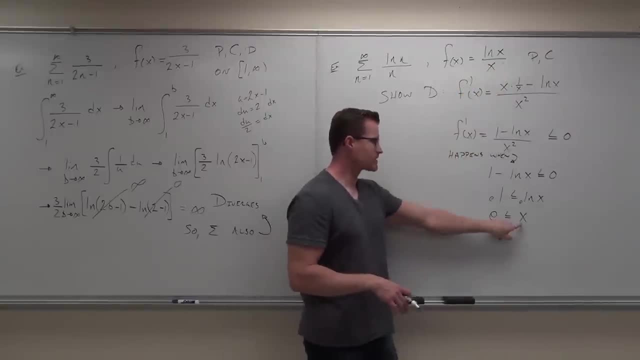 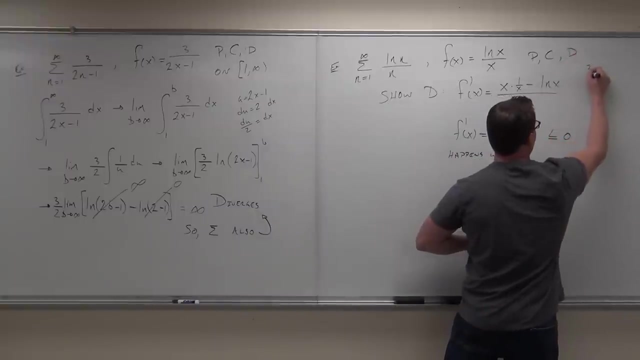 It will be decreasing as long as X is bigger than or equal to E. How much is E? 2.7.. Then what if I made this 3?? If I said this is decreasing on 3 to infinity, would it be positive? 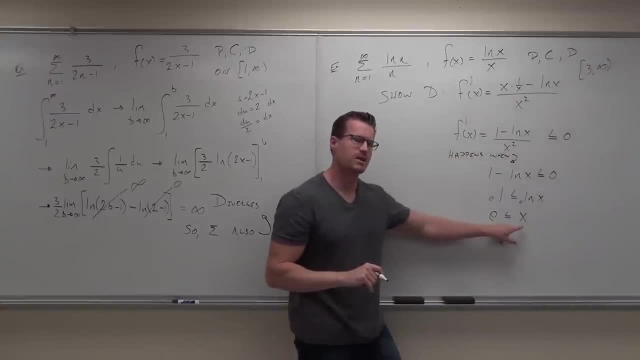 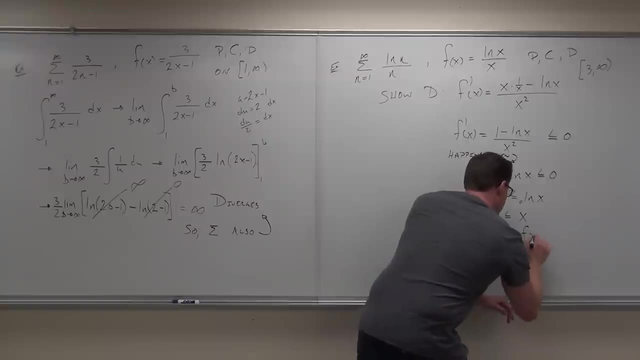 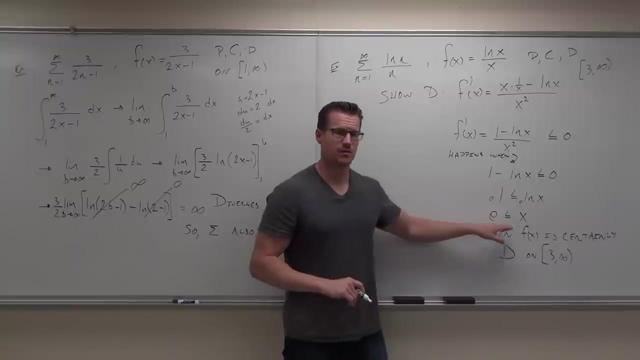 It would be true. If it takes X being bigger than or equal to E to be decreasing, then the function will certainly be that F is certainly decreasing on 3 to infinity Because 3 is bigger than E. it's that X has to be bigger than E. 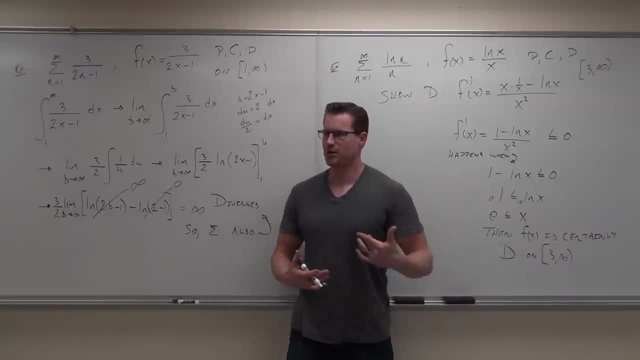 Well, 3 is bigger than that. Therefore, this is also decreasing on the interval from 3 to infinity. So, our integral, where's our integral? I'll see if you can put it all together. Where's our integral going to start? 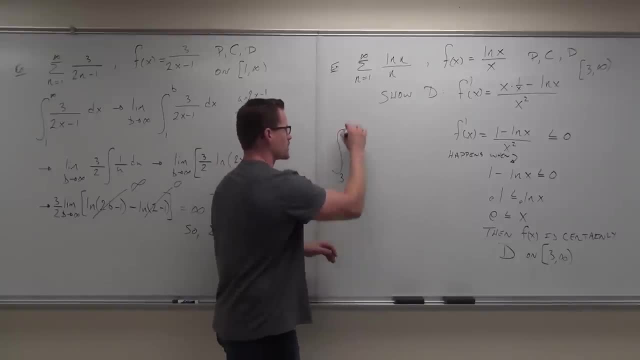 3. Not 1.. It's not decreasing there, But you start at 3.. This was the first thing that we talked about. in one of those notes It said that I can subtract a finite number of terms. Listen carefully to the last little bit, okay. 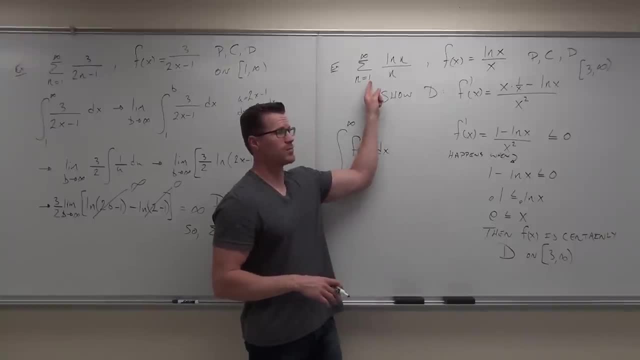 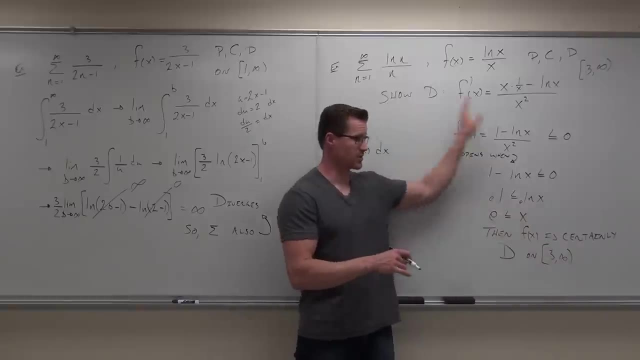 I can subtract a finite number of terms. I'm subtracting the first term and the second term. I'm starting at the third term. I don't want to start at E. okay, I want to make this an actual integer That matches up with our series. 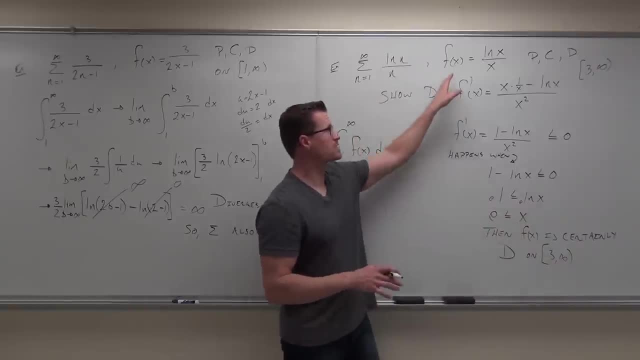 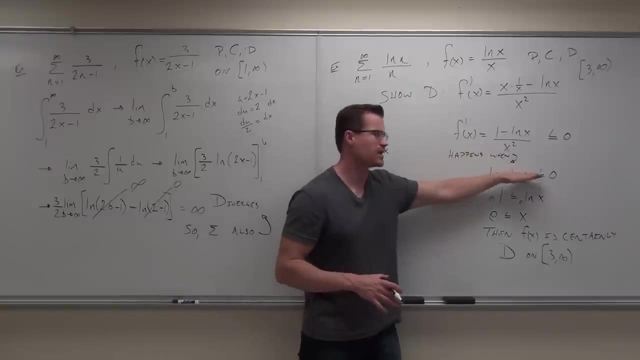 I'm going to start at 3.. So check positive check, continuous, You guys. okay with the decreasing part of this. Derivatives have to be less than 0 for decreasing. So show it, Hey, look it. This will be less than 0 when this happens. 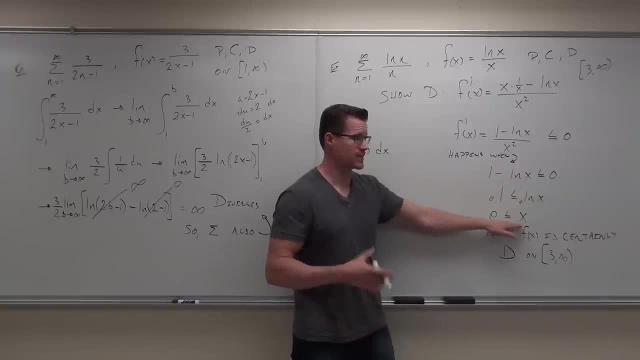 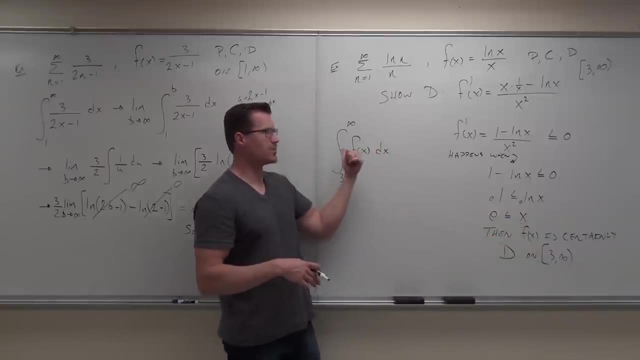 or when this happens to E on both sides. When this happens, X has to be bigger than E. Make it 3.. 3 is bigger than E. Therefore this will be positive. No problem. Continuous and decreasing on 3 to infinity. 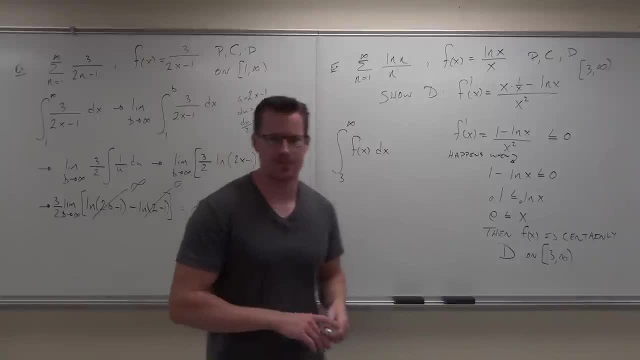 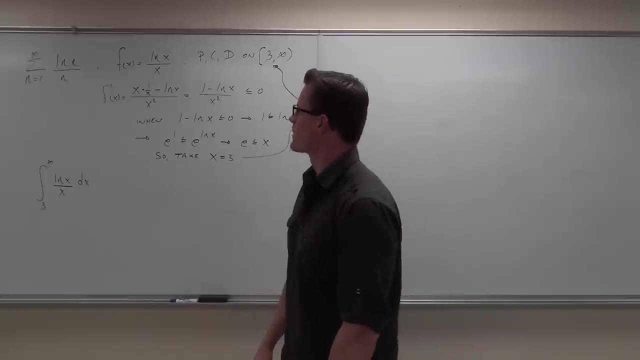 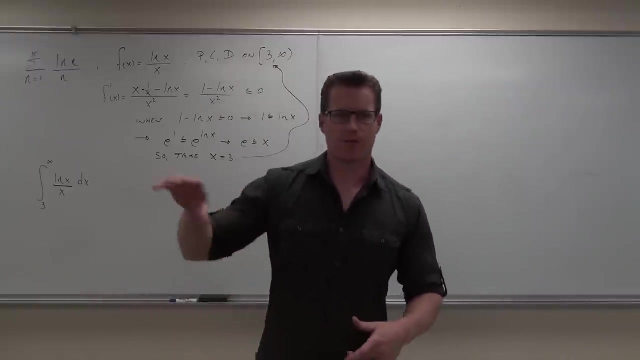 Start your integral at 3.. We'll finish it up next time. So we're going to finish up this problem. So if you were with us last time, what you saw was whenever we have these series and we can determine that our function that's based on our series. 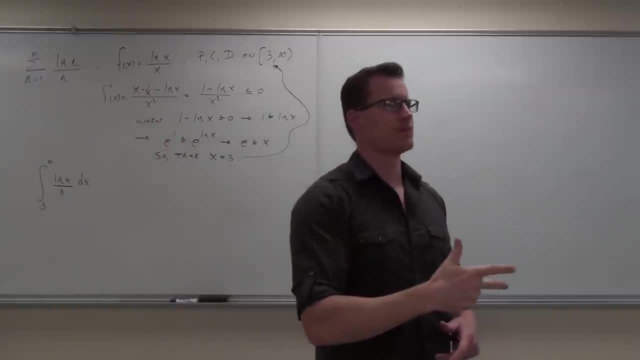 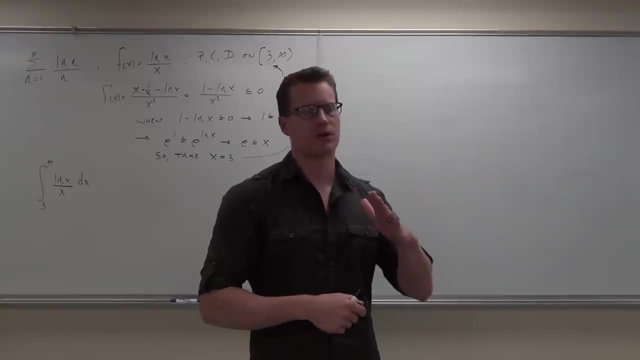 is positive, continuous and decreasing. we can take an integral of that function And what that function does. it stands for a lower bound for divergence or an upper bound for convergence. Basically, it says that every term of this sequence from which our series is built, 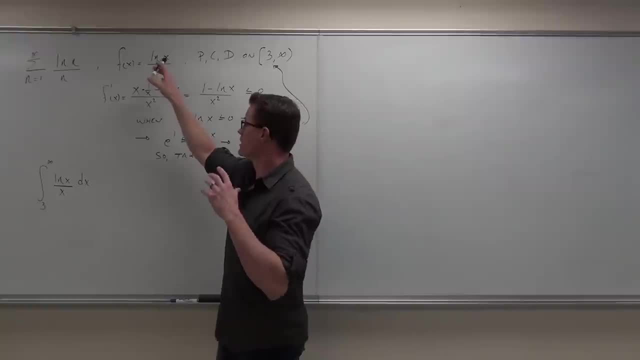 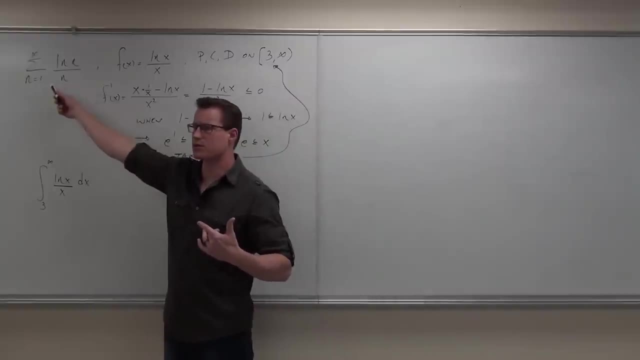 is found in this function. Therefore, if the integral of this function- remember, integral means add up stuff- if the integral of this function diverges, it means the sum or our series is also going to diverge If the integral converges. 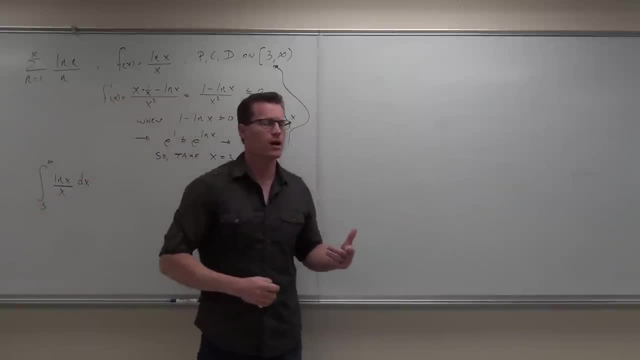 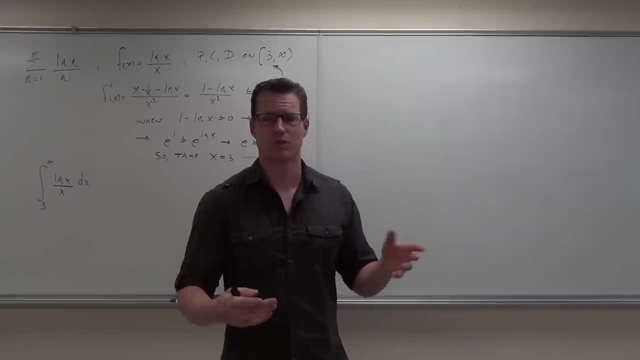 it means the sum or the series is also going to converge. That's the idea that we have Now. does the integral necessarily tell us the sum of our series? No, It doesn't give us the sum. It just tells us whether it will have a convergent sum. 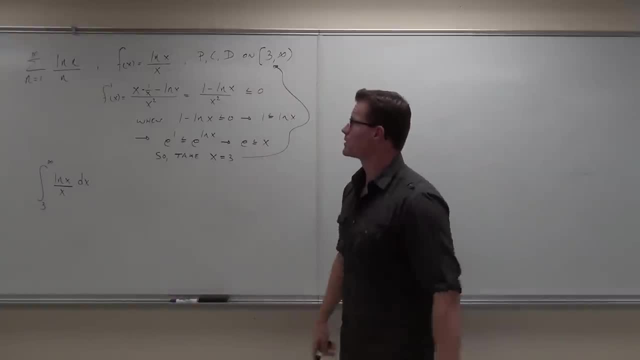 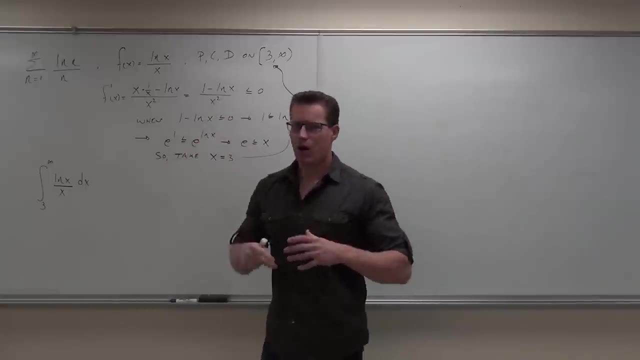 or a divergent sum. That's basically the idea. So what we've done here so far is just all right. let's call this function ln. So we've modeled it on our sequence We've determined. hopefully, obviously, to you. 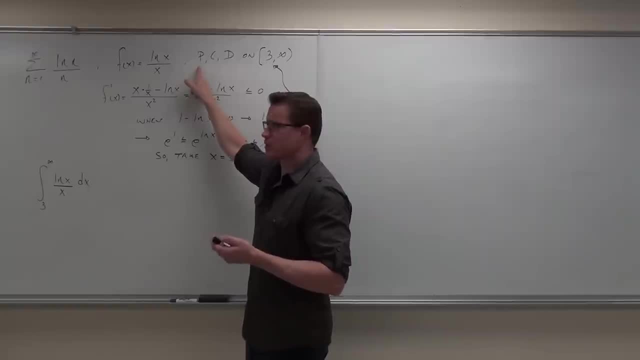 it is of course positive. It's definitely positive, That's positive and that's positive after 1.. Therefore, positive over positive gives us a positive. It's definitely positive after 1.. It's continuous. The only problem we would ever have is at 0.. 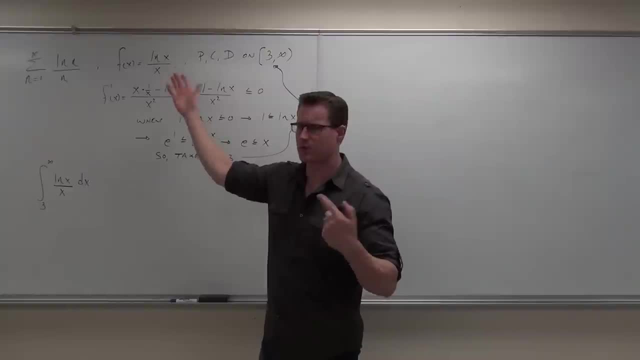 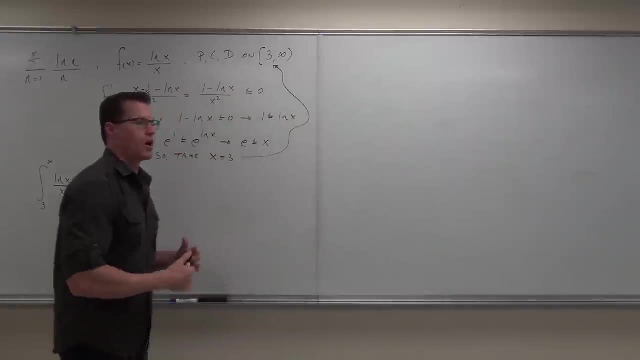 Since 0 is outside of our interval from 1 to infinity, no problem. The problem we came across with this problem was the decreasing. How do we show decreasing oftentimes with our functions? Take a derivative, If a derivative is less than 0,. 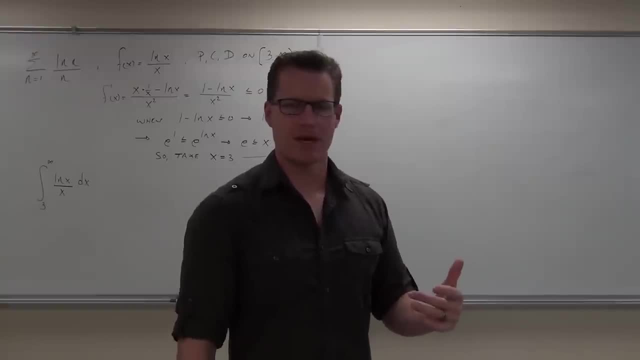 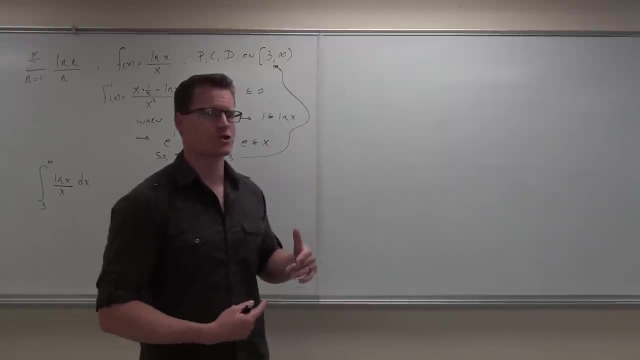 if a derivative is negative, that means that our function is decreasing. If a derivative is positive, that means our function is increasing for a given interval. What we're trying to show is that this function is always decreasing. Does that make sense to you? 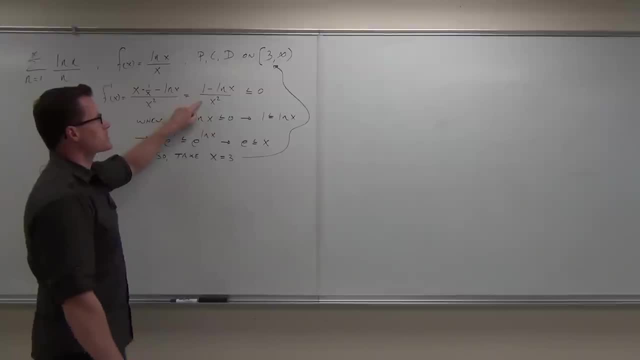 So we take a derivative, Our derivative. you should know how to do that. We say, okay, when is this derivative going to be less than 0?? Well, this derivative is less than 0 when the numerator is less than 0.. 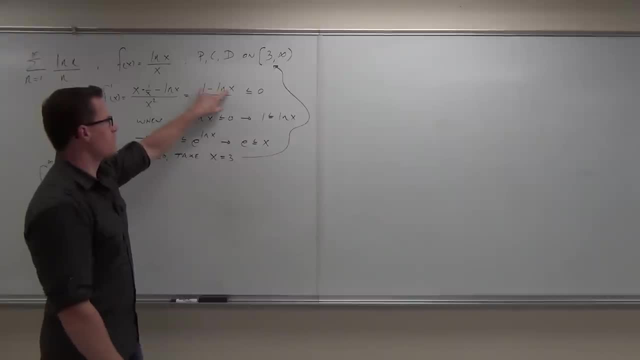 You see, the denominator is always positive, so we can't change our sign. So it's always the numerator less than 0 for this example, No problem. Well, if the numerator has to be less than 0, for a derivative to be less than 0,. 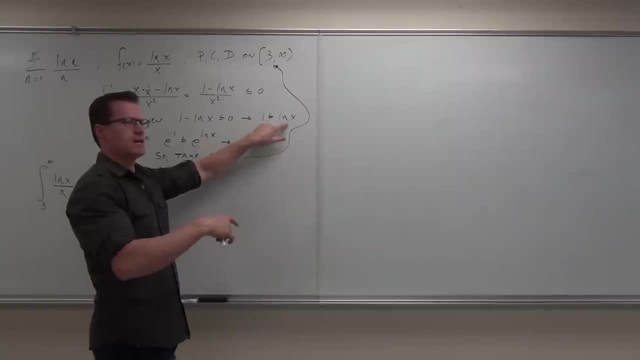 that means that 1's got to be less than ln x. If I take both these sides as an exponent upon e, I'm going to get e to the first is less than e to the ln x, No problem. What that basically says is this: 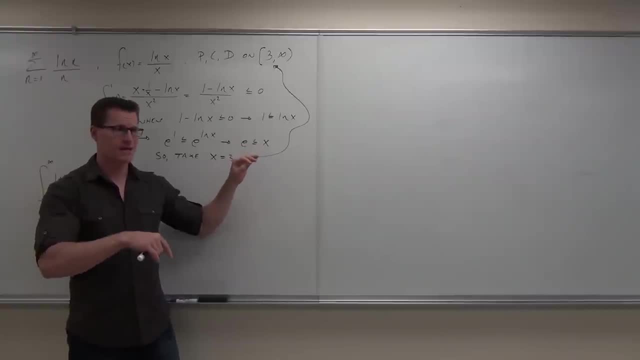 The derivative of our function will be negative when x is greater than or equal to e. That's the idea. Does that make sense to you? So basically, it says our function is decreasing everywhere after x equals e. That's what it says. 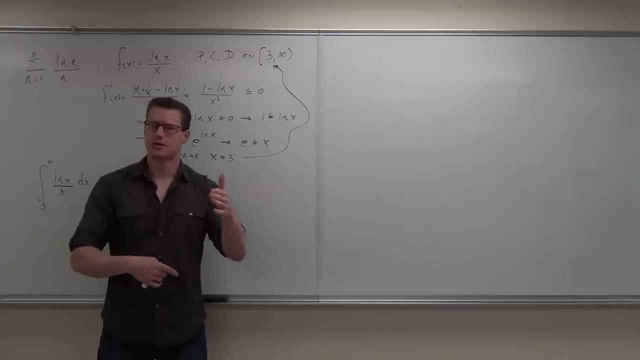 Well then, what we're going to do is we're going to pick some number after this, after e, Well, what's slightly bigger than e 3. 3 is We're going to say: well, you know what? 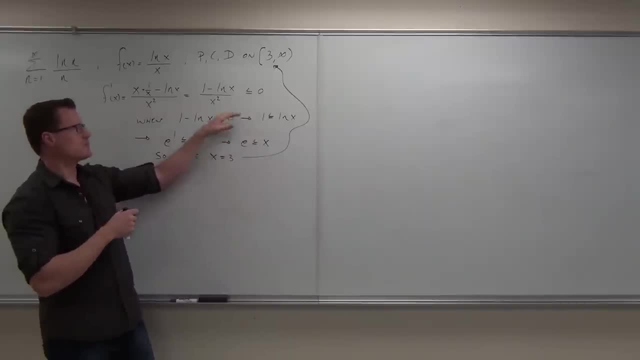 Tell you what Did you follow this logic down? by the way, Decreasing means less than 0.. That means this would have to be less than 0. That means this would have to happen. this would have to happen and x would have to be bigger than e. 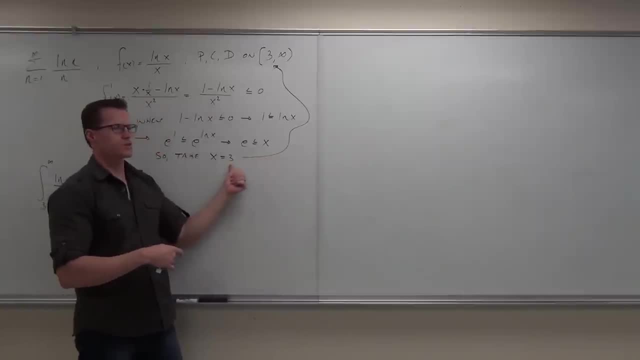 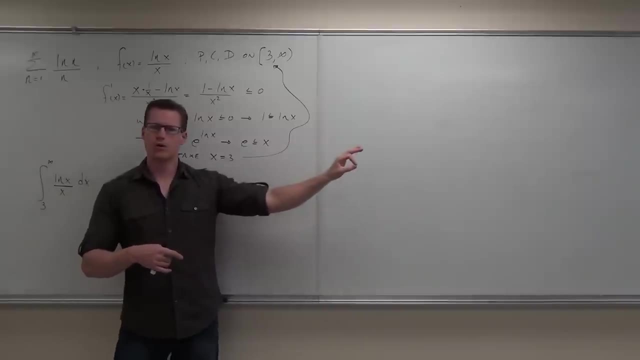 That's what that says. Well, pick x equals 3, and then we know for sure that our function will be decreasing at x equals 3 and further, all the way to infinity Show fans, if that makes sense to you. Now the reason why we're allowed to do this. 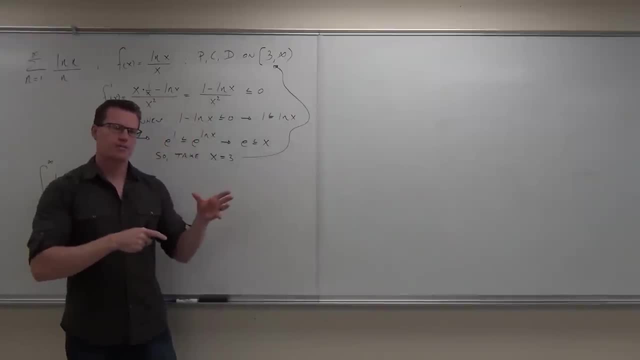 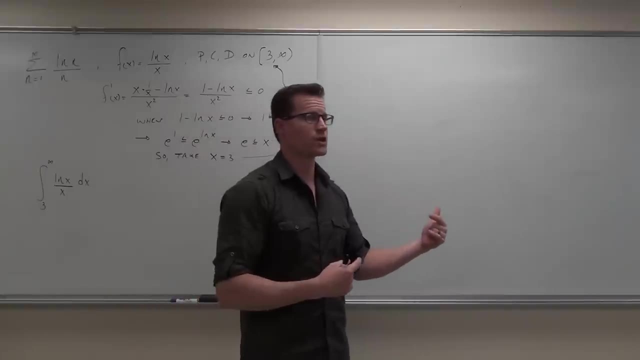 I gave you this statement last time. you can actually add or subtract a finite number of terms from your series and the resultant of convergence or divergence will not change. So I know that our series, where does our series start? Where's our integral going to start? 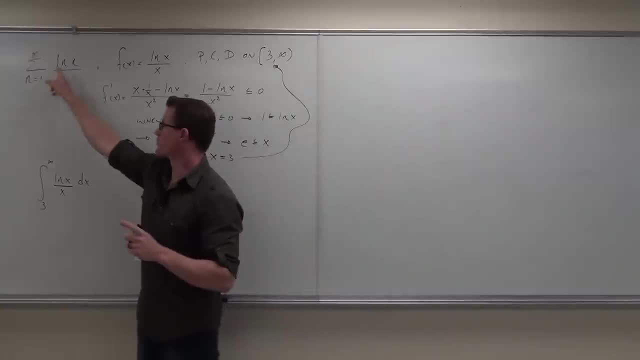 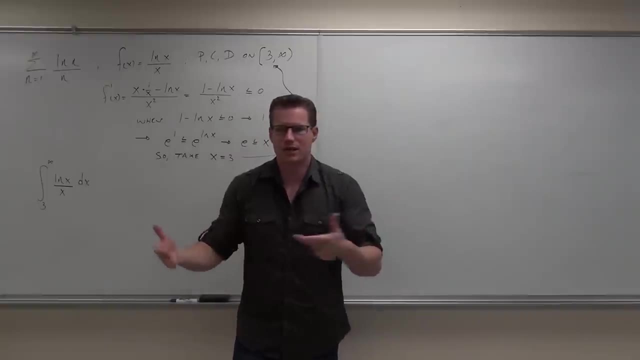 That's two terms difference actually. So we would ignore the first term and the second term and start with the third term. Is the sum going to be the same? No, it's going to be different. Who cares? It's not going to give us the sum anyway. 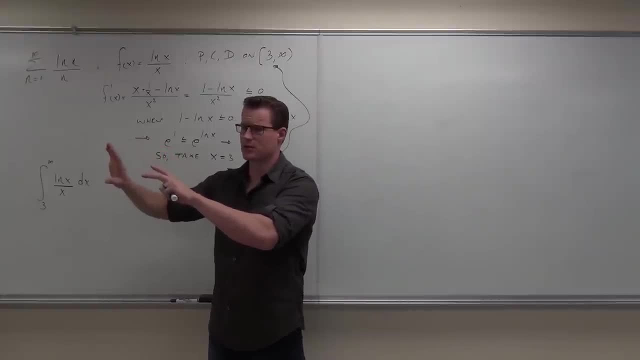 So it's just going to tell us: well, if I subtract a finite number of terms, who cares? It's going to give us whether this series is convergent or divergent anyway. Does that make sense to you? I think I explained it last time. 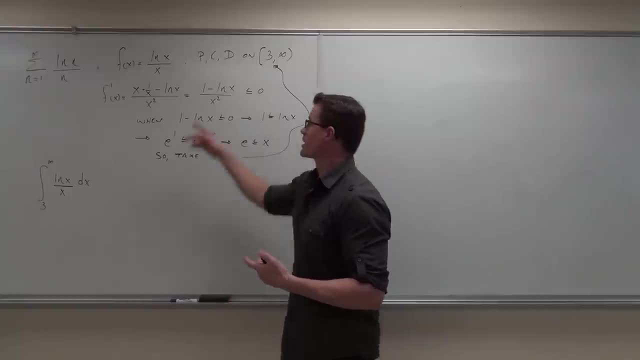 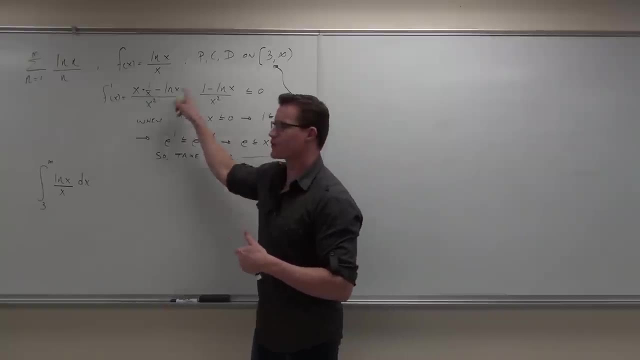 but I wanted to make sure that you guys actually got to it. So we check positive easy, Check continuous easy on this interval, On one to infinity. that's both positive and continuous. Good to go Decreasing. take a first derivative. 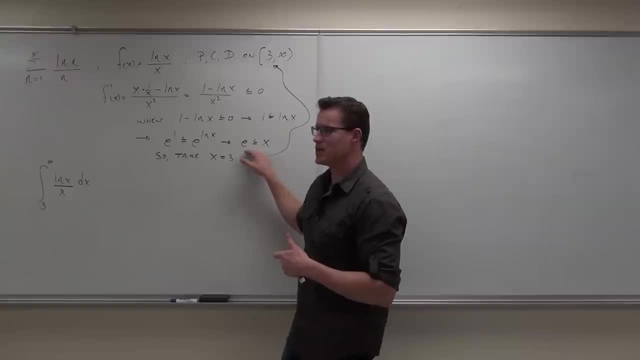 work it down. find out what x has to be for this function to be decreasing. For us, it's anything bigger than e, Well, three's bigger than e. so let's make our interval from three to infinity. Now, what that says is that: 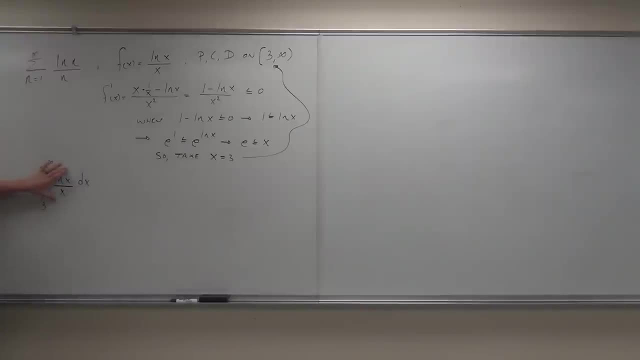 the integral of this function will have the same result as the series does. Either both will be convergent or both will be divergent. So we just got to do this integral. Fortunately for us, man, it looks so familiar. We've done that. 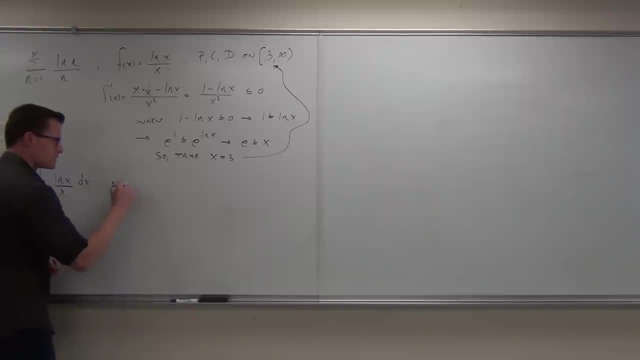 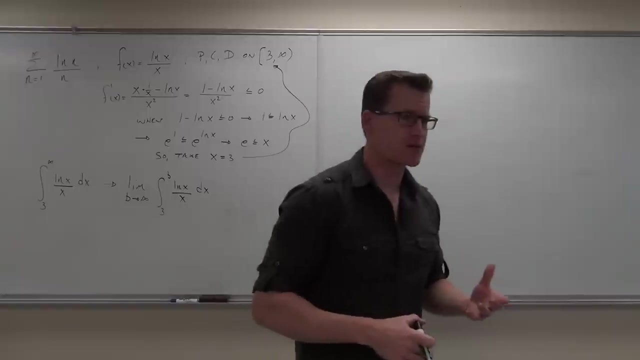 That's an improper integral. So what's our first step with an improper integral, please? From what? Integral? from three to b, ln, x, over x, dx. Now, of course, we're kind of past the whole integration phase of this class. 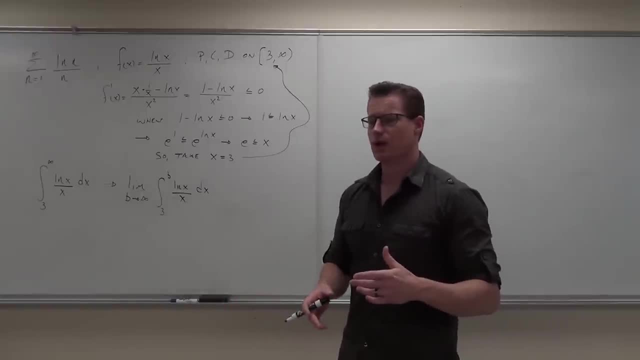 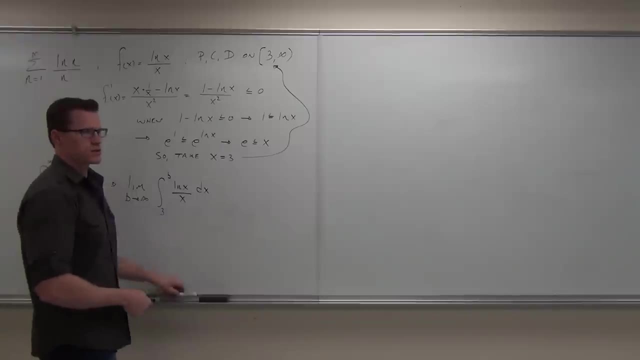 We're still going to use it, but these are going to be quite a bit simpler than what you're used to, So think easy on these things right now. How would I do this? You sub, You sub. What's our sub? 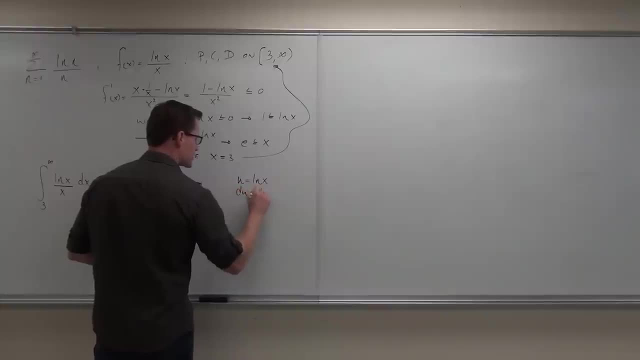 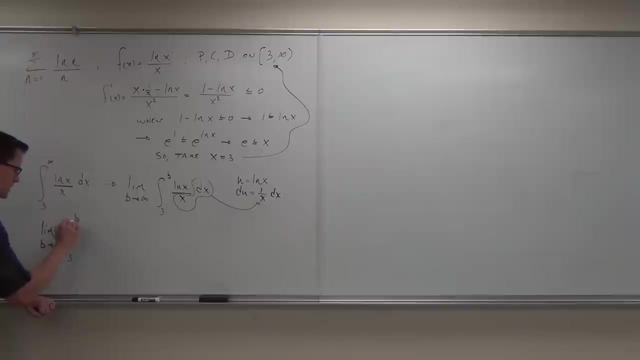 ln x Yep du equals one over x dx. Do you see it? It's right there. This is one over x dx. Therefore we have a limit As b approaches infinity. the integral from three to b of well. 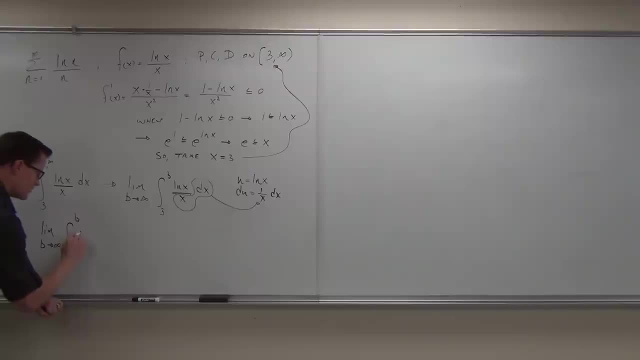 since I do my substitution, u equals ln, x, so I'm going to have u. du is one over x dx, So du is this piece. Well, that was pretty painless. That means we're going to get l, the limit of u squared. 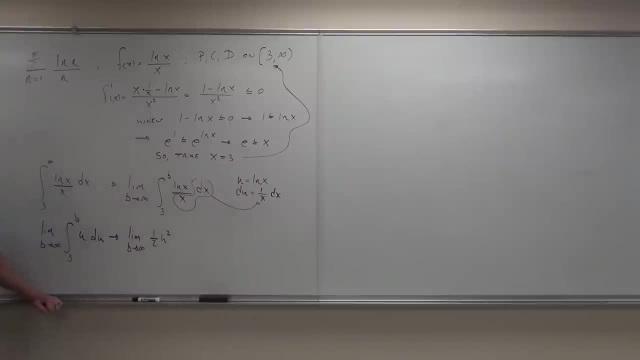 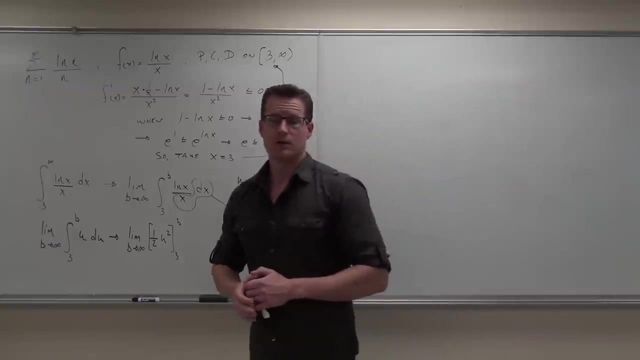 over two, as b goes to infinity from three to b. So fancy feels, so far, so good on this thing. Now there's one little issue. What's the little issue that we have Bounds? Bounds are different from our variable right now. 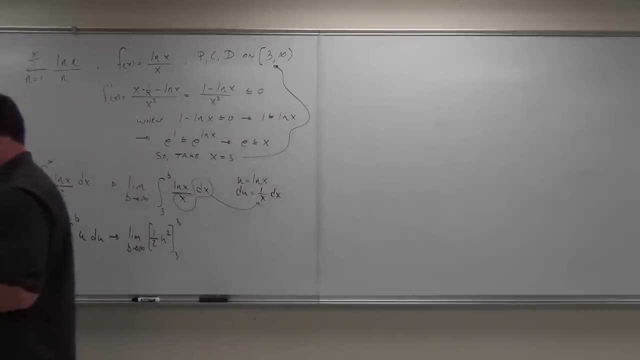 And since we haven't changed bounds, what we're going to have to do is we're going to have to resubstitute back in. So, instead of having u squared over two, we're going to make this the limit, as b approaches infinity, of one half. 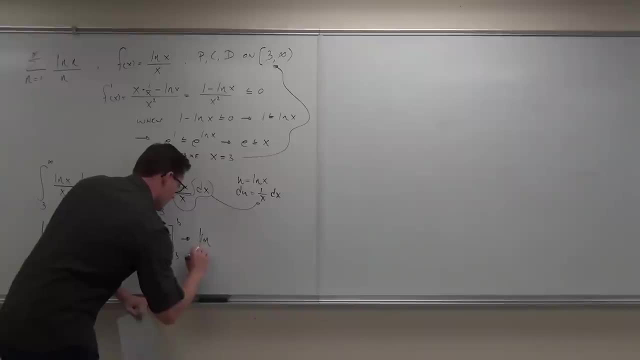 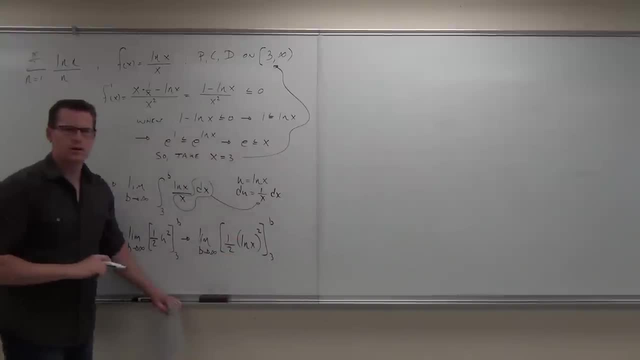 And take that from one to b. Sorry, three to b, My bad. You all OK with that so far? Yeah, Cool, Let's go for it. Is any of this hard for you at this point? No, No, We know how to do simple interviews. 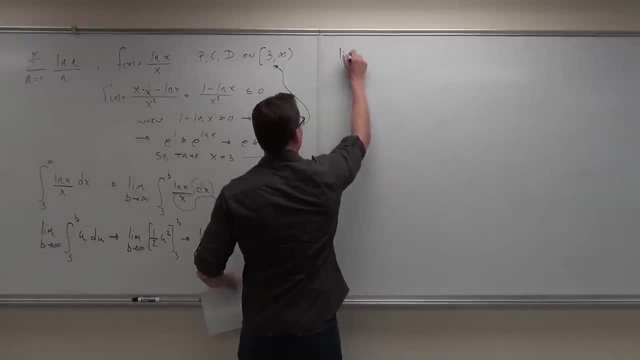 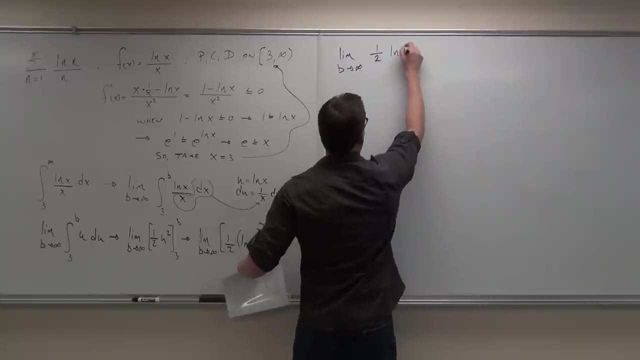 It's not a problem. We know how to evaluate. So when we do this we're going to have a limit. b goes to infinity. Looks like it'll be one half ln b squared minus one half times 1 1⁄2 ln 3, squared. 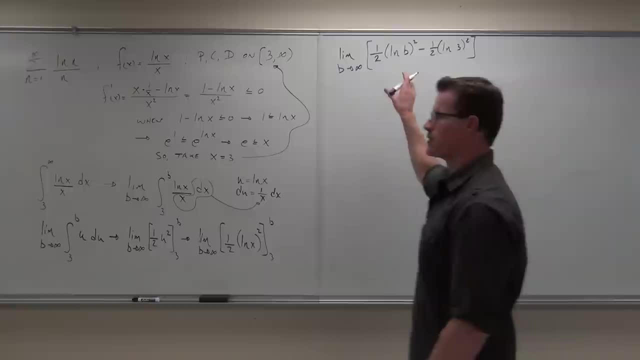 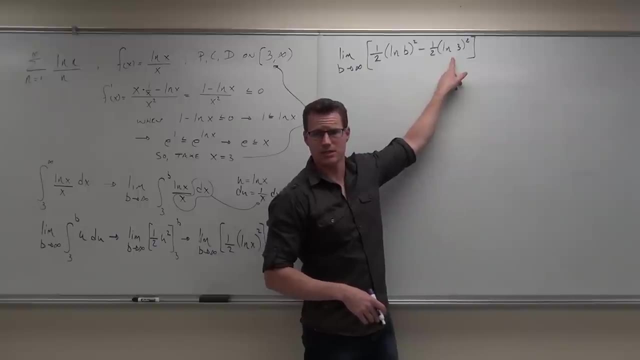 Can you please tell me what's gonna happen? What's gonna happen with this limit? What is, what's ln 3? No idea, But this is gonna be some sort of constant, isn't it? So this is gonna be some constant. 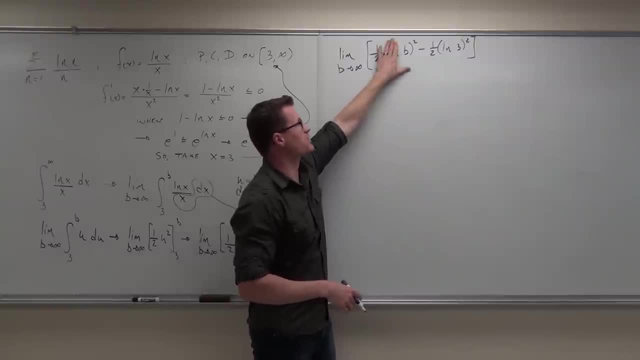 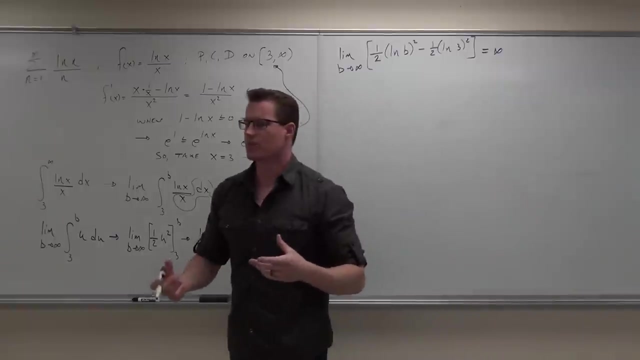 How much is ln B as B approaches? remember B's approaching infinity. How much is ln B? What's infinity? squared Times 1 1⁄2?? It's still infinity. Infinity minus a constant Of infinity. Tell me something about this integral. 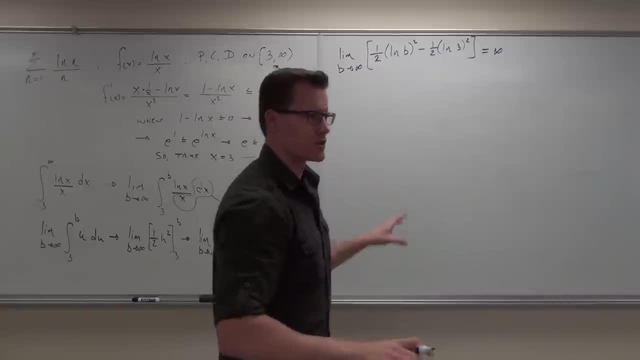 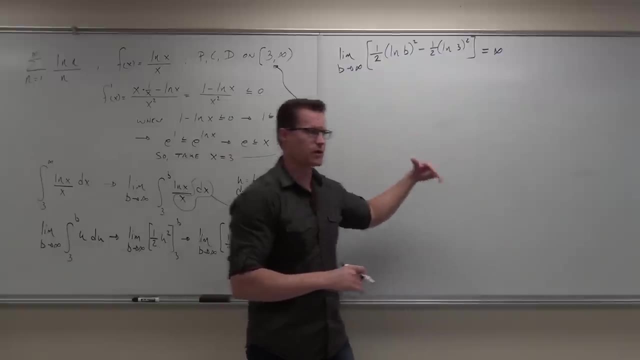 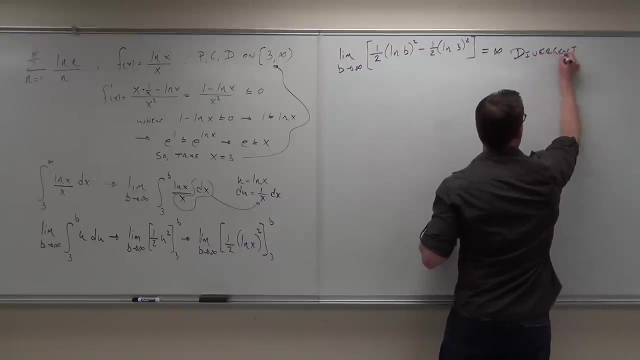 Is this improper integral, convergent or divergent? Convergent Why? Because it's like infinity, Very good, The limit goes to infinity. therefore, this integral is divergent. So, or the integral diverges. Now, what we said was because this function. 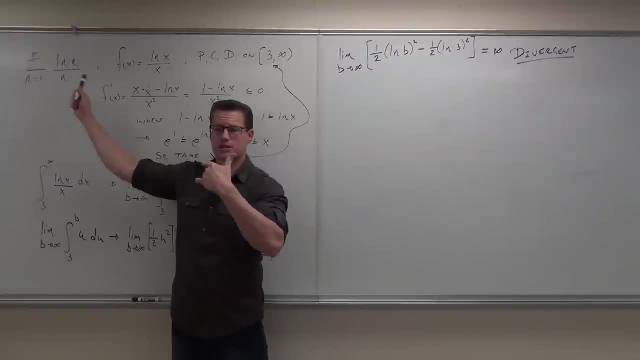 is modeling this series. it contains every term of our sequence and it's adding stuff together, just like our series would do. A series adds the terms. Well, the function basically adds up areas. basically the same thing. Since this is modeling this, 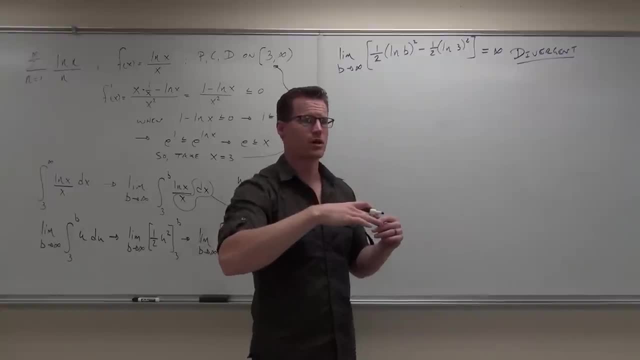 it's an upper bound for convergence, it's a lower bound for divergence. What that means is if our limit of our integral, basically if our improper integral, diverges, tell me something about our series. Inoperative, You have to say that, okay. 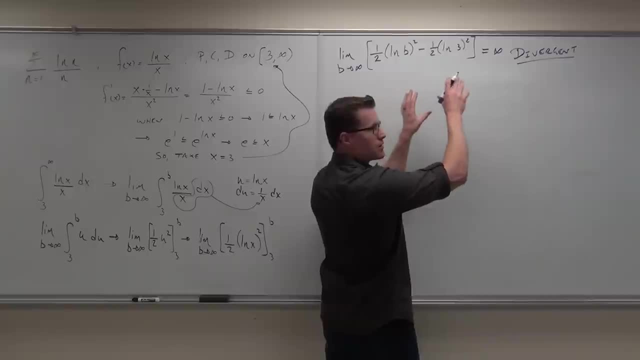 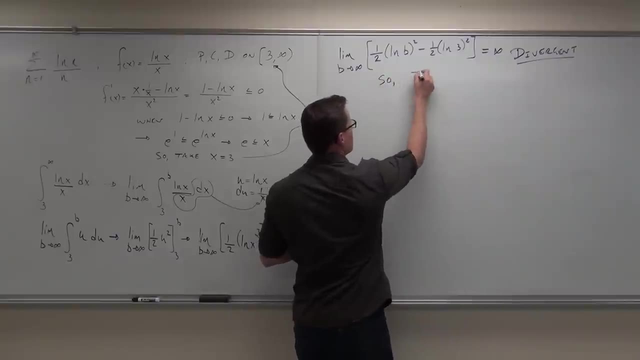 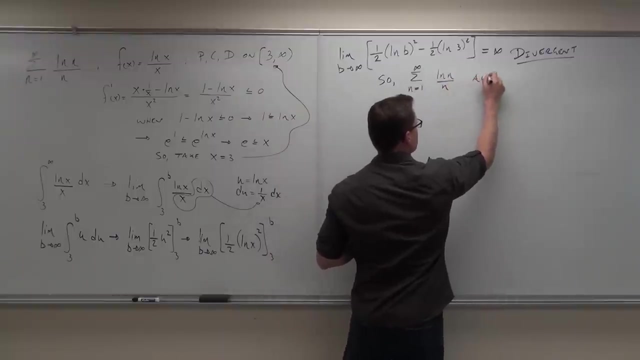 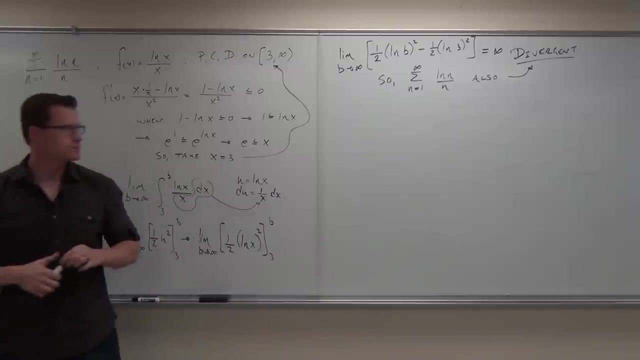 You don't just leave it divergent done. You say so because the integral, the improper integral, diverges, the series also diverges. So we say so, series of ln, n over n also diverges. Quick show of hands if you feel okay with this so far. 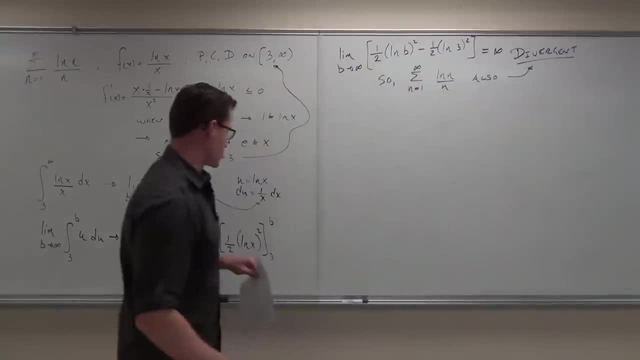 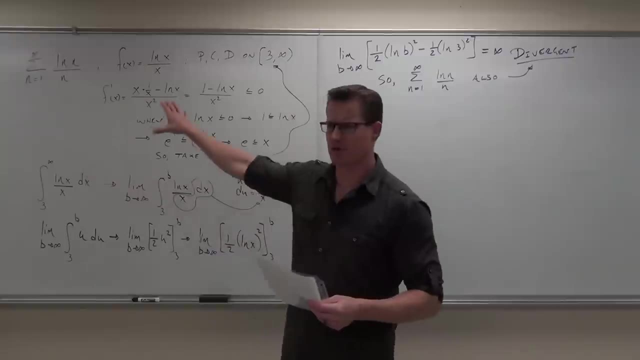 All right, we'll tell you what we got a little bit left to do in this section. I'm gonna go through what is called the p series. Go through that one. I'll do one more example of this, very similar to this problem. 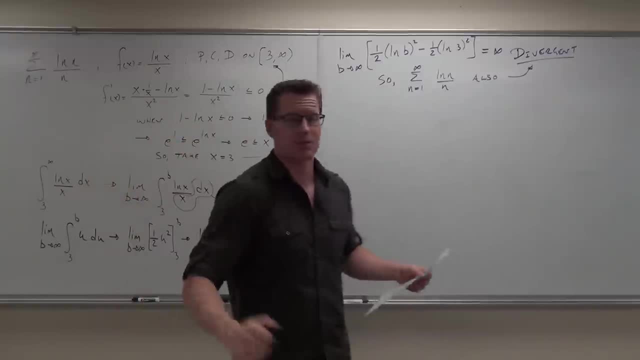 just to get our brains wrapped around it one last time And then we're basically done with our section. So last little bit we gotta talk about is something called the p series. Here's what the p series stems from. It says: suppose you've got a series. 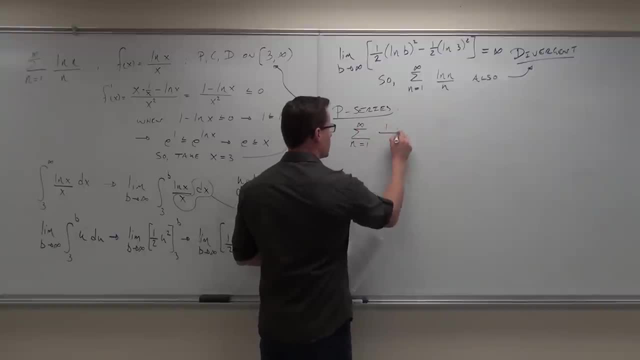 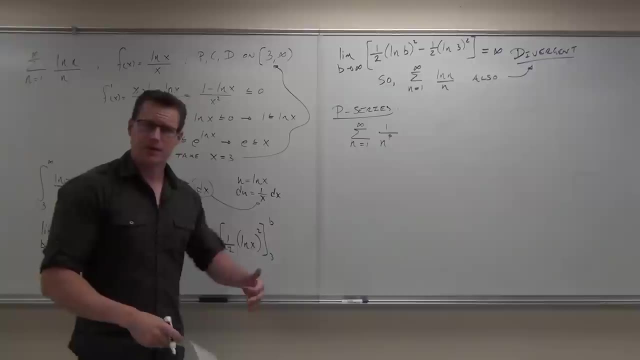 suppose it starts at one to infinity, and it's one over n over n, and it's one over n to the p, Where p does not change, The n is what changes. I want you to think about what this would look like, okay. 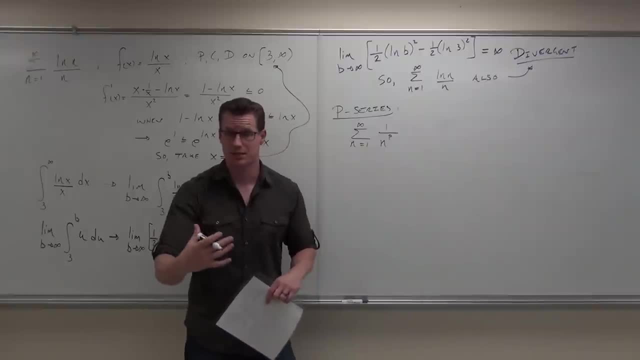 Let's think about the first few terms just to get our head wrapped around. what the world of the p series? So notice n's our index right. N is what's changing. So would the p change? No, the p's gonna be something like two. 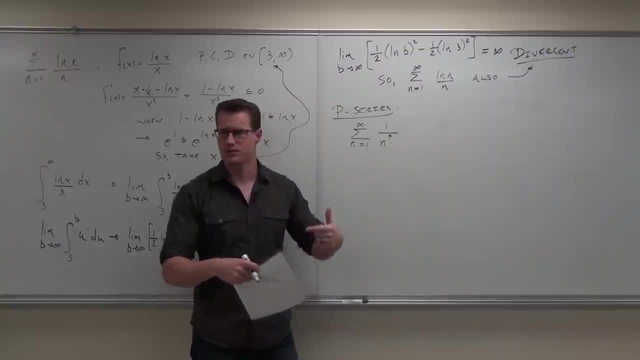 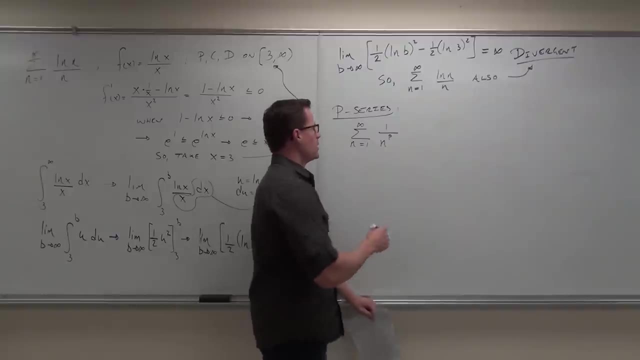 three, four, whatever P's gonna be some sort of a positive number not equal to one. Well, it could be one, but then we have something, but it's not very interesting. So here's what happens. Actually it is interesting. 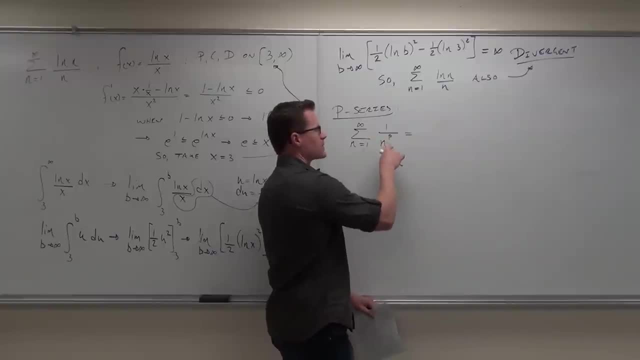 It's just something we've already covered. I should say it that way. Here's what happens: If I plug in one. I'm gonna have one over what N? What is n? One? What's one to any power One? 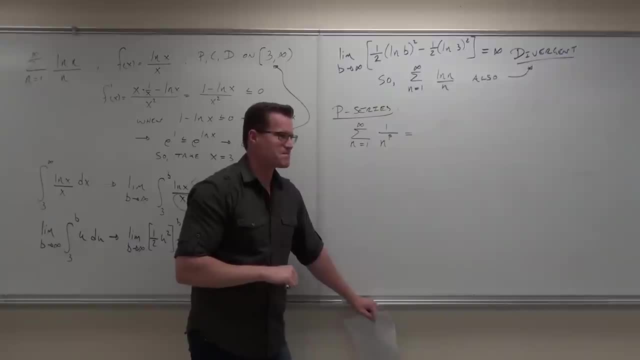 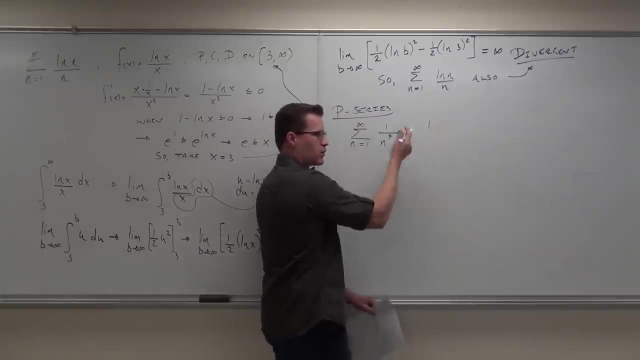 Excuse me, hope I didn't blow the speakers out on people's computers. That was loud. Well, if p's a power, hey, p power cool. If p's a power, then I'm basically taking one over one to the whatever power. 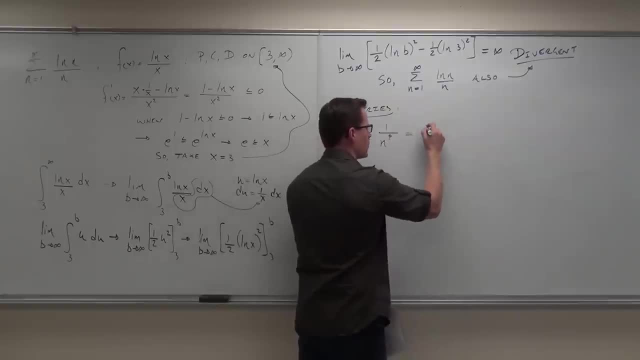 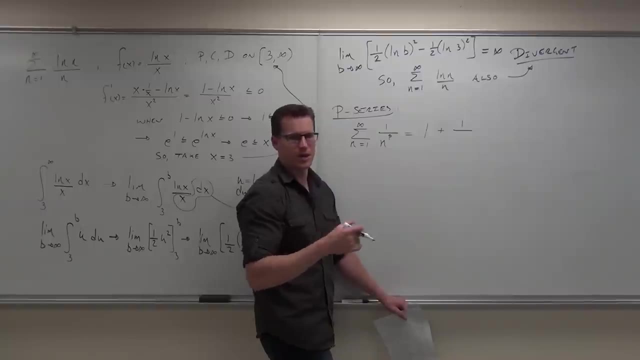 It's gonna be one. You see that. So I'm gonna get one for my first term. Next, I'd get one over. what would my n be? Two, Two. What would my p be? I don't know, It'd be whatever. I tell you it is. 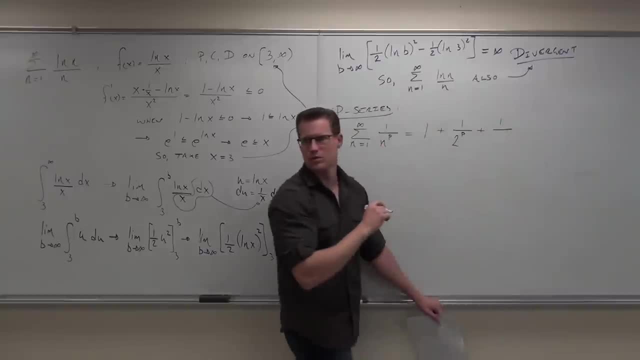 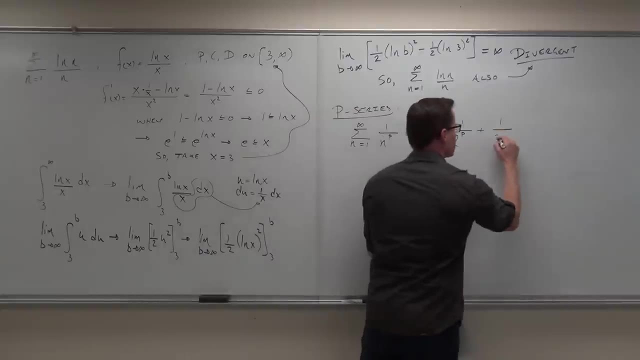 It's gonna be two to the p plus one over. what's the next one gonna be Three. Three to the what P? P? Is the p changing? No, No, it's gonna be whatever's defined in your series. 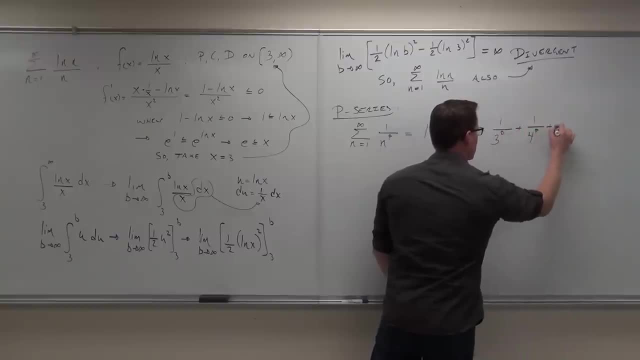 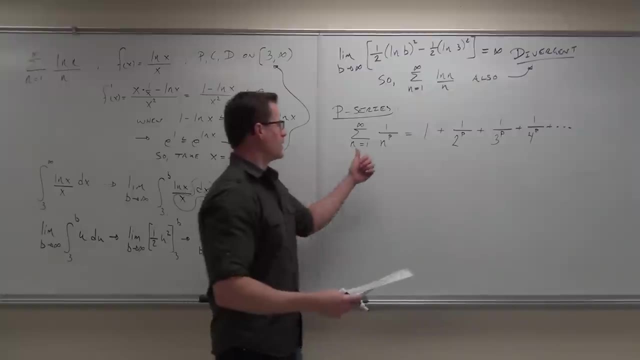 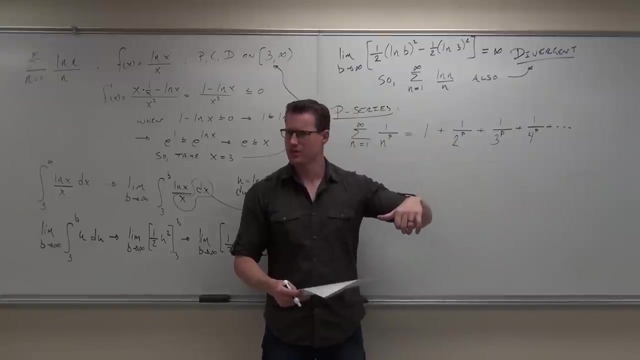 Three to the p plus one over four to the p plus forever. That's what a p-series does. It's basically taking your n and raise it to some power under one one over whatever that happens to be You guys. okay with the idea of a p-series? 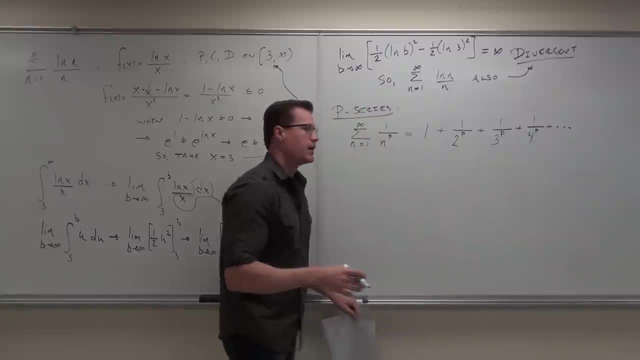 Yeah, Now we're gonna talk about when this converges and when this diverges, And basically we're gonna talk about the idea of a p-series. Basically, we have everything in hand to do that, So this will always converge. 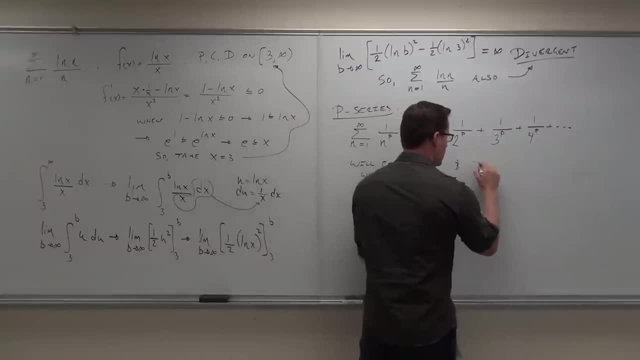 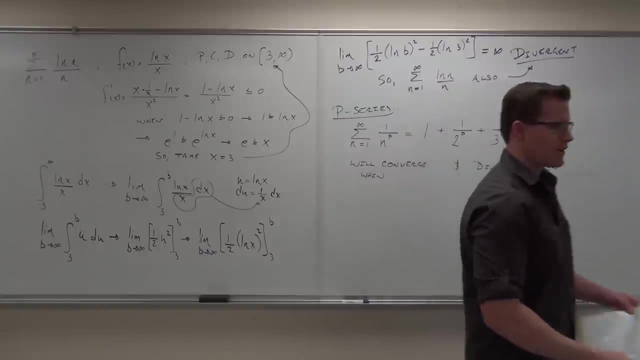 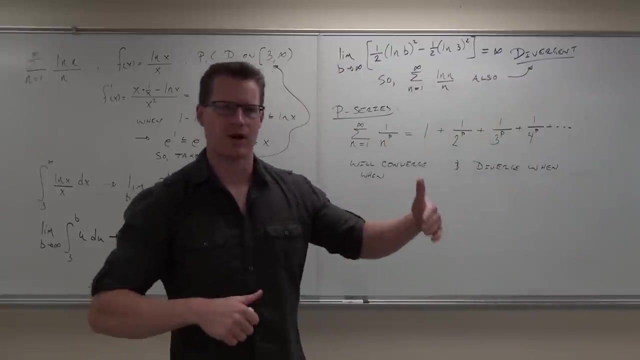 when something happens, And it will diverge. when something happens, It's not gonna be based on the n this time because n's gonna go through its sequence of numbers One, One, two, three, four, five, six, seven, eight, nine. 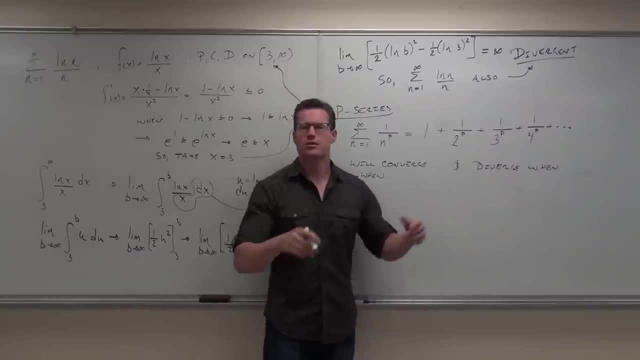 It's gonna be based on the p, So can you tell me? let's talk about the divergence first. Can you tell me when this series would diverge? What do you think When p is negative? When p is negative, You're right. when p is negative? 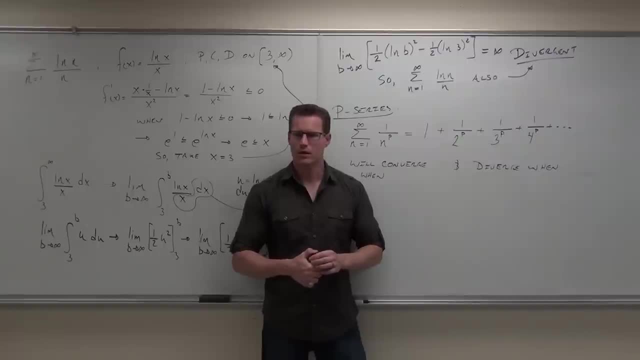 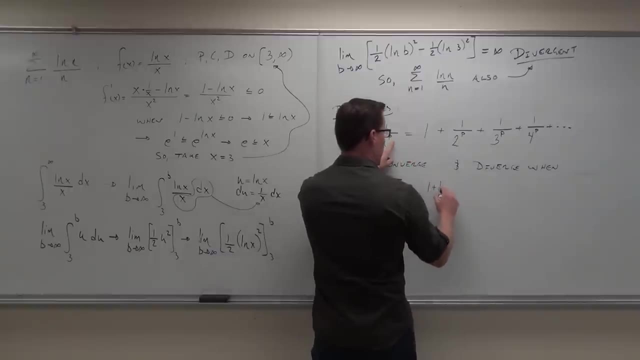 There's also one more thing: When one is zero, What about one One? Now, listen carefully, If p is one, if p is one, we would get one plus 1 1⁄2.. You know, I'll write it over here. 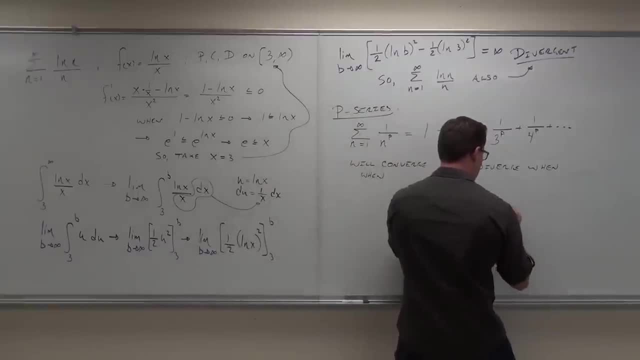 1: 1.. When p is one, we would get one plus 1 1⁄2 plus 1 1⁄3 plus 1 1⁄4.. Are you seeing where these numbers come from? Yeah, Tell me what series that is. 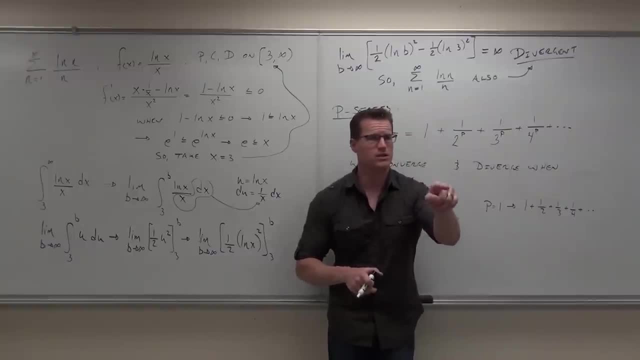 You should know Harmonic, That's harmonic series- very good. Is the harmonic series convergent or divergent? Divergent- Very good. So what we know is that it's not only negatives, but it's actually anything less than one. 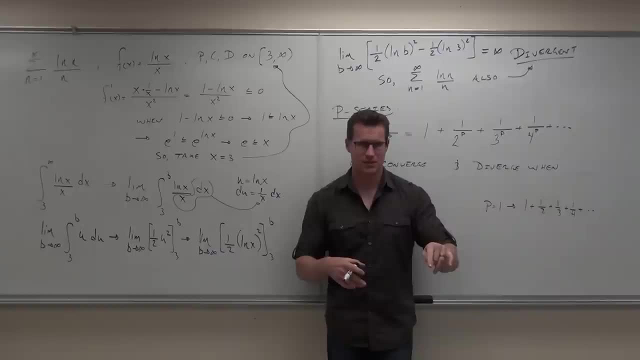 Anything less than or including one. Does that make sense to you? No, It's a harmonic series. So when p equals one, it's divergent If p is less than one. if p is less than one, well, the divergence test will actually show that to you. 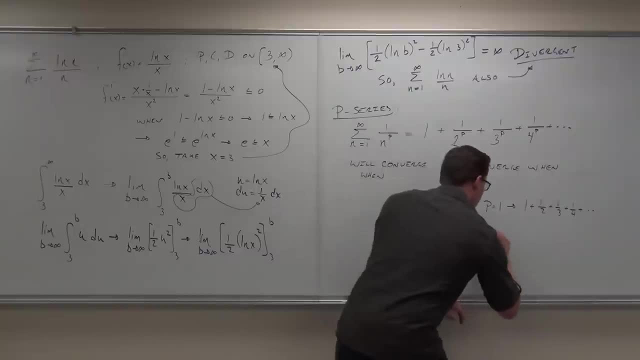 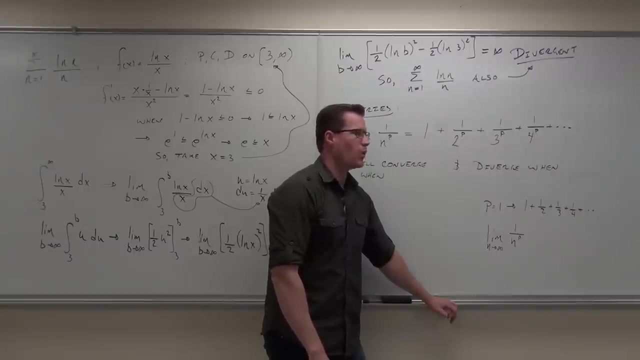 If p is less than one, imagine this. This is actually a word for both. but if you take a limit of one over n to the p, as n approaches infinity, If you do that and p is less than one, we're gonna get something. 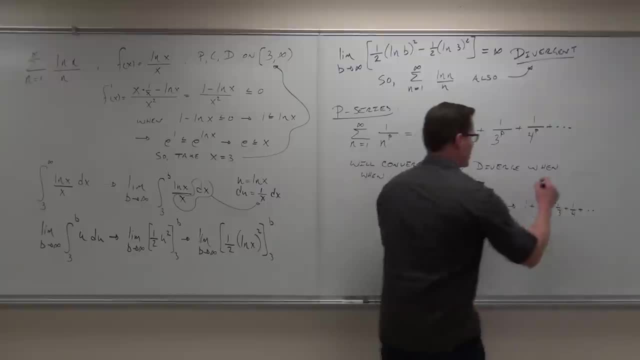 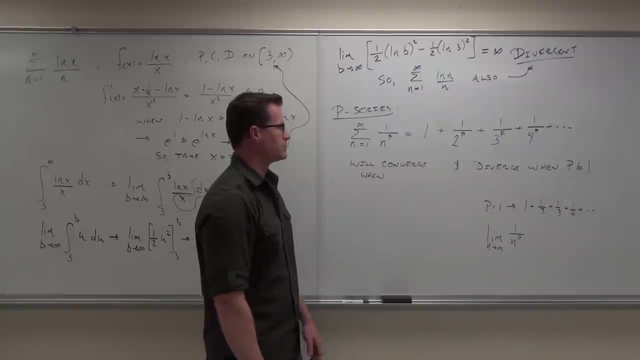 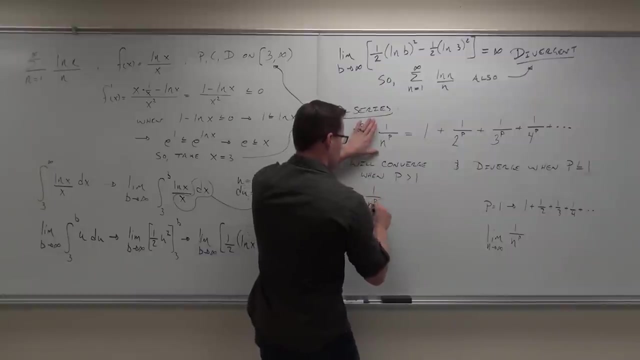 It's divergent for sure. Now, when will this converge? when p is greater than one, When p is greater than one, you can think about this: If p is greater than one, then one is greater than one. If p is one over n to the p, 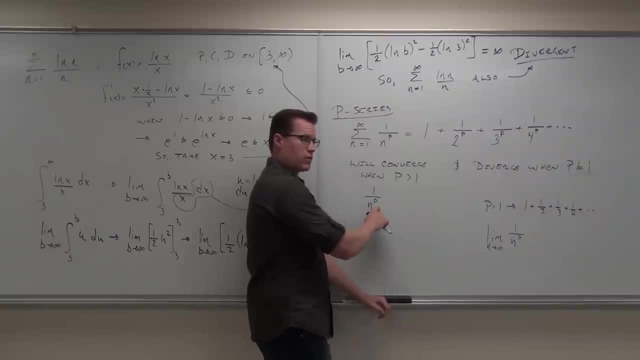 if you model this with a function, if p is greater than one, this is positive. Yes, Any positive number raised to any power is going to be positive. This is continuous. n is never zero. It's also decreasing On the interval one to infinity. 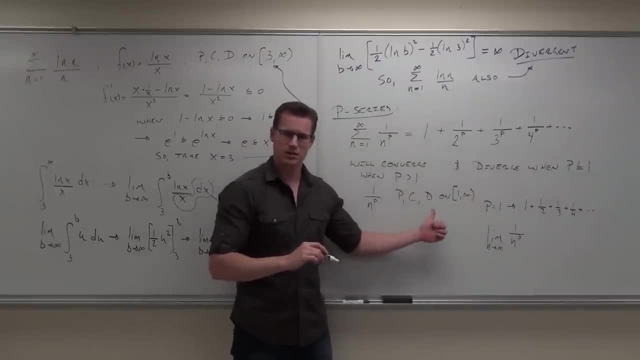 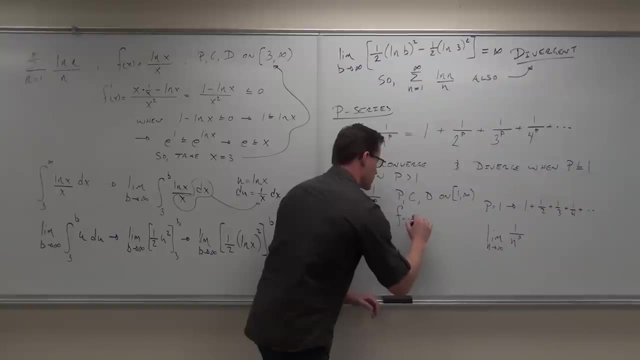 Because this will give you positive, continuous and decreasing. Basically, I'm kind of skipping a step here. okay, You model this on the function of x to the p. F equals x to the p. This would be positive, continuous and decreasing. 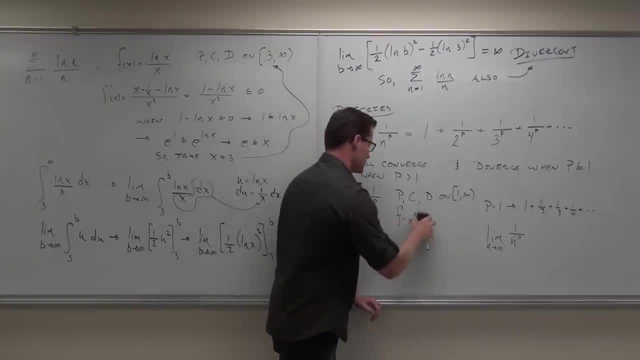 If that's the case- sorry, I'm gonna go faster than I really should- We model this on: f of x equals one over x to the p, and if we did that, this is positive. This is continuous. This is decreasing. 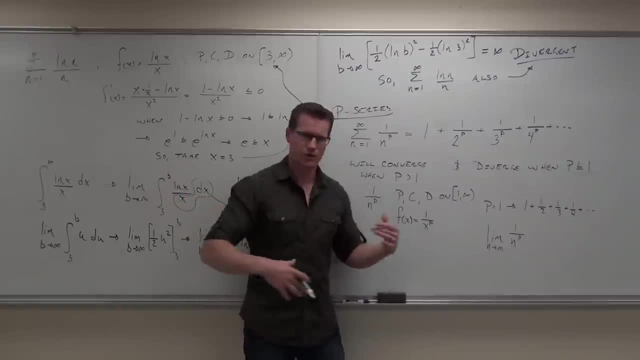 Therefore, by the integral test also- all the integral of this thing's always gonna be- we're gonna find something that converges. The integral test is gonna tell us this is also convergent, So because of this. So here's the thing. one more time. 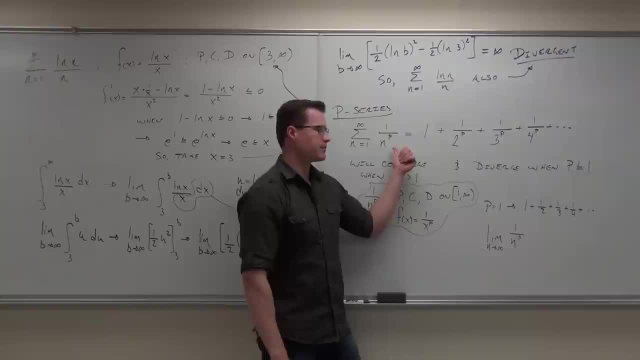 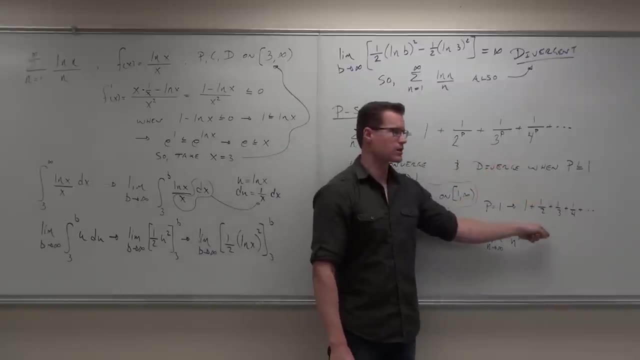 If you have your p as less than or equal to one. if you have your p as less than or equal to one, what do you know about your p? Harmonic series, Harmonic series, Harmonic series or anything lower than that, for how it's gonna diverge. 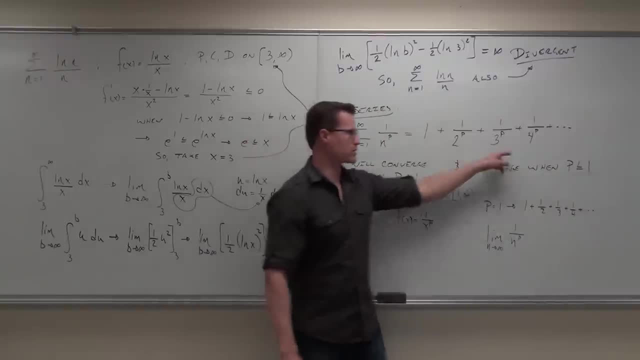 If you have your p greater than one, not equal to one, one's over here, okay. If you have your p greater than one, what do you know about it? Convergence: It's got to, Because any sort of a function like this. 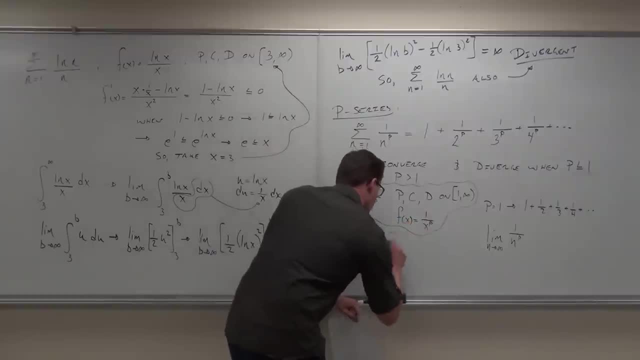 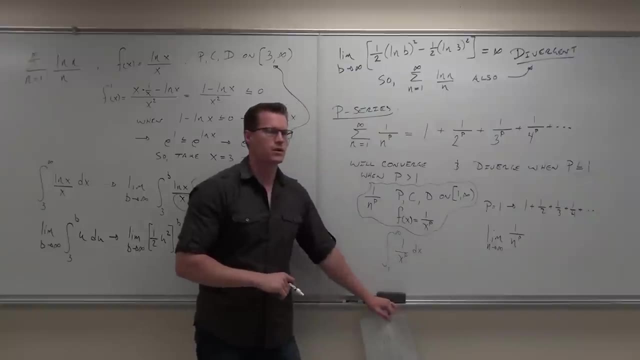 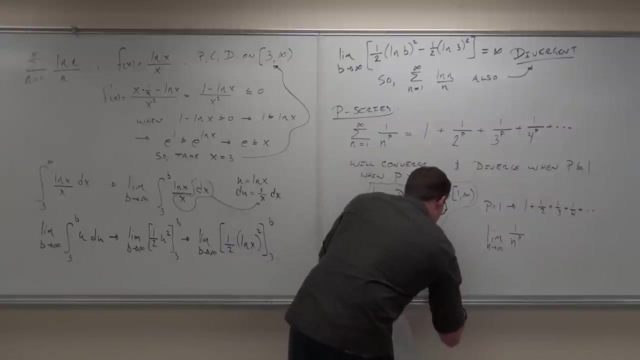 where p is more than one, your integral, from one to infinity, of one, over x to the p, dx, it's gonna converge. You can do the limit on that if you want to. You do a limit From, You do a limit of whatever your. 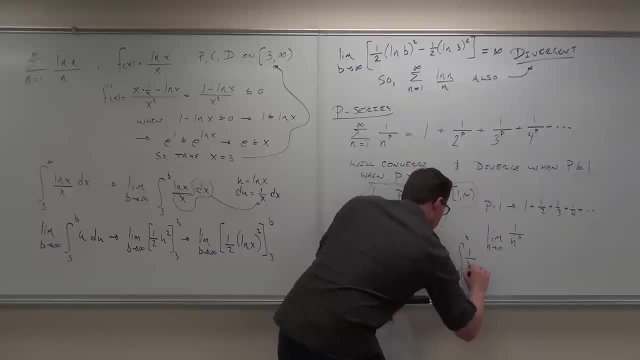 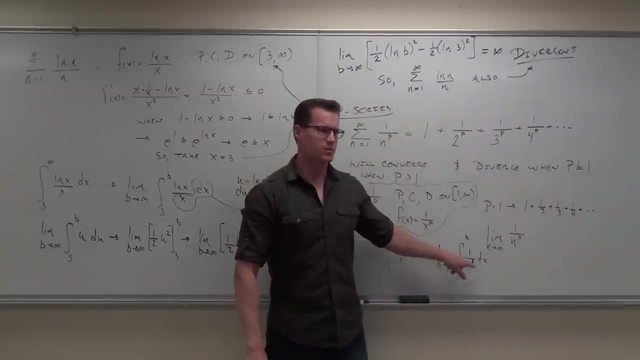 integral says: from one to the p, one over x to the p, dx. If p is greater than one, this becomes a pretty easy integral to do. This would be like x to the negative two or x to the negative three or x to the negative four. are you with me on this one? 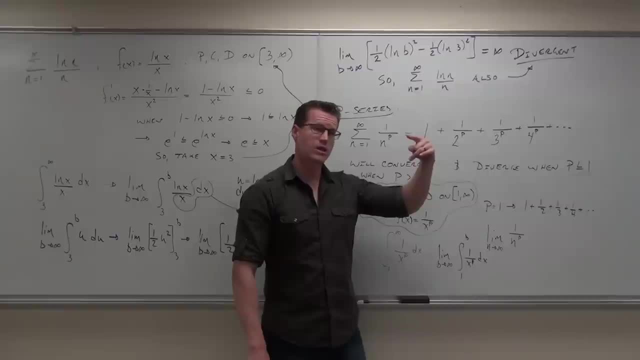 Whatever's gonna happen is you would add one to your power. that would give you at most x to the negative one. if you add one to your power, does that make sense to you? Because you'd have at least x to the second there? Well, that's not quite true. 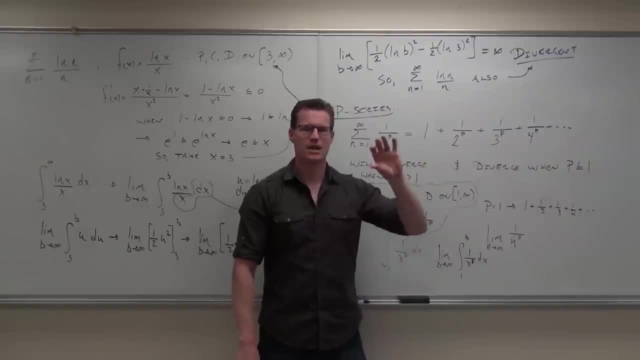 you could do this with decimals as well, But you'd have something that would still be a negative exponent. does that make sense? That would be one over infinity. when you plugged in that b, One over infinity gives you that zero plus whatever constant you have. 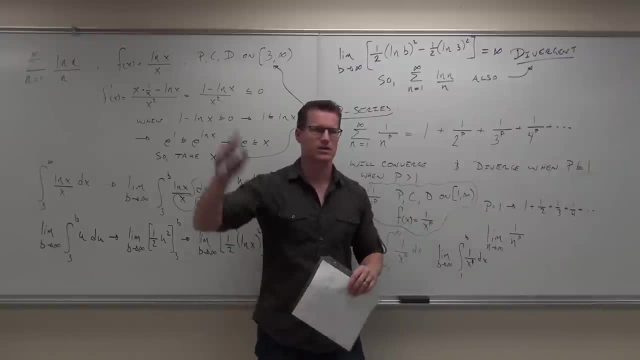 that's gonna be convergent. So we have something that is convergent here. Show of hands if that made sense to you. Okay, so p series divergent p is less than or equal to one. p series convergent p is greater than one. 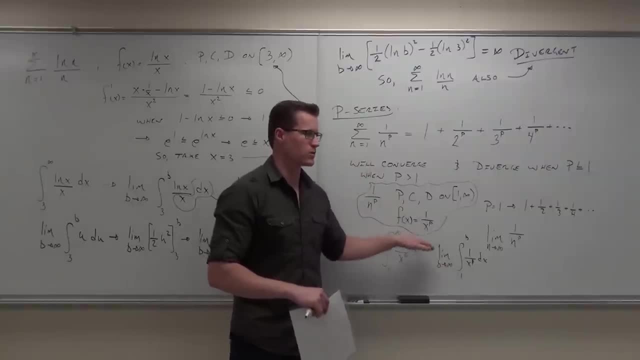 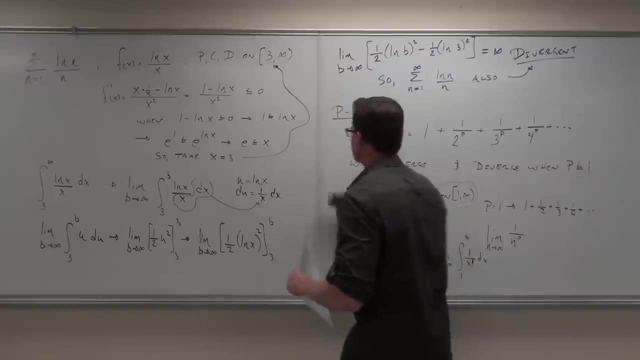 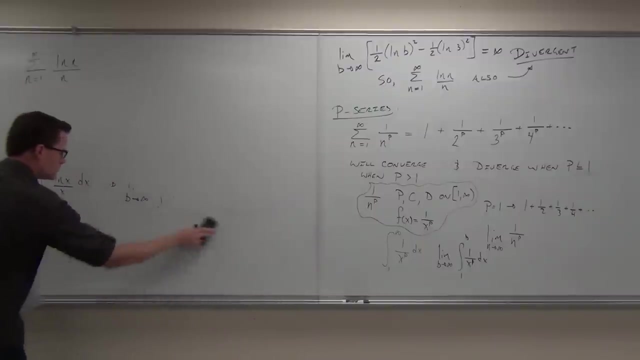 by our integral test, and you can do this in general when p is greater than one. Now let me show you how this works and how nice this is. Trust me, you're gonna like this. Here's why you're gonna like it. 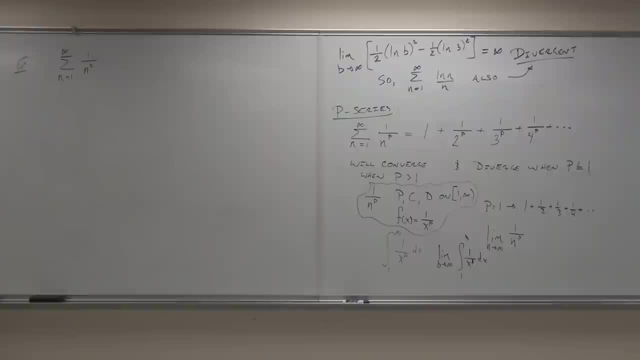 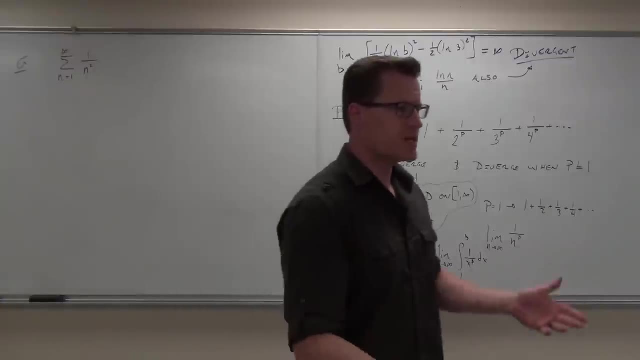 I want you to consider that series. Firstly, is that a specific type of series that you know? Yes, Yeah, is it geometric? No, it's not geometric. Well, we have lots of different types of series here. Is it a p series? 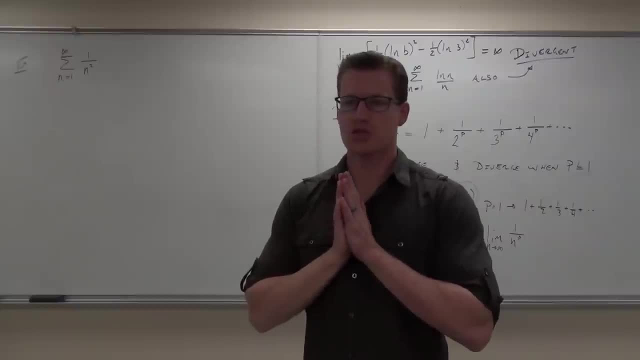 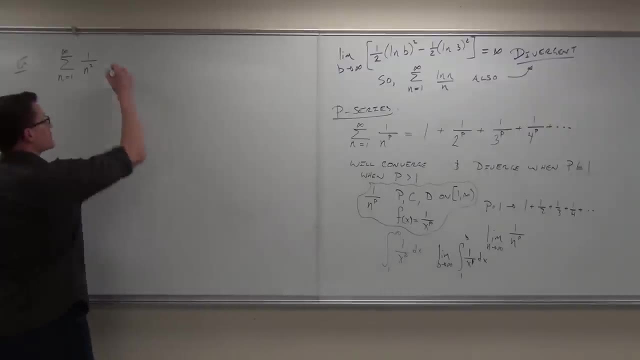 Yes, Very good. Hey, what's the p Two? Is two more than one. Yes, Tell me about the series Convergent Bam. Okay. So you have to state something like this. You say, okay, this is a p series. 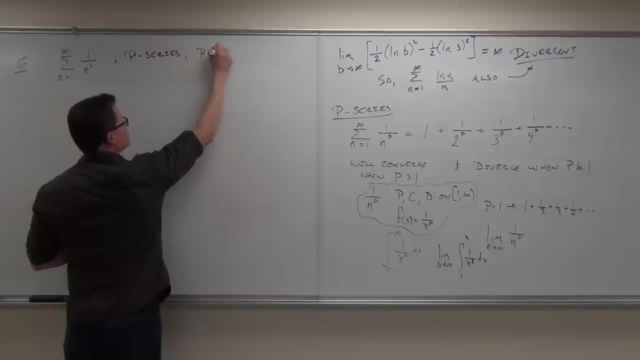 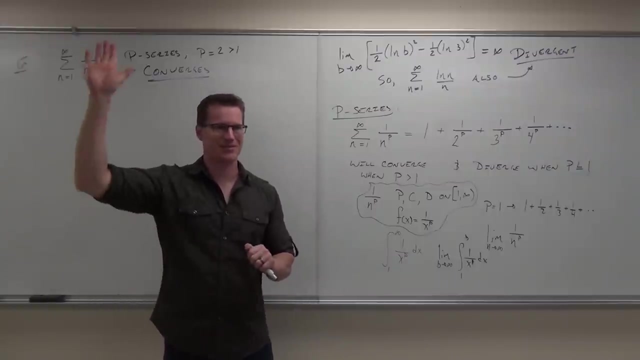 The p is two, which is greater than one. therefore, this series converges. Do I know what the sum is? No, Do I know what converges? Yep, That's what I'm asking here. Okay, Should have answered, if you like that stuff. 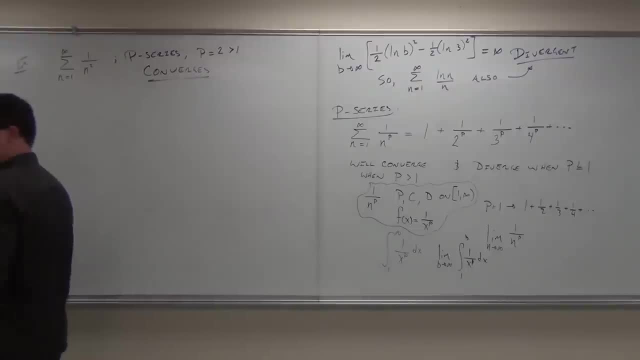 Don't you like that? Give me 30 of these on the test. huh, 100%, 100%. We'll kick some calculus in this class. Okay, What's the right answer? I don't know, I can't remember. 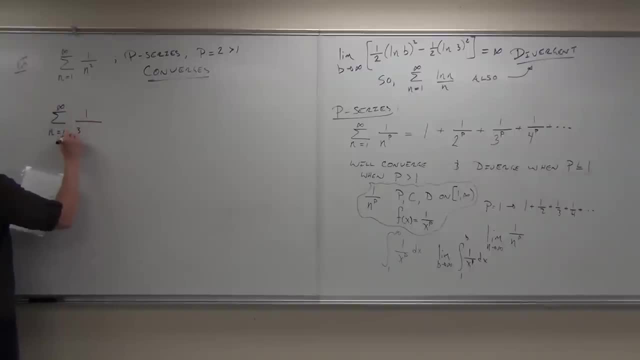 Forarten, I don't know. I'll go with that. I don't know. It's in the book, forarten, I think. What? the? What kind of lecture? A lecture series? Okay, So we got a question here. 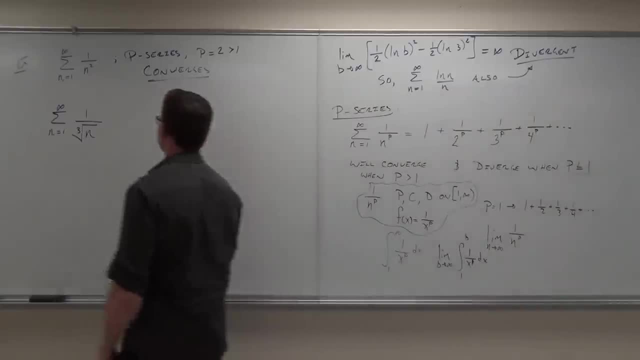 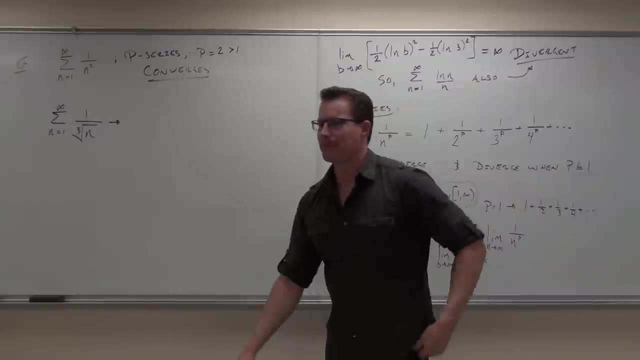 We have a question: Why does one nine, Why does one nine count? We don't know. I don't know. Why does one nine count? Now you tell me what type of series is that. It's still a p-series. 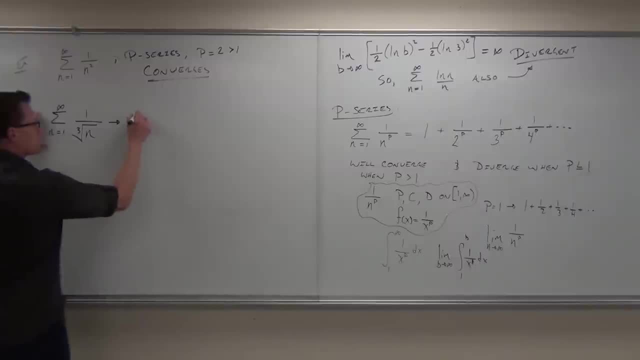 Now you might want to write it as a p-series. So how in the world is that a p-series? Well, it's a series, and it was 1 to infinity, 1 over n to the. every type of root is automatically a power. 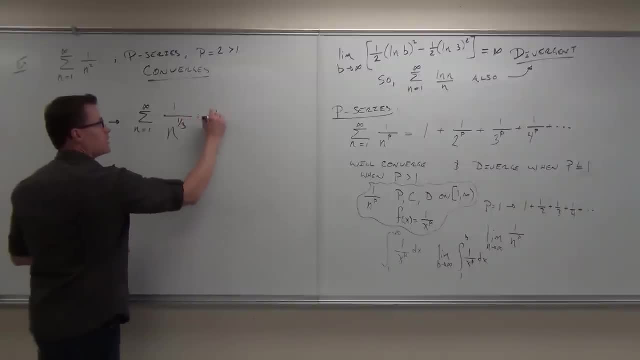 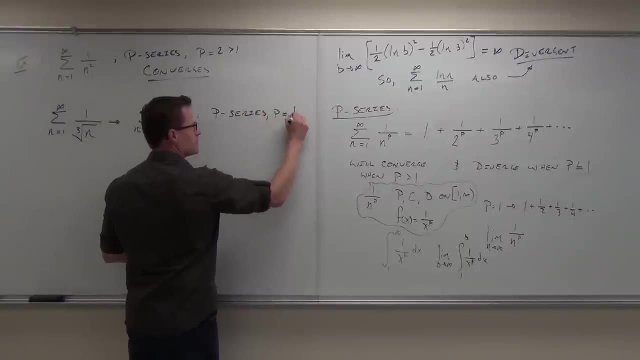 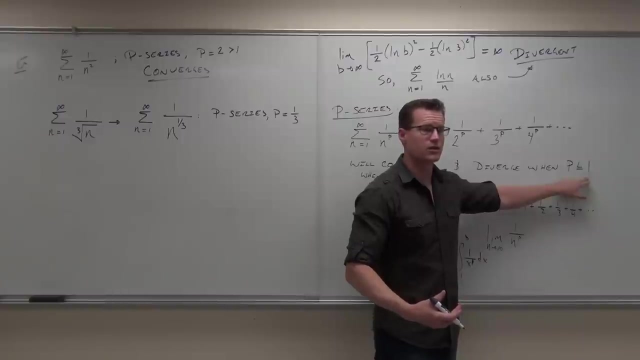 This is a power. So we say this is a p-series. p is equal to what's our p. Now remember: this is not 0.. It's not a negative, Of course. every negative p is going to give us a divergent series here. 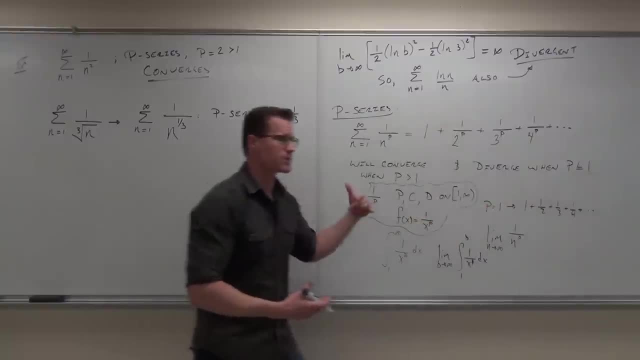 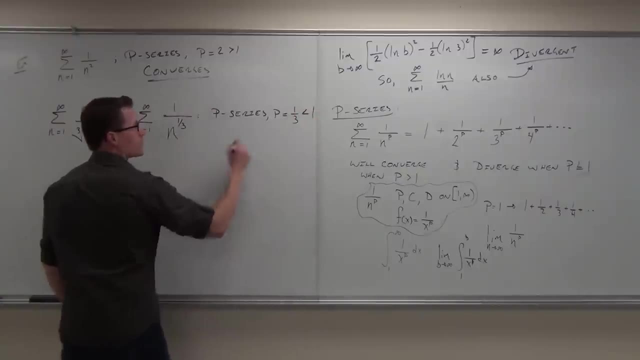 but it's not 0.. It's less than 1.. So even if we get something like 1 third, what's that tell us about our series here? This is less than 1 or equal to 1.. You can put that here. 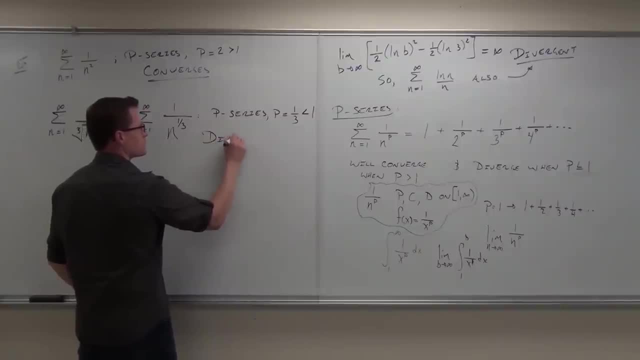 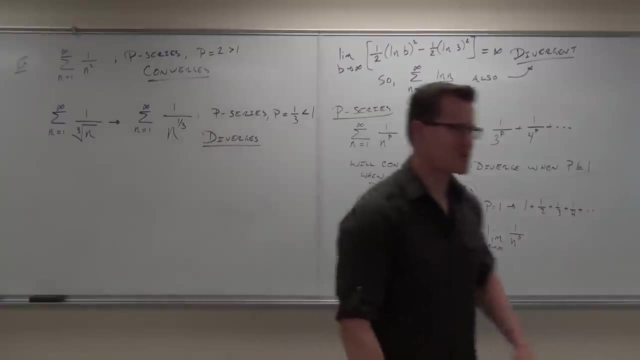 Less than or equal to 1,. therefore, this series diverges. Is it a p-series? Is this making sense to you? Yes, Got a nice little break from doing all the other stuff, right? Okay, we'll do one more. 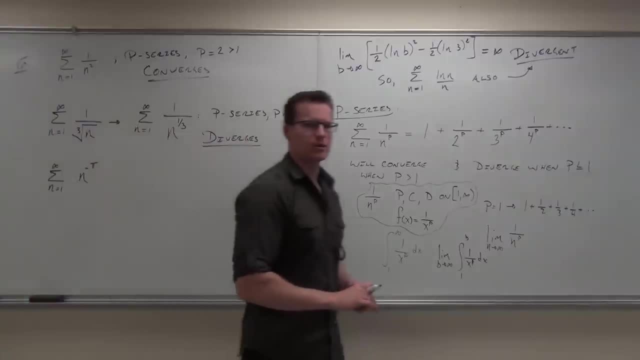 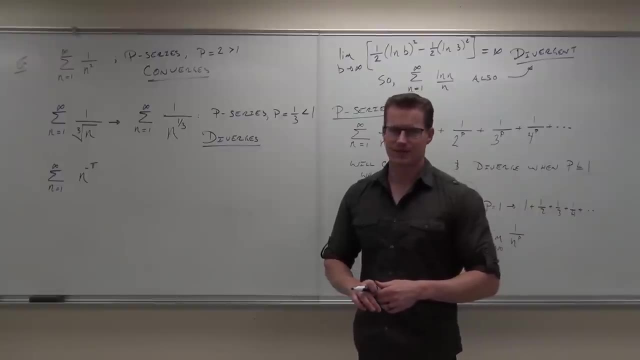 True or false. this is a p-series. True or false. False, True or false, it's a p-series. Well, wait a minute. it's not 1 over something, It's a negative power. You better be smart enough to do that right. 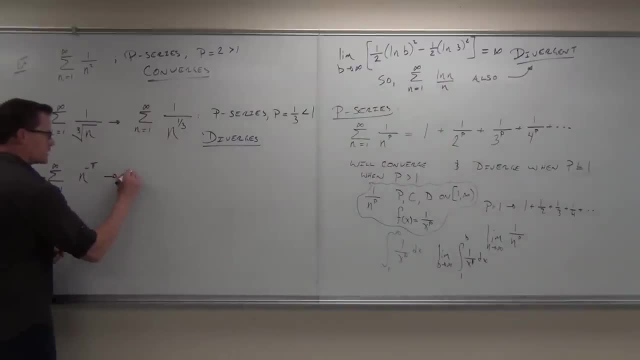 Okay. so if you have a negative power, you need to understand that this is the same thing as 1 over n to the positive pi power. That's a weird power, but I didn't say anything about p being an integer. I didn't say anything about that. 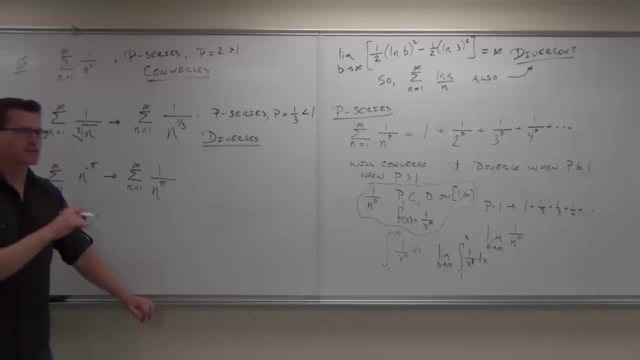 All I said was p was a power. p is an exponent. If p is less than or equal to 1, your p-series diverges. If p is more than 1, your p-series converges. So is this a p-series? 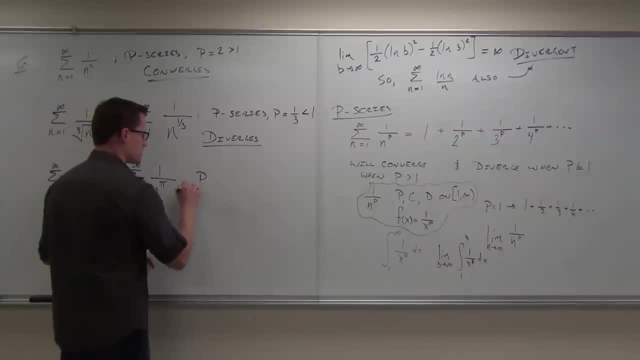 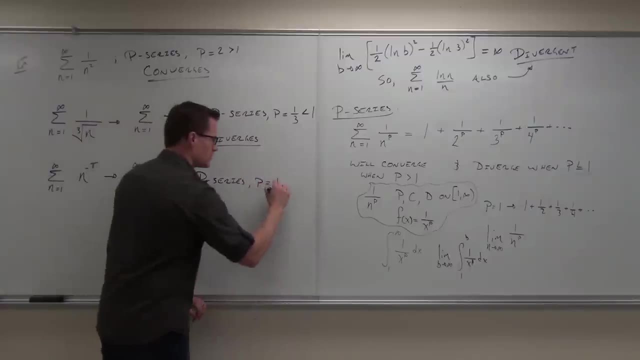 Yes, Yes, it is. You might want to write it as such. So it's a p-series. Okay, The p is what's the p? Pi? Pi 1, 4.. Yeah, pi is about 3.1415926 something, whatever. 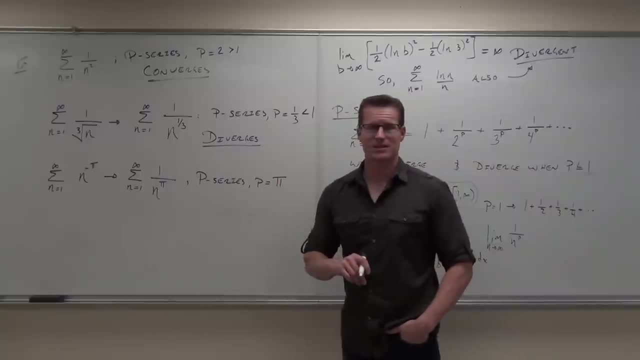 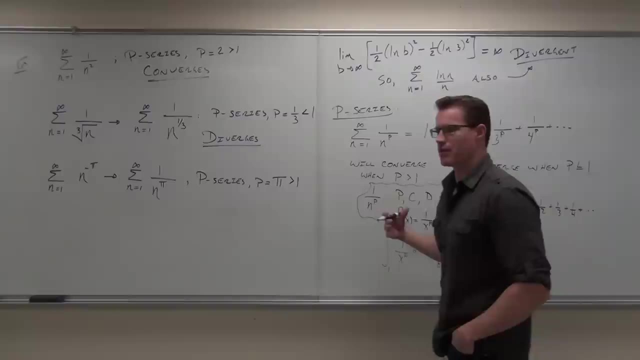 I don't know the rest of them, But what I'm asking is: is that bigger than 1, or is that less than 1?? Bigger than 1.. That's more than 1.. So what does our p-series say about that? 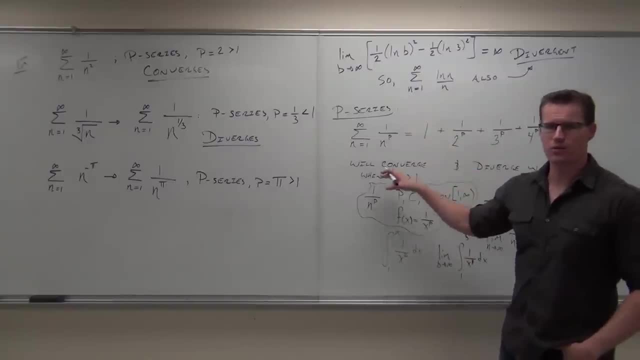 Because we've done this in general for p is anything bigger than 1, we can say that all the time. We don't have to reinvent the wheel and prove it every time. We know that if p is less than or equal to 1,. 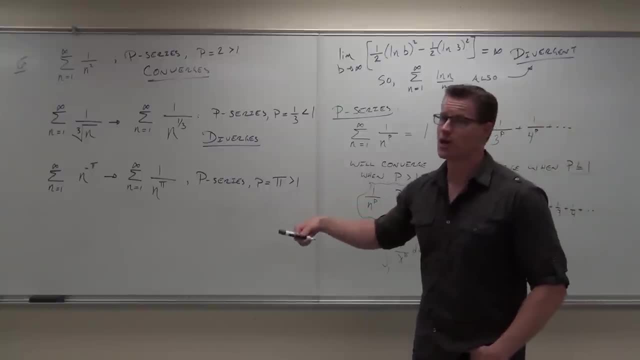 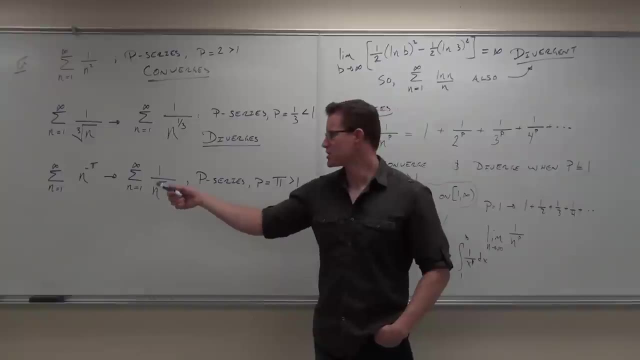 that series is going to diverge. If p is more than 1, that series is going to converge. You better make darn sure that it actually is a p-series though. okay, So spend some time and really think about it, But if it is, goodness gracious, isn't that nice. 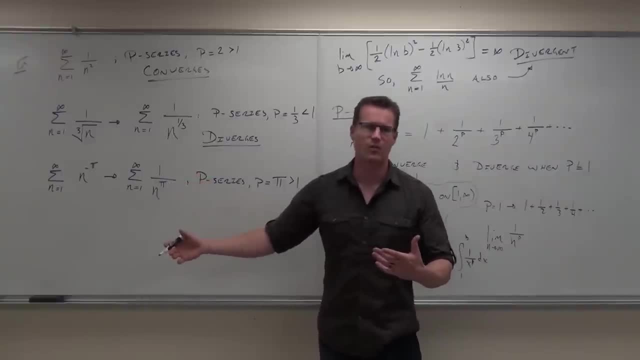 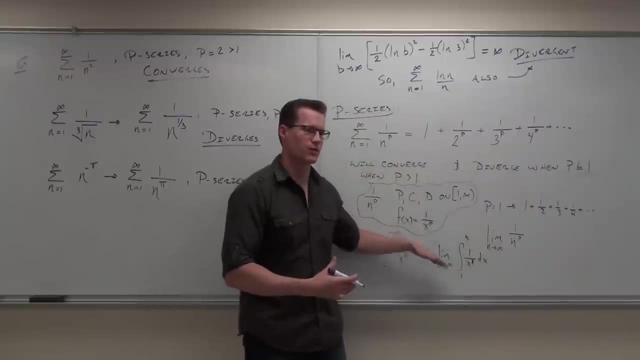 So if you don't recognize the p-series, you have a lot more work that you're going to have to do. right, You do the integral test with this when you don't actually have to. We've done the integral test basically once and for all for this. 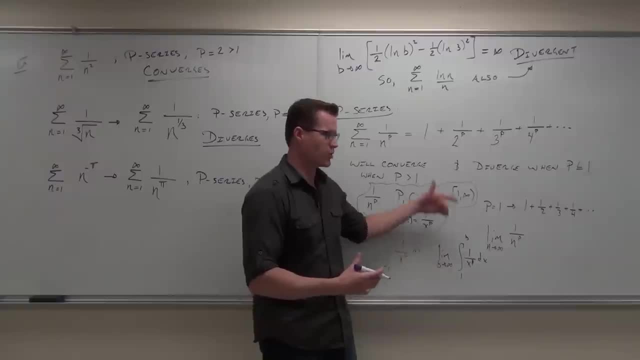 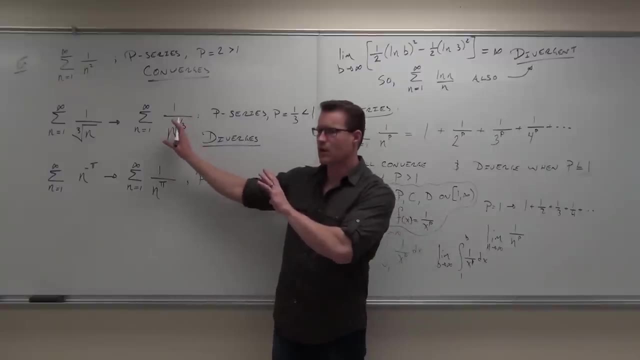 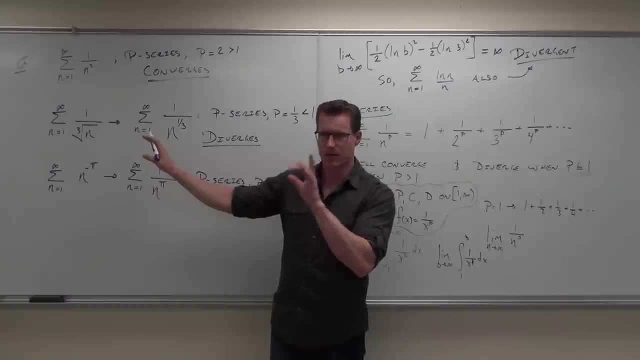 That's all it is. If you have any power, listen, listen. If you have any power, that's less than 1, any power less than like 1 third. what happens is that this is this would become x to the negative 1 third power correct. 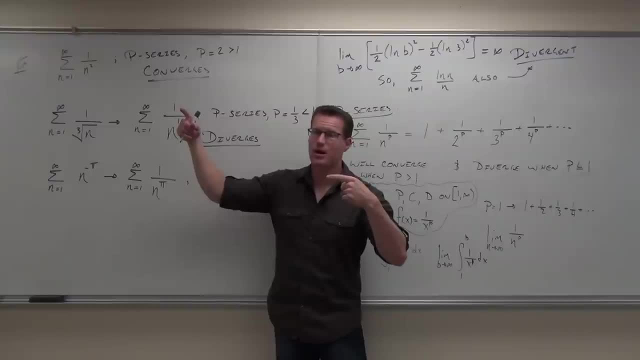 You would add 1 to it on an integral. That would become positive, negative, 2 thirds power. When I let b approach infinity, that is going to approach infinity, That series is going, that limit's going to diverge. It means my integral diverges. 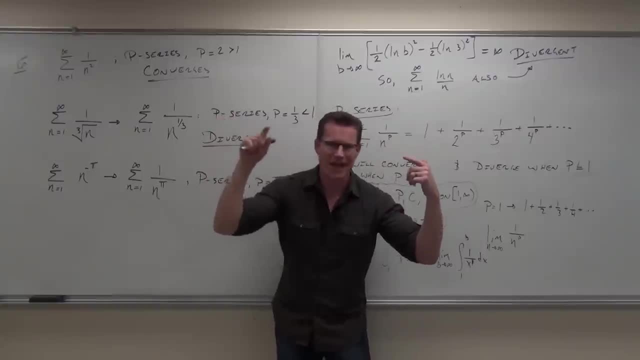 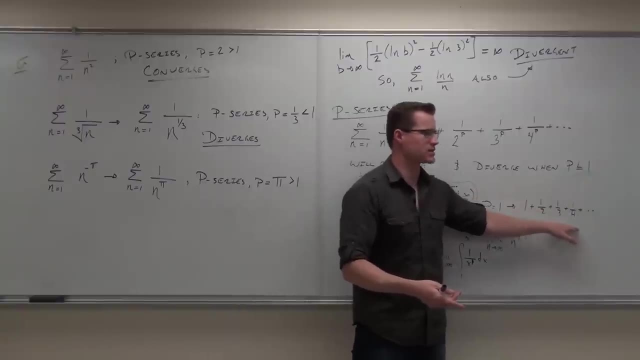 That means my series diverges. Does that make sense to you? That happens any time your p is less than or equal to 1.. If it equals 1, you've got l and x. We already determined that. well, this harmonic series diverges. 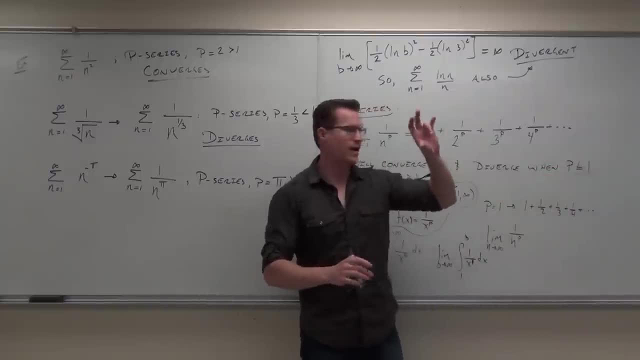 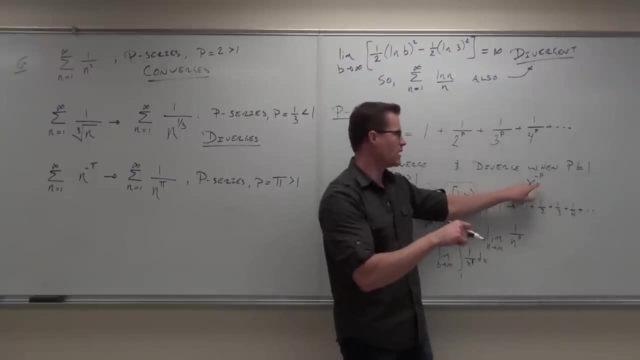 so that takes care of the equal to 1.. Anything less than 1, I'd have x to a negative p power. If p is less than 1, when I add 1 to it, x gets to a positive power. Does that make sense? 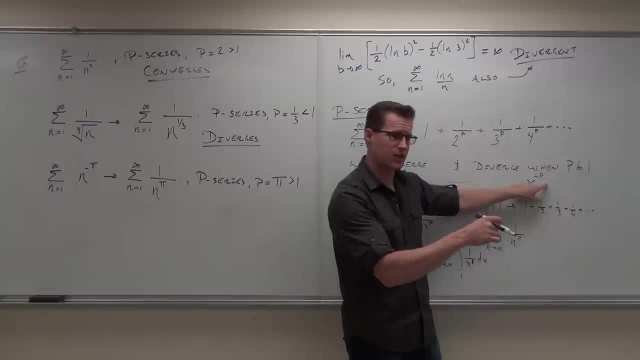 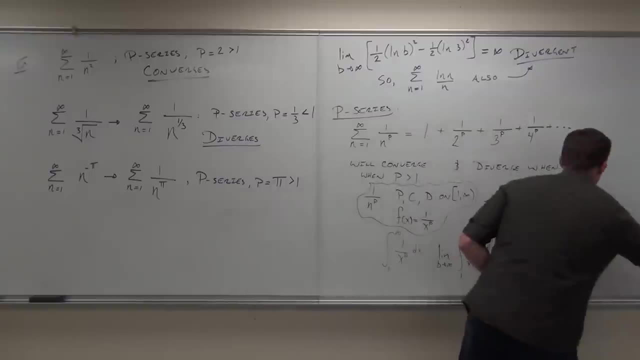 What that means is that when I evaluate my limit as b approaches infinity, that thing's going to go to infinity. That's why, any time p is less than or equal to 1, I get a series that diverges. The opposite is true for convergence. 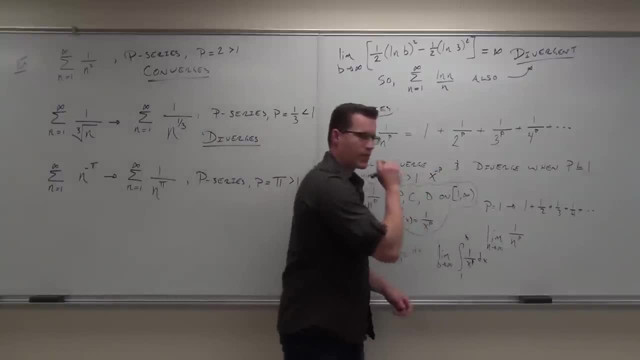 If p is more than 1, I would add x to the negative p, correct. But if p is more than 1, when I add 1 to it the power is still negative. That means I have 1 over x to some power. 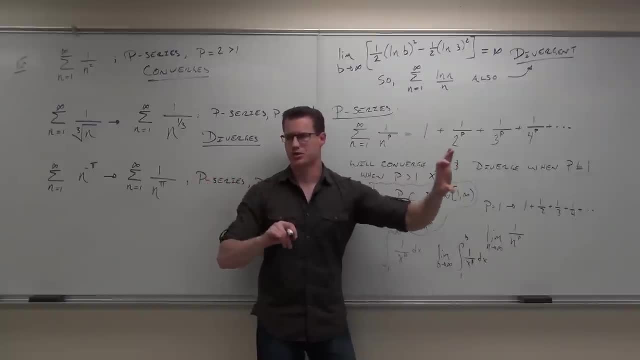 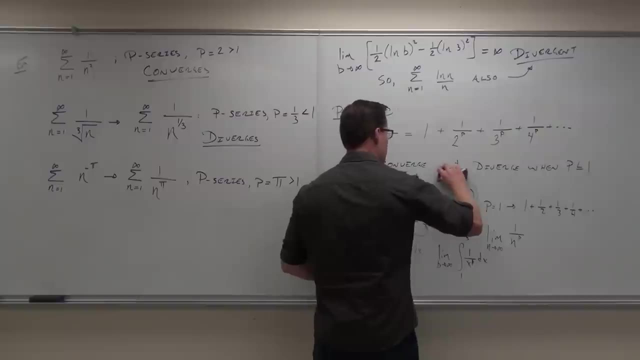 I don't care what it is. When b approaches infinity, that's going to approach 0. Make sense. Then I'd have a constant or something. Therefore my integral would converge. That's the whole idea. So don't be doing integral test, all this stuff. 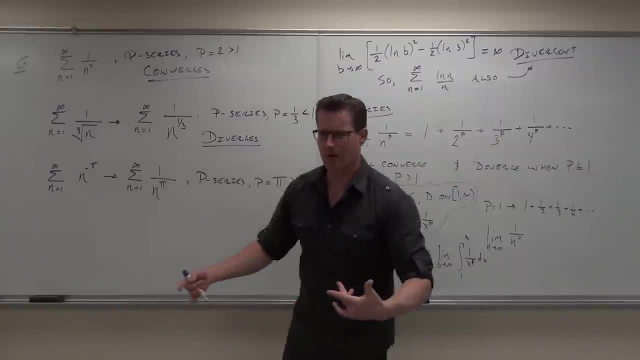 It for sure would work absolutely, But we've only done it like once and for all here, so don't reinvent the wheel. That's the whole point. Show of hands. if you understand the problem, Good deal. Tell you what. we're not going to do any more p series. 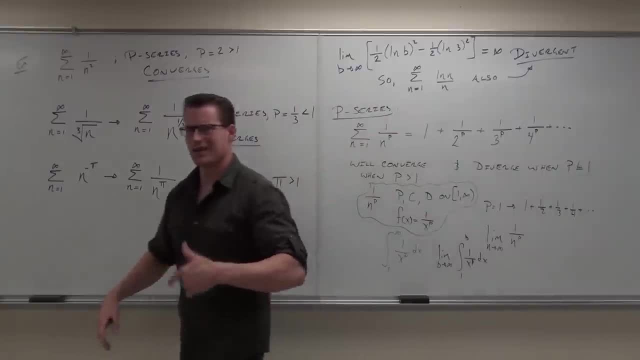 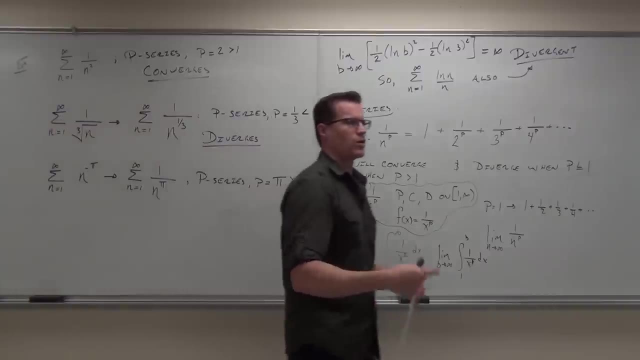 This is hopefully straightforward to you. I want to do one more kind of a little bit more advanced idea of a series: show you what you can and can't do with it. Basically deal with a little bit more with how to show decreasing. 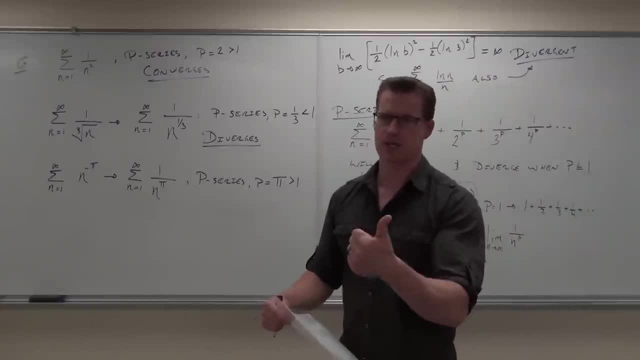 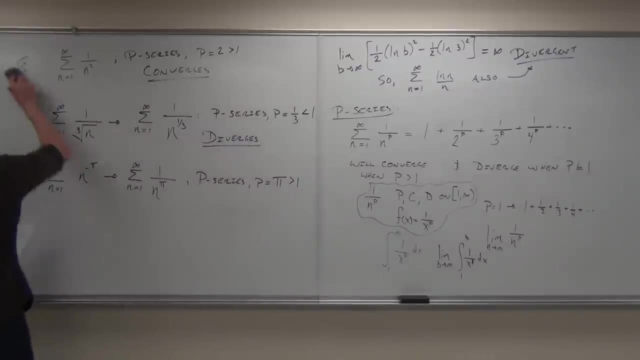 Because the whole integral test says you've got to have something that's positive, You've got to have something that's continuous and you have to have something that's decreasing. So I want to go through one more of those and then we'll call it good on this section. 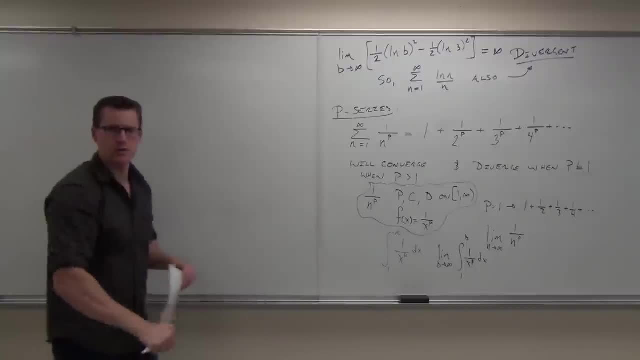 Do you guys have any questions on the p series at all that I can answer for you? Yes, Just the only qualification for it that your variable has to be in your denominator. just to any power. It can't be added to anything, right. 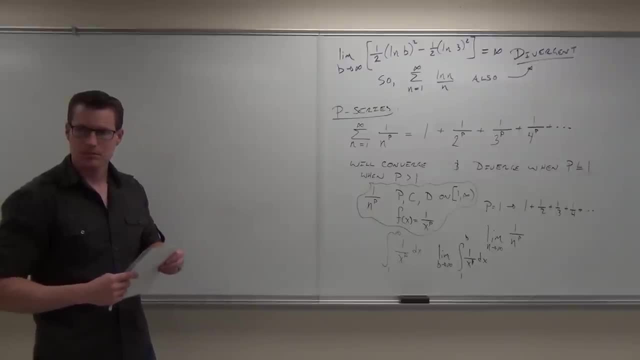 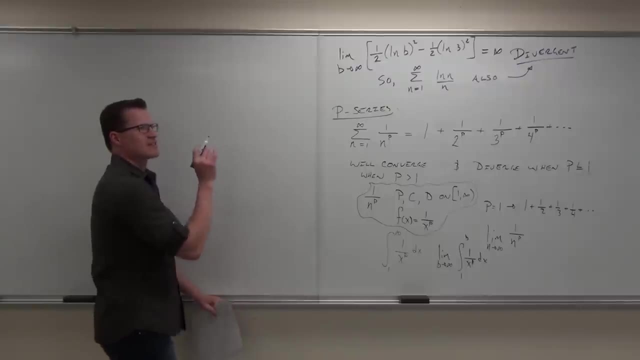 It just has to be variable to a power. Then you can use p series in your denominator. I didn't quite catch that. All right for p series. yeah, your variable. Give me an example. Let's just say 1 over what? 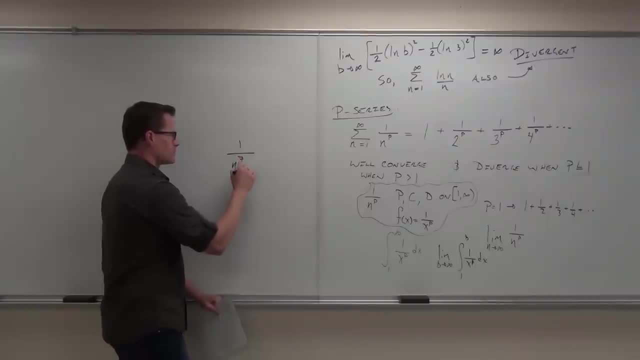 Let's just say 1 over n to the 7th plus 1.. You couldn't use p series on that Like that. Yeah, No, It just has to be the. But in the next section we're going to cheat. 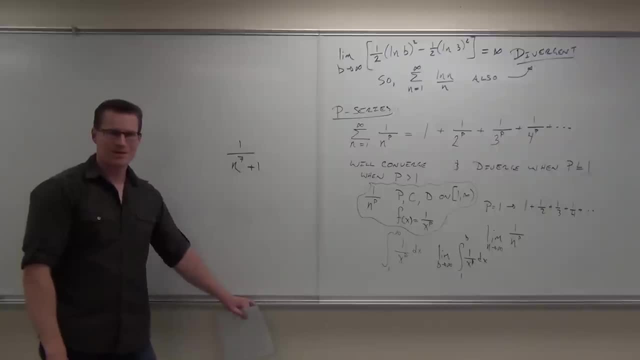 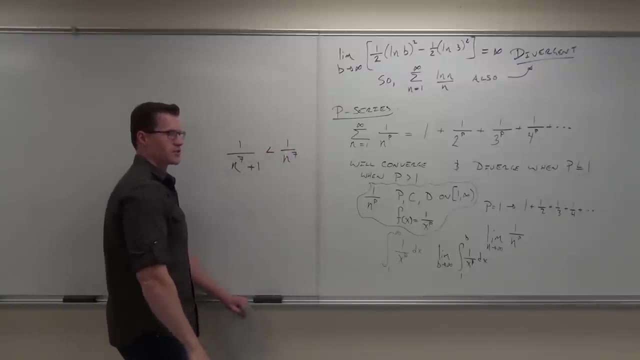 a little bit and do it. Oh, all right, cool, You want to see it. Yeah, sure, Is this for sure. less than 1 over n to the 7th? It sure is. Yeah, Does that converge p series if this is always less than that one? 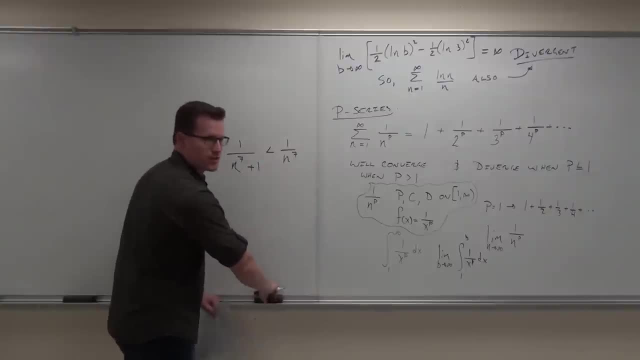 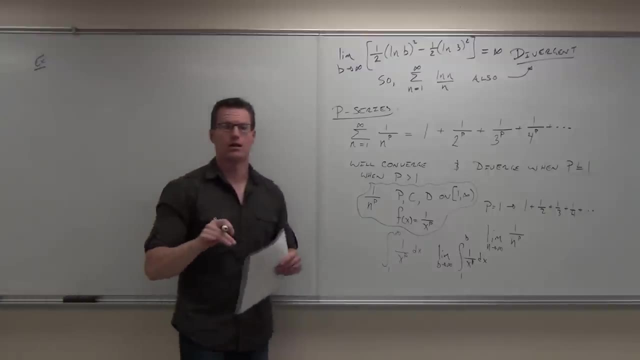 tell me something about this one. No, It converges. Comparison test. That's the next section Now. so yes, we are going to use the p series a lot- okie dokie a lot- But we're going to normally do it. 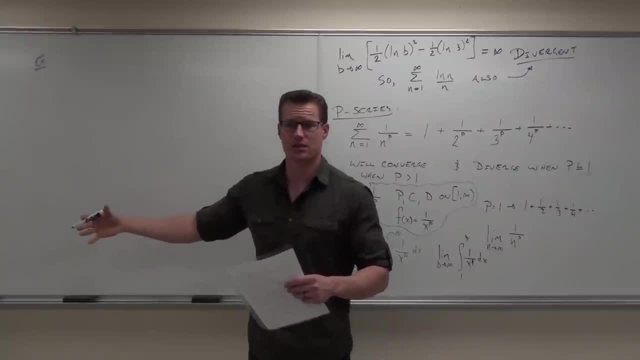 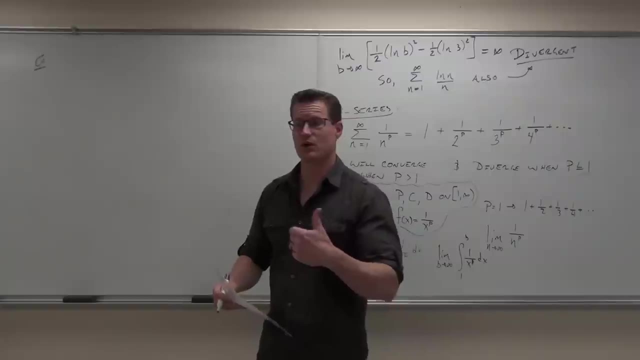 It's not as easy as what I gave it to you. We're going to normally do it as a comparison test. We're going to base our other series on something we already know about. We're going to base them on geometric series. We're going to base them on p series. 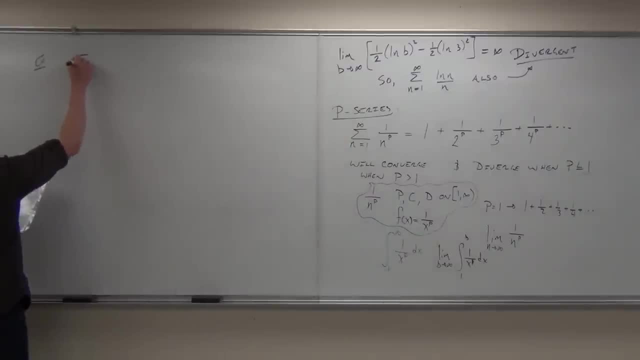 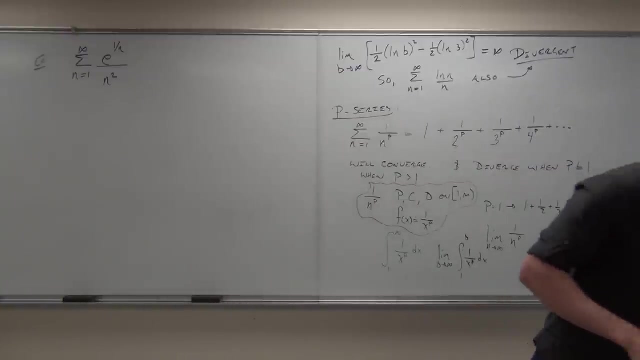 We're going to compare them to. I'll show you how to do that, But first I want to do this example. OK, Here's how we would go through this. I kind of did this for integrals for you, so I'll kind of show you how to do this for series as well. the thought process: 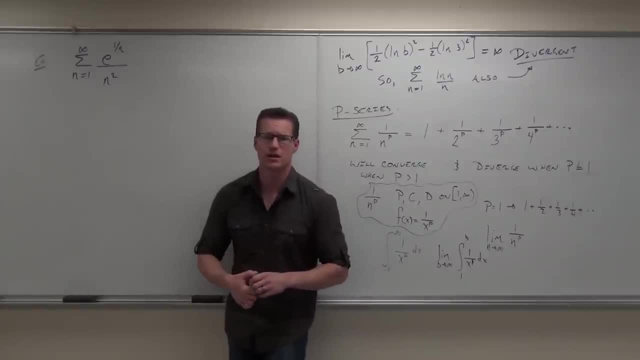 The thought process is: the first thing you check for is the divergence test. That would be the first thing you check for In this case. the divergence test is going to show you- because you do a couple well- L'Hopital's rules there. 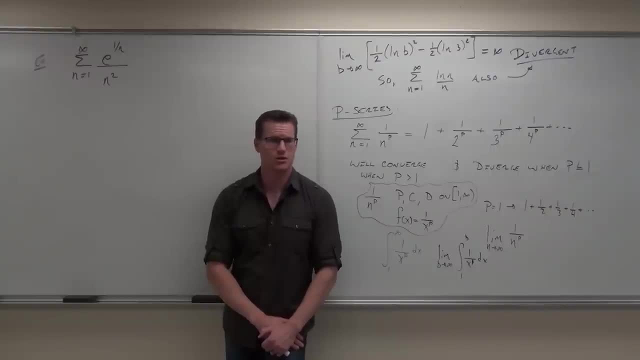 you're going to get a 0 out of that thing. Your divergence test tells you 0.. What's divergence test say? If it's not 0, what happens? It's divergent If it is 0, what's it say? 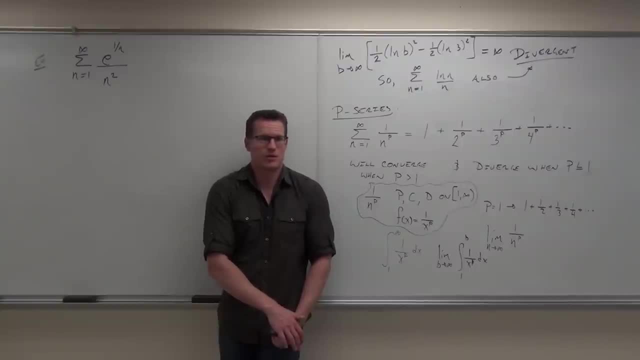 Divergent, Maybe not divergent, Don't know. Undetermined. We've got to figure this thing out. OK, So for us, we already determined that Next thing you check for is this a simple series? Is this a geometric? 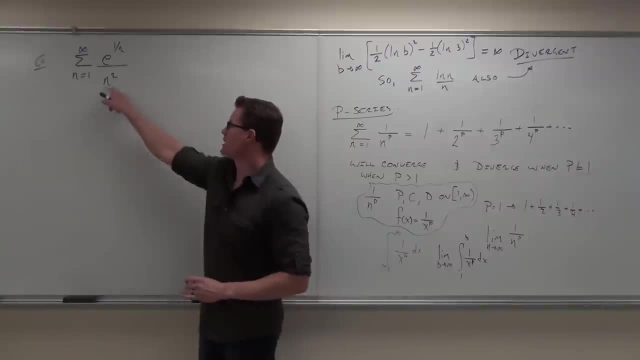 No, It's not. Here's how you tell. Is it a number raised to the n under a number raised to the n? No, No, It's n raised to a power. That's not a geometric series. Does that make sense? 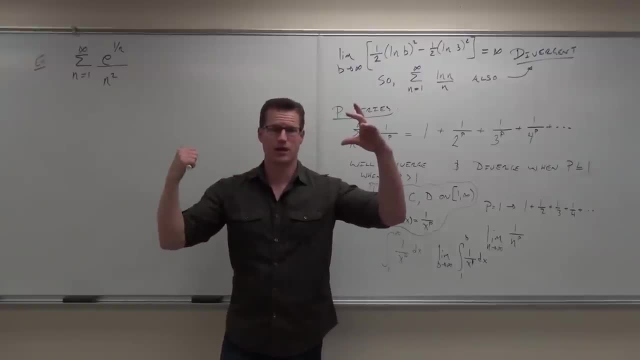 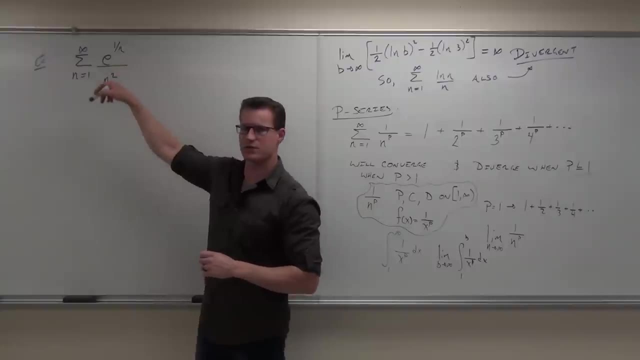 Geometric is a constant. It's a constant raised to a power. This is not that And you can't make it that. So, no, it's not geometric. Is it a p-series? No, No, It's got to be 1 over something. 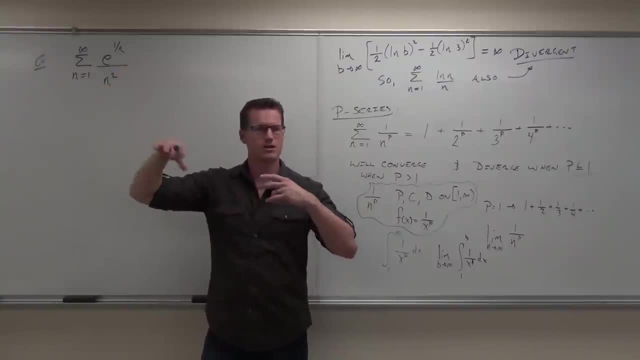 That would be a p-series there, Or a constant over something, Because a constant you can pull out, This is not a constant. Does that make sense? So divergence test. well, it is equal to 0.. So it might not be divergent. 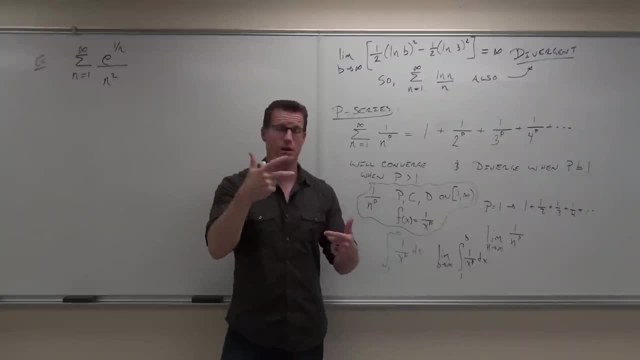 We've got to check Geometric series no, P-series no, And hopefully you just caught on how to check for that, Because I just explained it right now. So what's our last option for us right now? Well, our last option is an integral test. 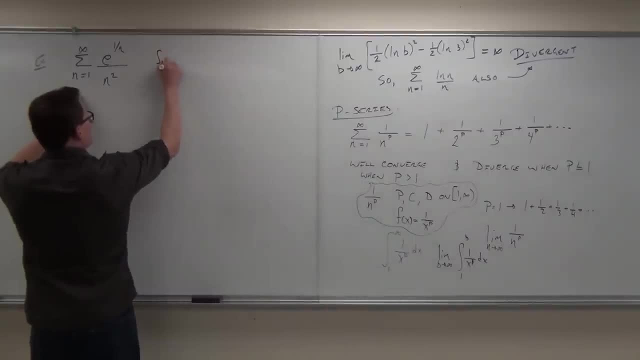 So we've got to look at this thing and pretend that we've got a function of x. actually make a function of x that models this sequence: e to the 1 over x over x squared. OK, in order for you to use an integral test. 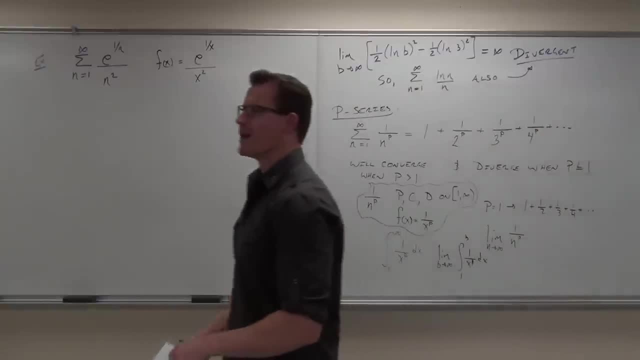 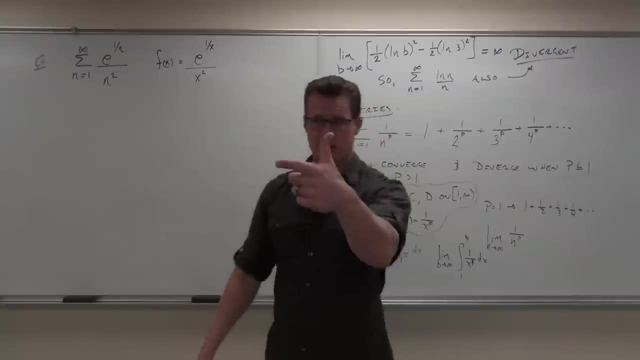 and you guys should all know this in order for you to use an integral test. what must this function be on my interval, for my series? What must it be Positive? Positive, Very good. What else? Continuous, Continuous And 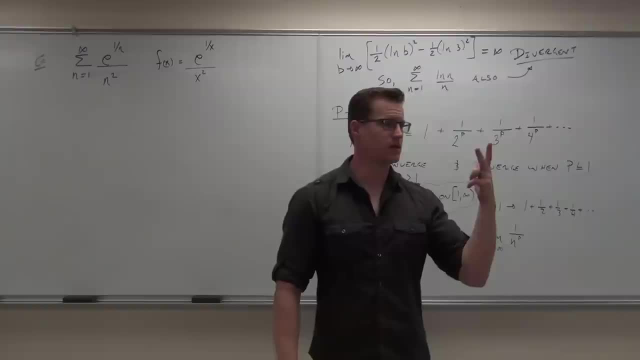 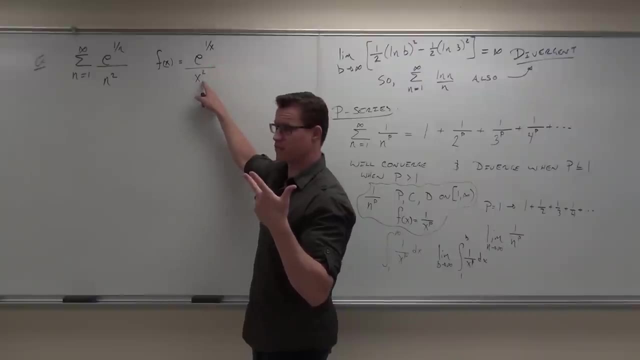 Decreasing. The hardest one to show is usually decreasing. Positive is pretty easy to show. You just go. that's always positive because it's e to some power. That's always positive because it's squared. A positive over a positive is a positive. 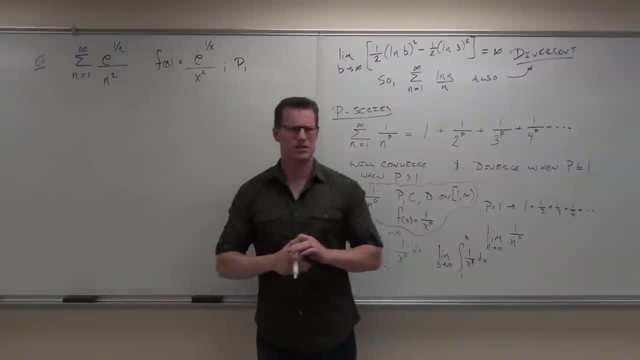 It's definitely positive. Does that make sense to you? Continuity- Continuity is usually pretty easy to show. This is only discontinuous at 0.. That's it. e is continuous everywhere. e to the power is always continuous. How about x squared? 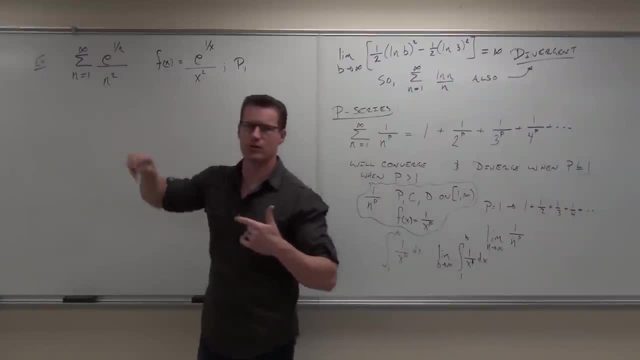 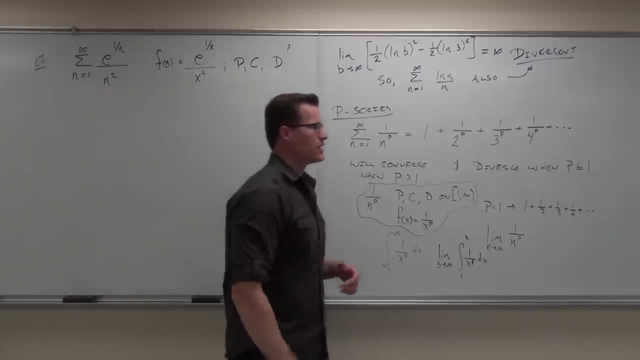 Well, it's always continuous, except at 0.. Do we ever hit 0 in our interval? No, It's always continuous. The hard one here is decreasing, Decreasing. you go. I don't know How do you show decreasing for a function? 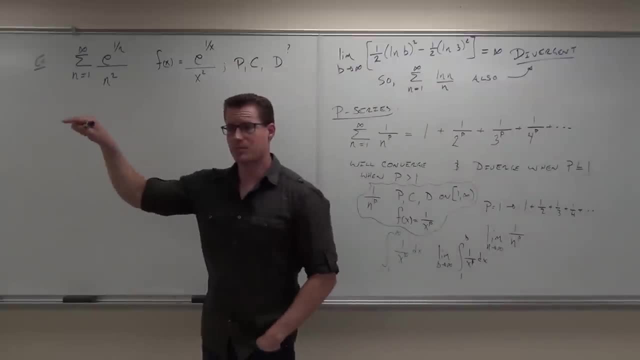 You've got to do one of two things: You've got to show that a sub n plus 1 is less than a sub n, which is sometimes very hard to do, Or you take a derivative, if it's something that you can take a derivative of. 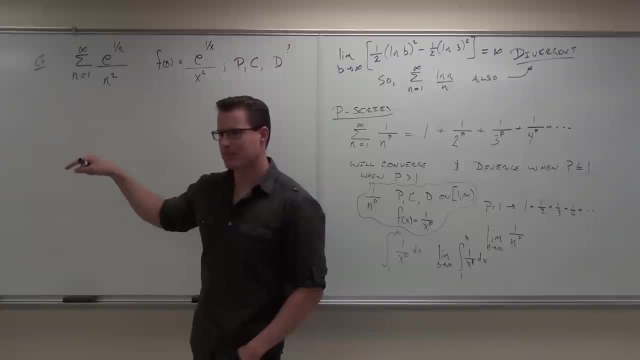 That's probably the easy way If you have n factorials and things. do you know how to take a derivative of a factorial? No, So you'd have to show that a sub n plus 1 is less than a sub n and go for it that way. 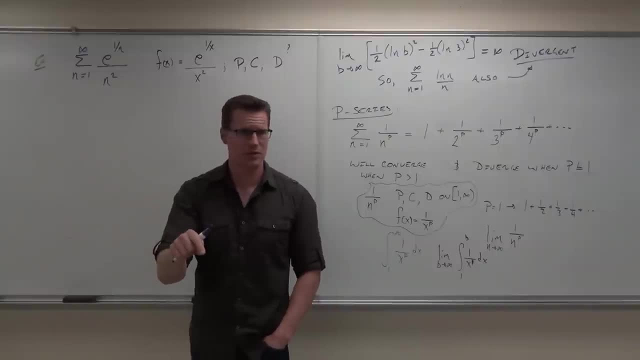 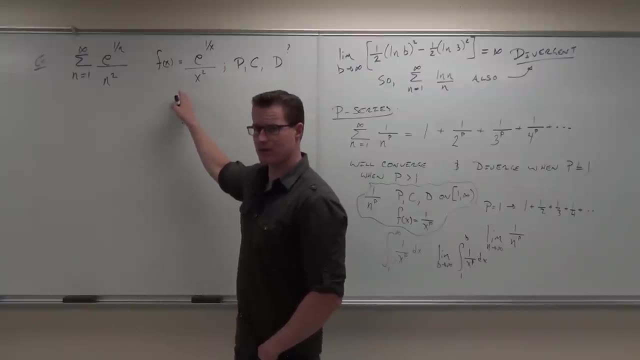 Show that it's decreasing. We did that once, if you remember. Do you remember that with sequences? We did it In this case because I don't have any factorials. I have nothing horrible going on and I can take a derivative of this. 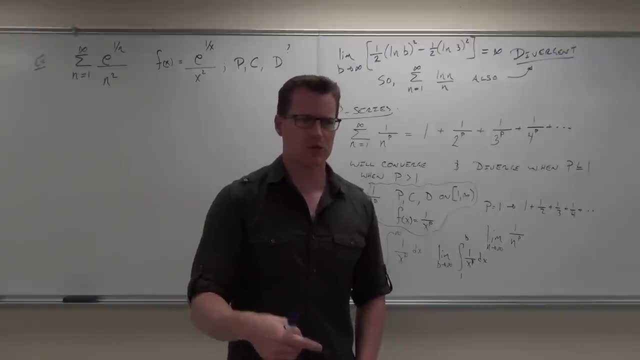 you can always show decreasing of functions by showing the derivative: is what Decreasing functions? Decreasing functions always have derivatives that are Negative, Negative. So if we can show that this derivative is negative for our interval, we show that this is decreasing. 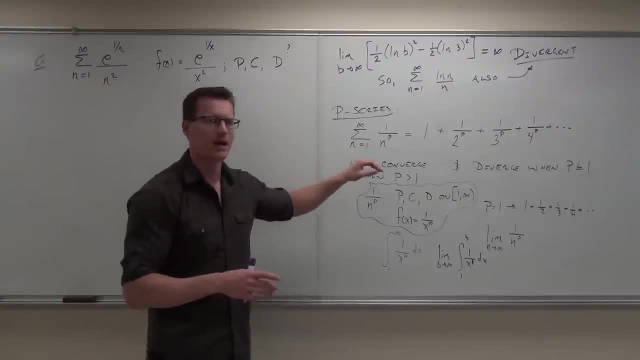 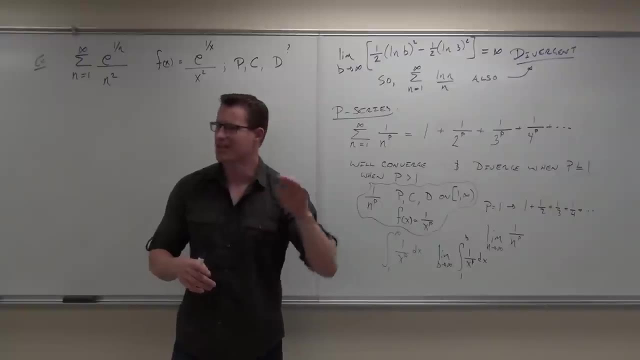 on the entire interval. Now here's a little caveat. I showed this before. If it's not decreasing on the entire interval, is there a point where it is decreasing? If there is a point where it's decreasing- like last time it was decreasing after e. 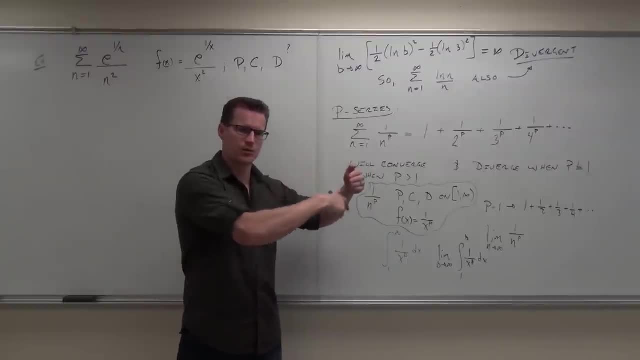 Remember that If there's a point, then we can subtract a finite number of terms from our series and get the same result. They're both going to converge or diverge, But it's just to find out whether this thing is decreasing on a certain interval. 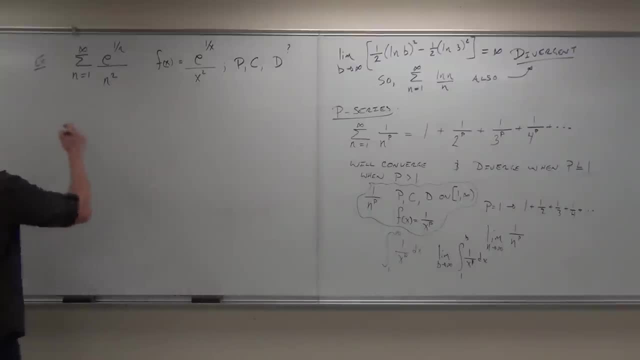 and that's all about the derivative. So we're going to take the derivative. I'm going to do it very quickly. I know you guys know how to take derivatives. so if you do the derivative, remember it's not Lobital's. 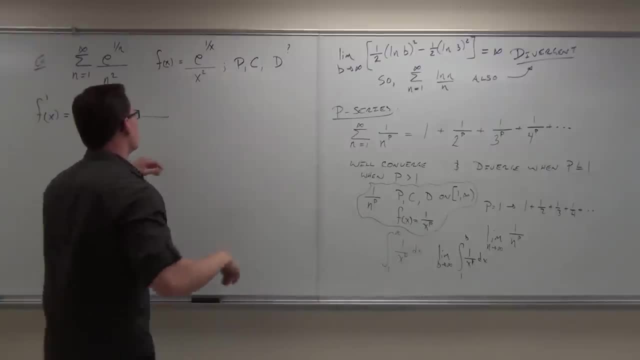 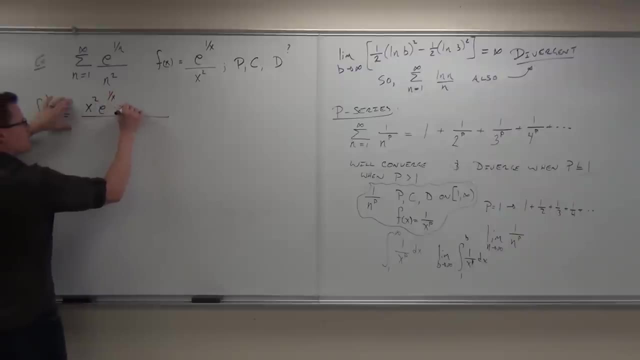 It is a quotient rule. It's low d high minus high d low. square the bottom away you go. So low d high gives you x squared e to the 1 over x times negative x squared- sorry times 1 over x squared. 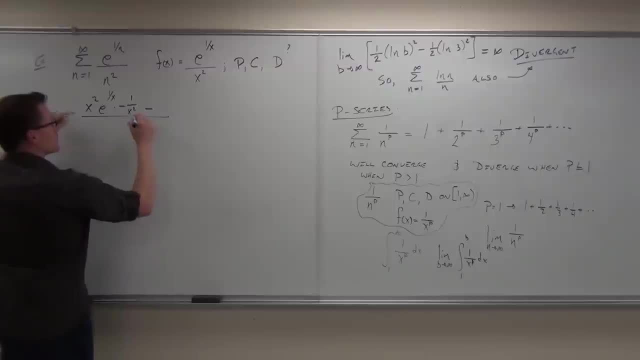 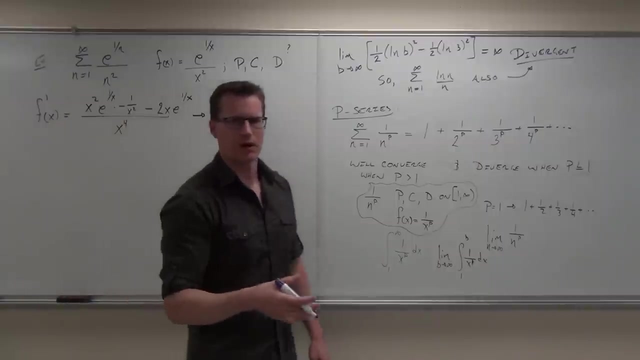 Negative 1 over x, squared Minus. so that's low d high minus, high d low, square the bottom and away you go. Spend some time on your own if you need to and do that derivative on your own. I'm doing it really quickly, of course. 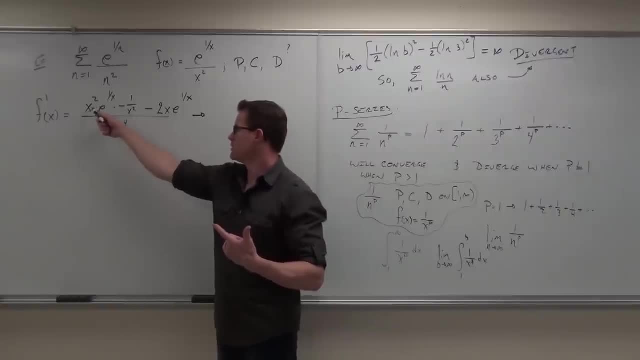 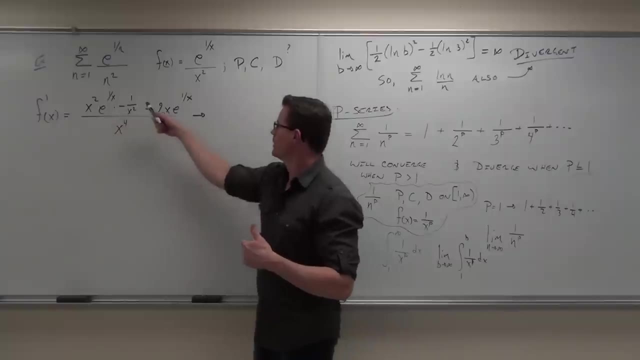 but do you have a chain rule at work here? We'd have low derivative of e to the 1 over x is e to the 1 over x times negative 1 over x squared by the chain rule. Keep the high one, derive the low one. 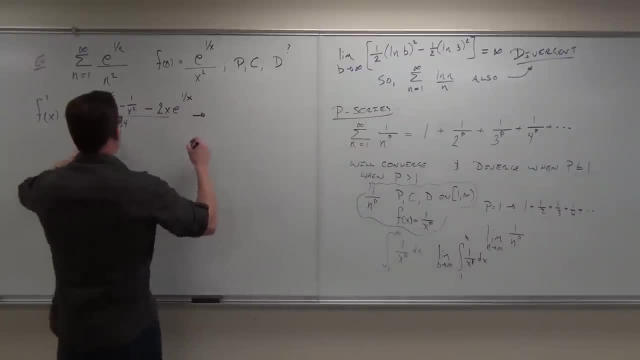 you get 2 x e to the 1 over x and then square the bottom. So if we do this we're going to get negative e to the 1 over x, minus 2 x e to the 1 over x, all over x to the fourth. 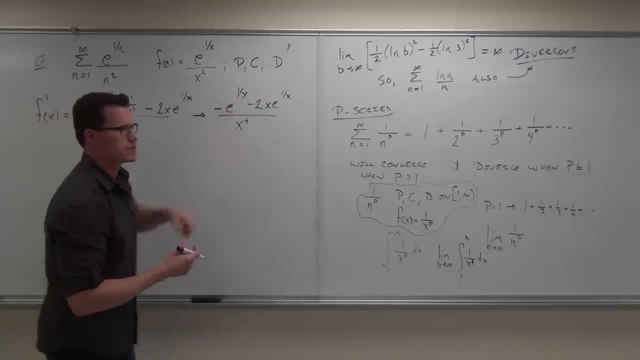 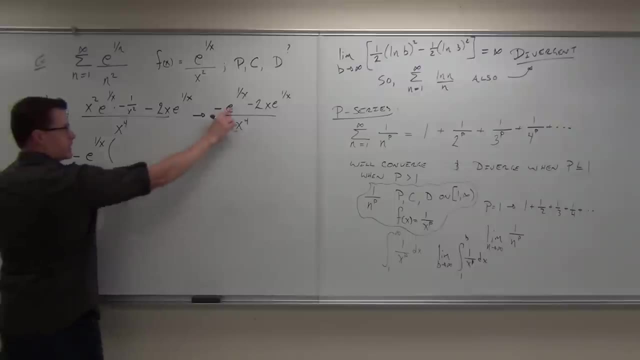 Let's make this a little nicer. If I factor out negative e to the 1 over x, if I factor out negative e to the 1 over x, what we're left with is positive 1 plus 2 x. Can you verify that for me? 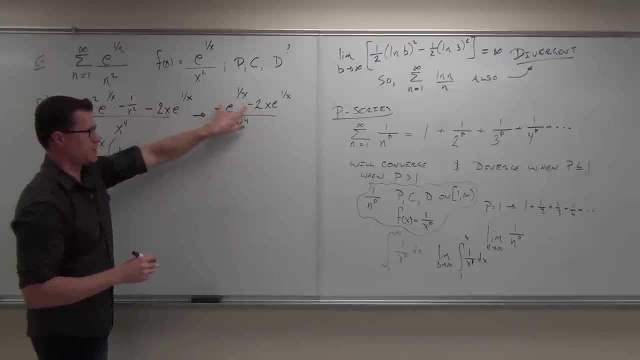 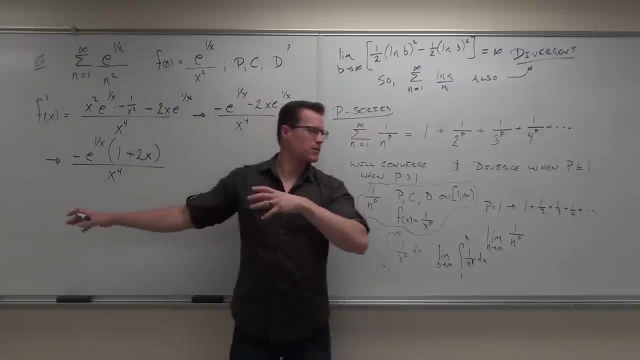 that if I factor out negative e to the 1 over x, I get positive 1 plus 2 x. Can you verify that? Yes Over x. to the fourth, Tell me what we just found: Derivatives. Derivatives show decreasing when they are. 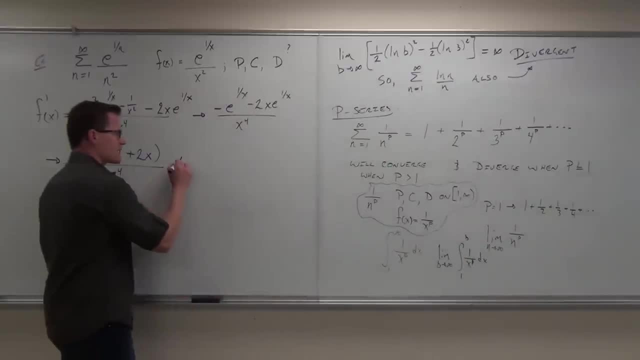 Negative. Okay, so what we got to ask our question is: is this thing negative? is this thing less than or equal to 0, on my interval? Well, let's think about it. All you're trying to do is show it. 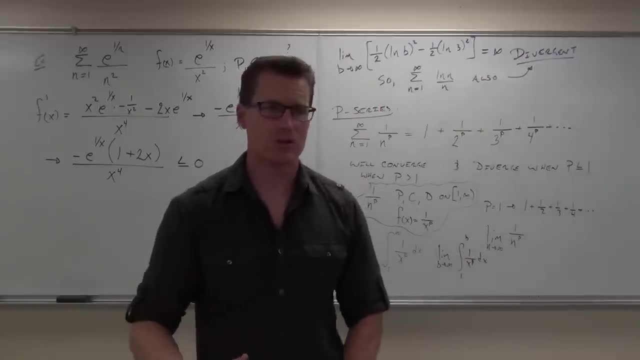 You're just trying to show that it is decreasing. If you can't show it, if it's not decreasing, you can't use this stuff. So hopefully it's decreasing for you. Let's see Where does our interval start here? 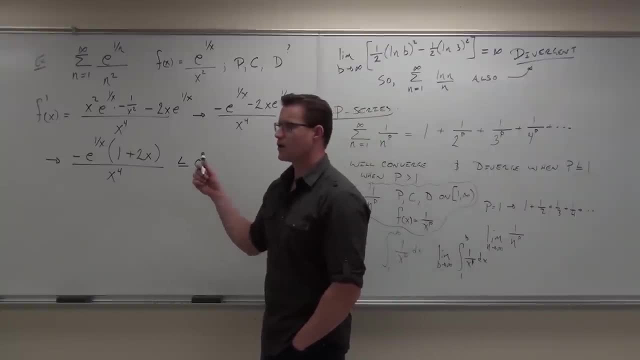 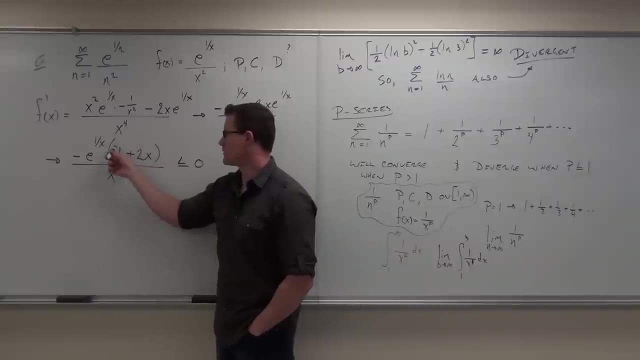 It starts at 1.. Is this decreasing on 1?? Well, let's think: True or false. this is always positive. True or false. This is always positive if x is greater than or equal to 1.. I don't care about negative numbers, because my series doesn't start negatively. 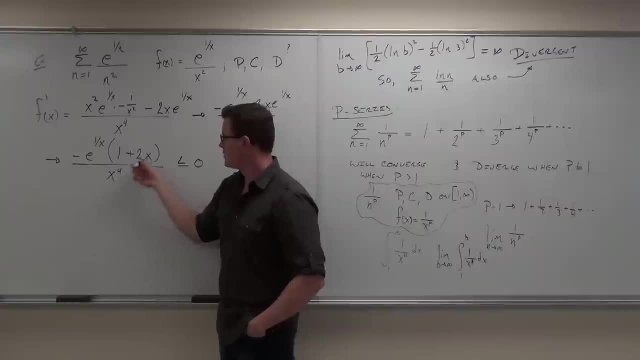 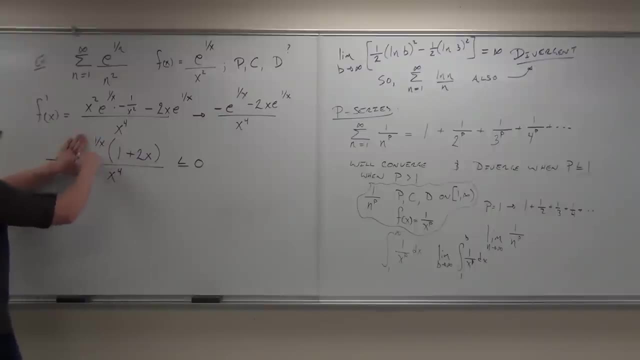 It starts at 1.. So this is always positive, right, This is always positive. Now think about this one: Is this always positive without the negative? Is this always positive? E to any power is always positive, So we got a positive. 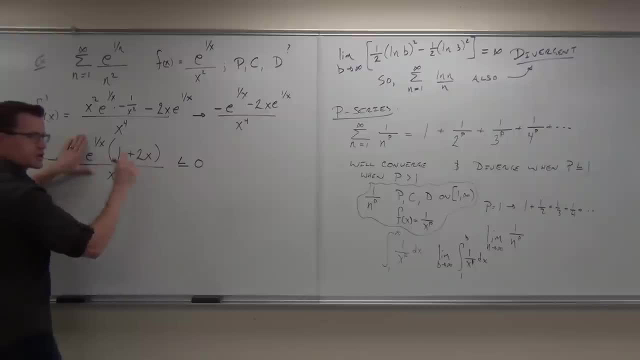 We got a positive. We got a positive. So you're telling me, for any value of x, this expression will be positive, correct? Yeah, Are you sure? Me too, because that's positive, that's positive, and that's positive when x is greater than 1.. 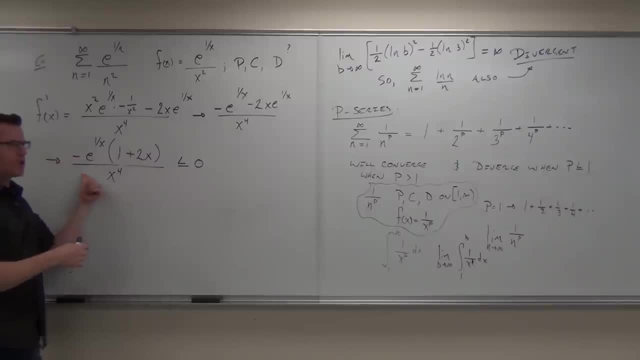 What would that do? Negative. So is this always negative? for x is between 1 to infinity. Yes, This is positive. for x equals 1 to infinity. This is positive. for x equals 1 to infinity. This is positive. for x equals 1 to infinity. 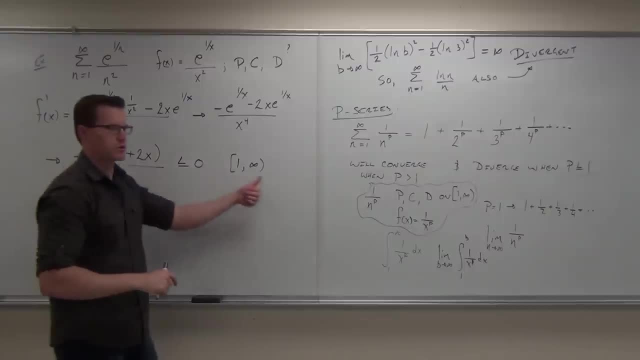 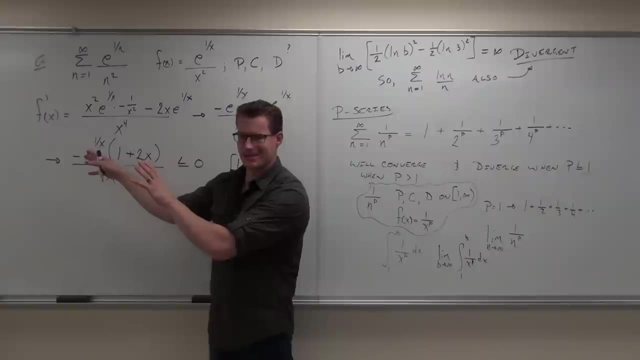 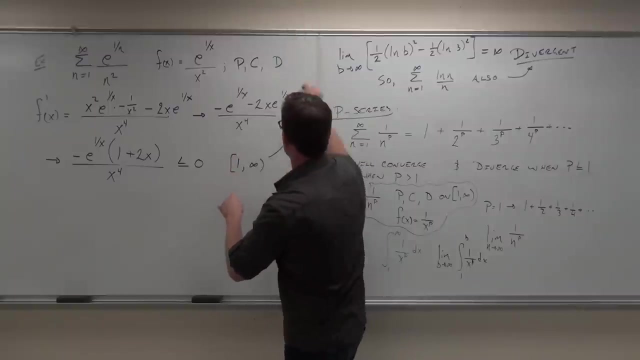 Therefore this whole thing is negative. when x equals 1 to infinity. Because my first derivative is negative on this interval. because my first derivative represents increasing or decreasing. because my first derivative is negative on this interval, it shows that it is decreasing on this interval. 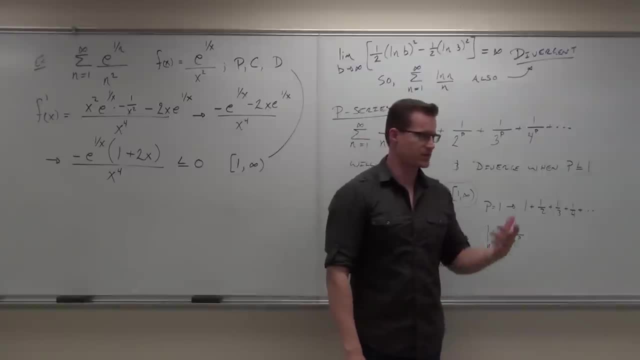 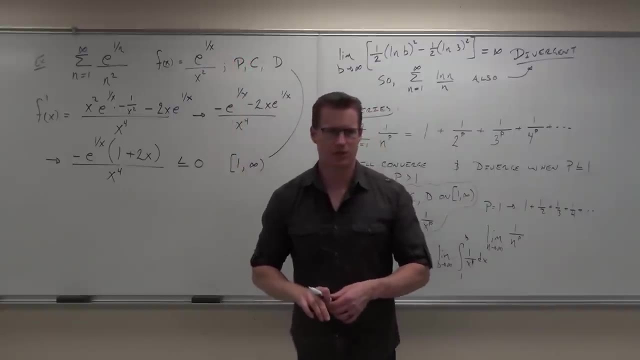 That's the idea. That's the hard part. The rest of it is pretty easy. Show me if you understand that part. Do you feel okay with it? Can you go ahead and try to do the rest of this? Sure, Go for it. 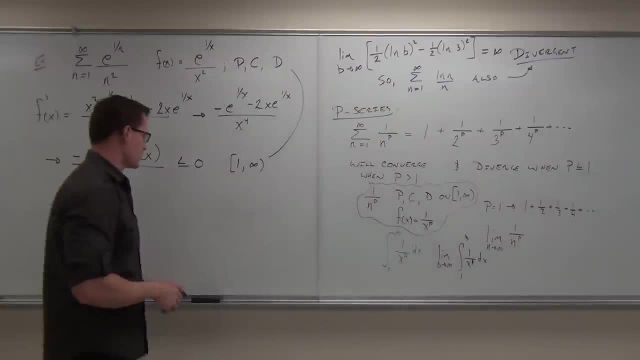 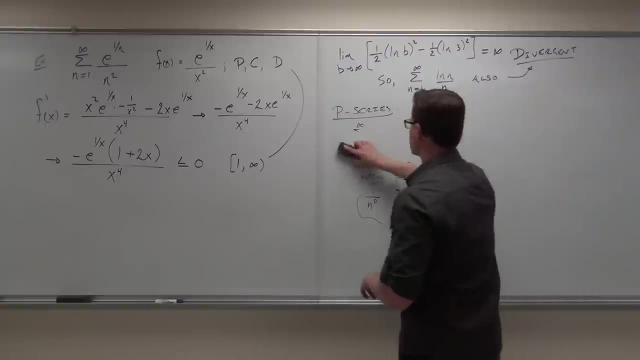 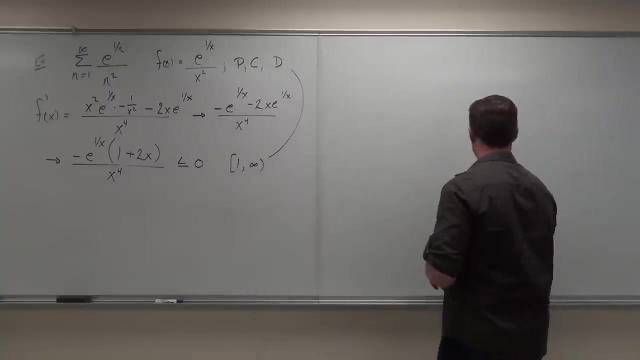 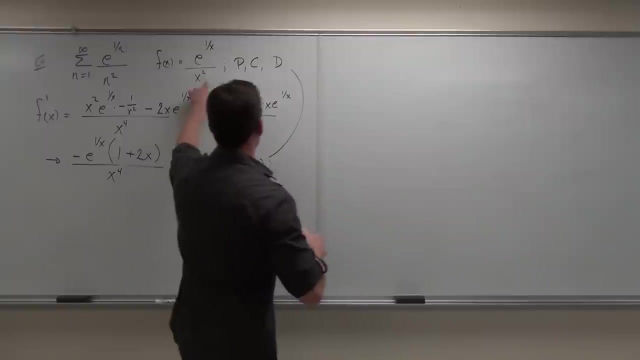 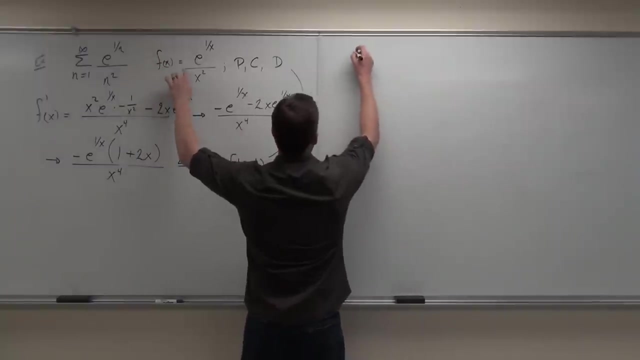 Go for it. See that you still have the chops to do integration. So, because this function is positive, continuous and decreasing, and because it's based on the sequence from which we get our series, the integral from 1,, whatever our interval is, 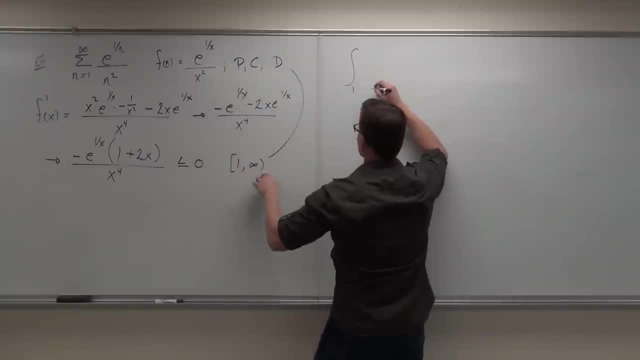 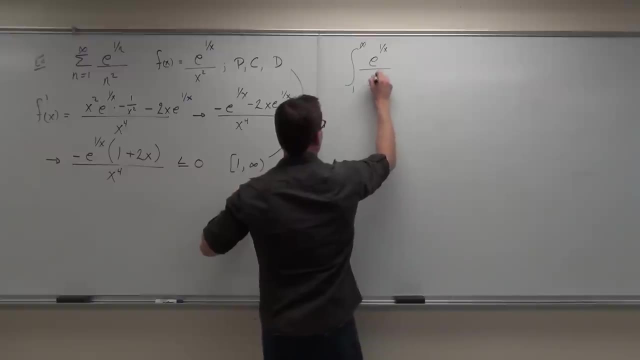 where it is positive, continuous decreasing, our interval is 1 to infinity. where that happens, Our integral, from 1 to infinity, of e to the 1 over x over x squared dx, will have the same result as our series. 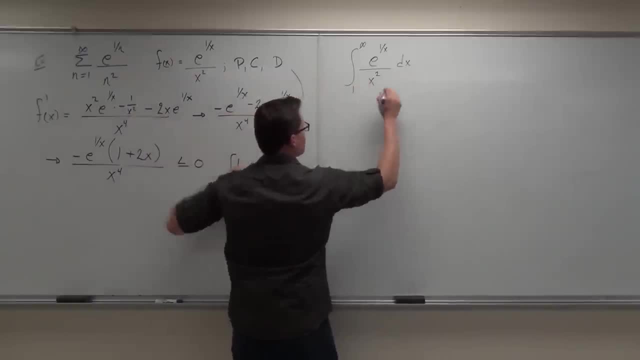 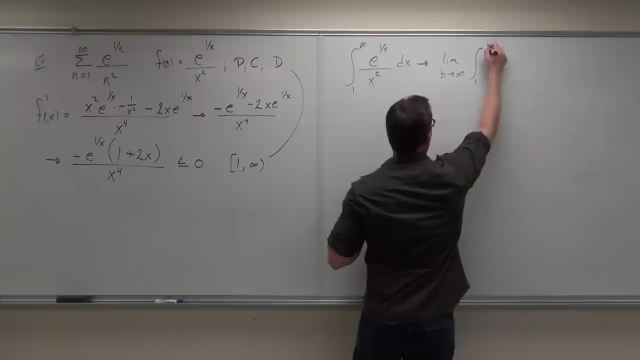 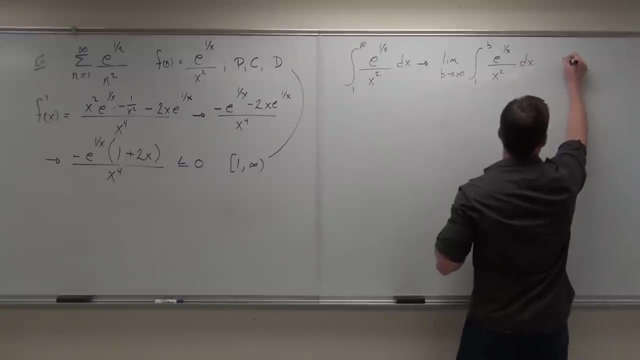 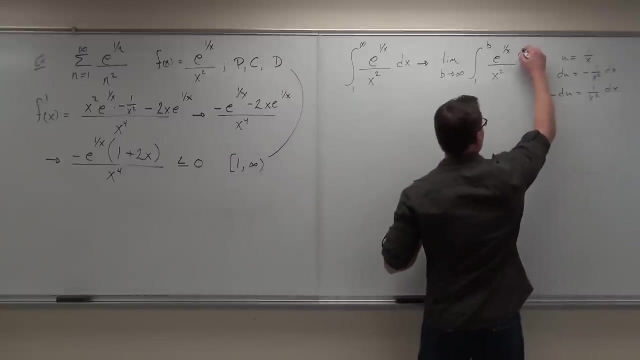 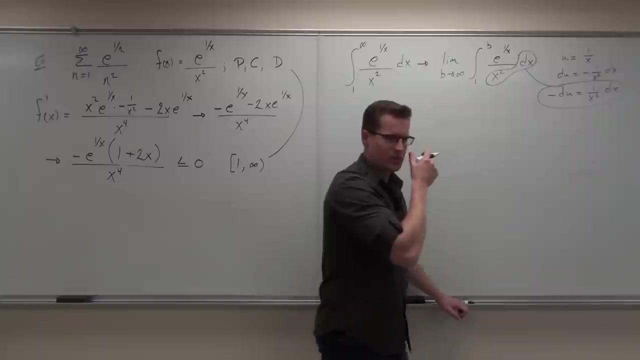 If this is convergent, our series is convergent. If this is divergent, our series is divergent. Of course, what we know is that this is an improper integral. We must treat it as such. Yay, Did you find the appropriate substitution? 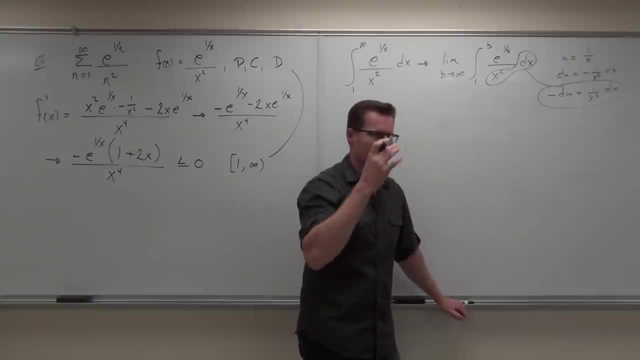 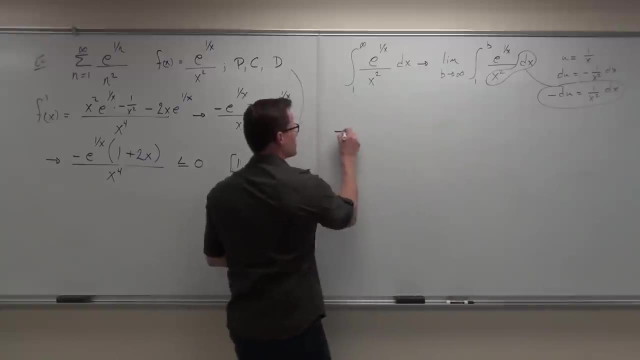 Not so bad, right? Not so bad, It's just a substitution. Most of these things are going to be just substitutions for you, Not horrible. If you do u equals 1 over x, then our integral becomes from 1 to b, e to the u. 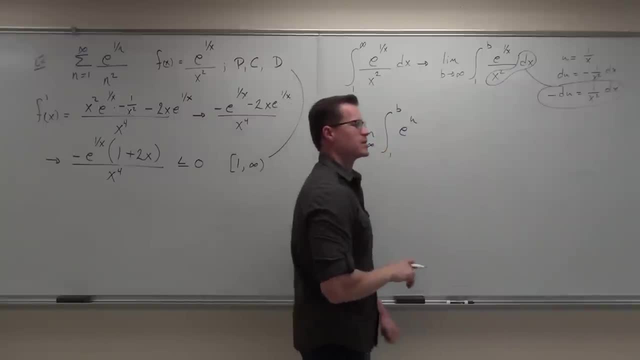 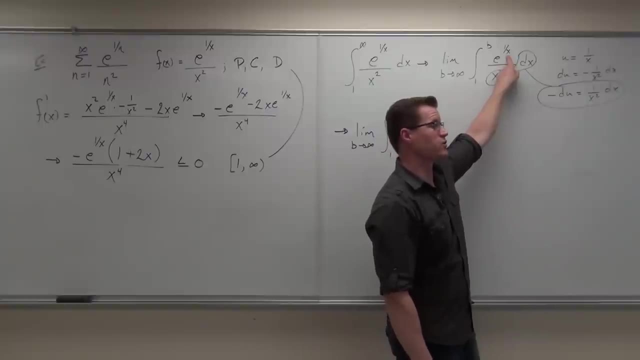 Now what else happens. Let's see if you did this right, You guys. okay, with the, u equals 1 over x. The reason why we see this is because the derivative of 1 over x is 1 over x, squared somehow without the constant. 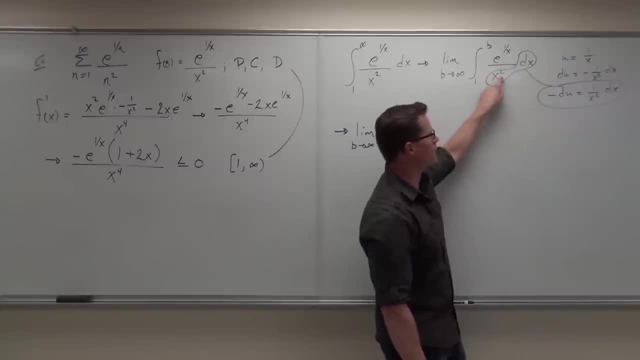 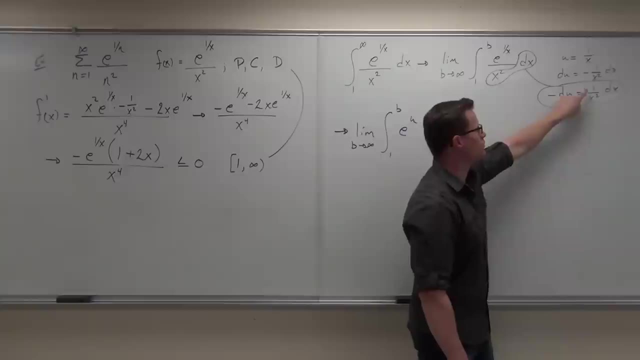 So that derivative is up there. This counts as a 1 over x squared. So u equals 1 over x. du is negative 1 over x squared, Not a problem, Move the negative over here. Negative du equals 1 over x squared dx. 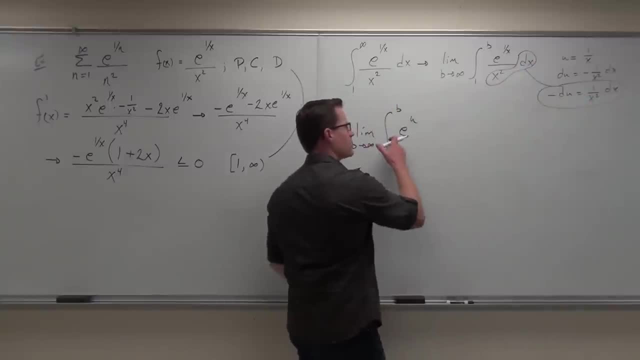 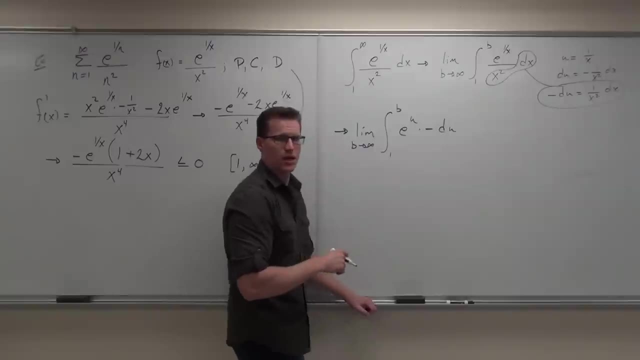 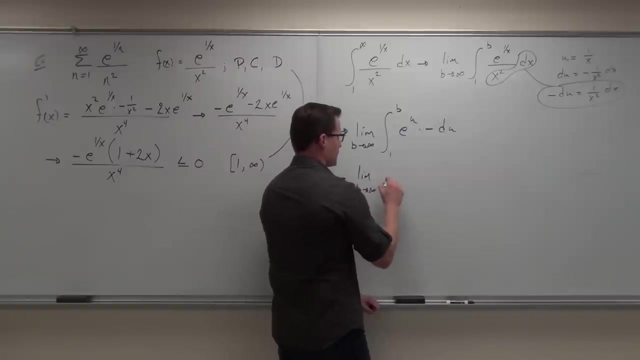 That is this piece right here. So what is after my e to the? u? Negative du Cool, That's about the easiest integral I can think of. So this is a limit, as b approaches infinity, of what is it going to be Negative? 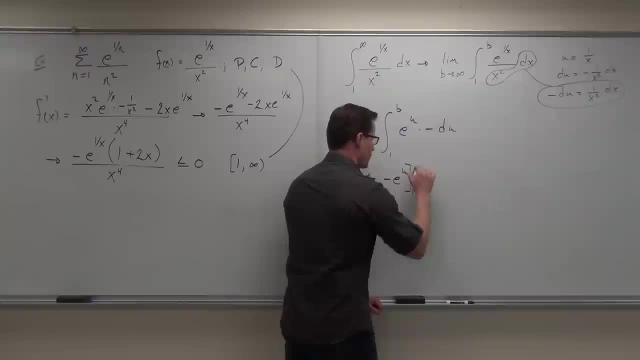 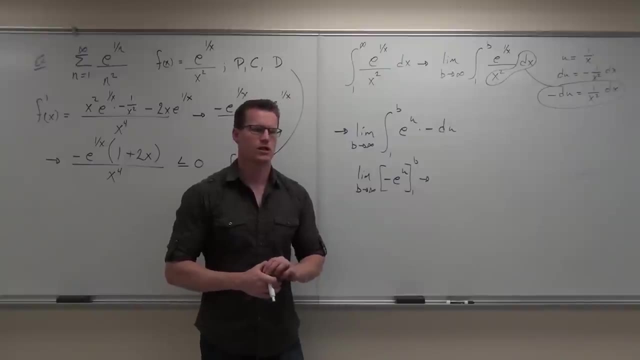 I like the negative. what From 1 to b? Now there's a problem here. Do we want to plug in b and 1 right now? No, If you do this, you're going to get a divergent limit. It's going to look like it's different. 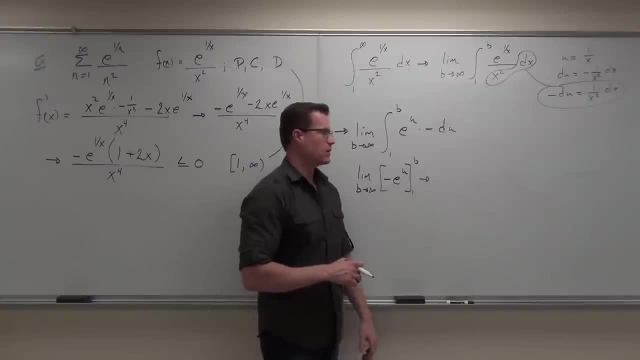 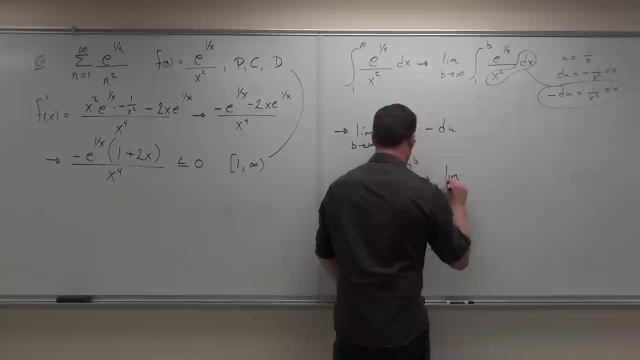 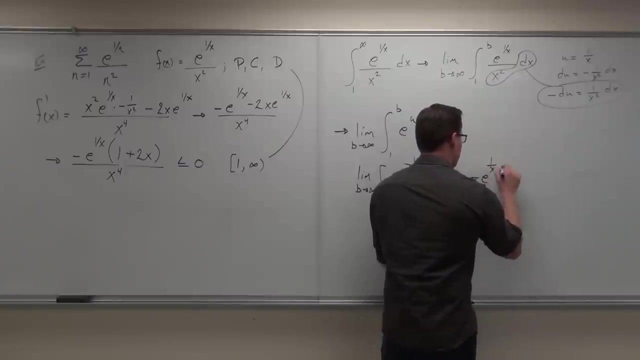 If you plug this in, what's the big problem with doing this? These aren't in terms of u, They're in terms of x actually. So for us we absolutely must substitute back in before we evaluate our limit. So this has to be negative e to the 1 over x. 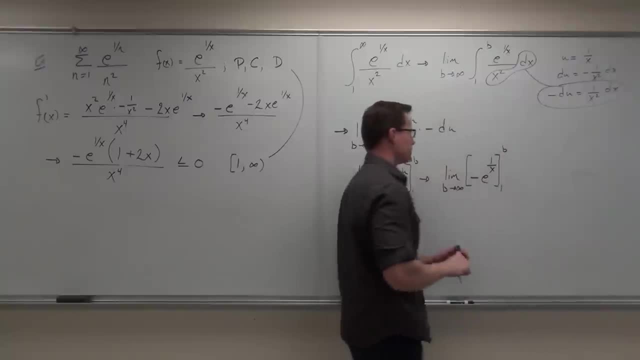 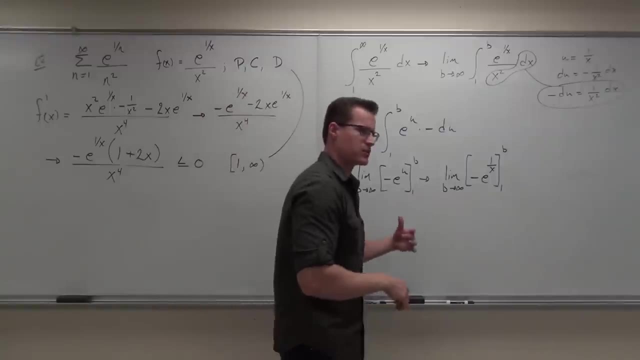 That's going to make a big difference. Did you catch that? You've got to make sure you substitute in, Make sure your bounds match your variables. If your bounds are in terms of x, which they will be your resultant from your integral, better be in terms of x as well. 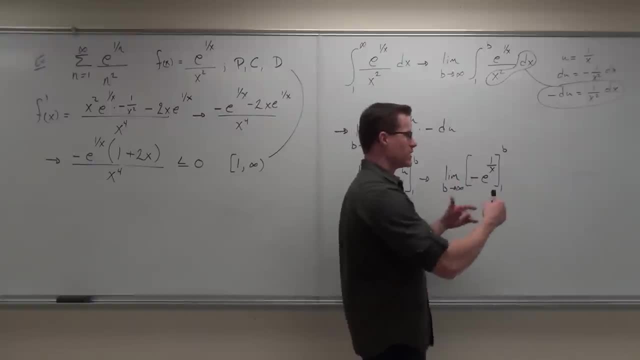 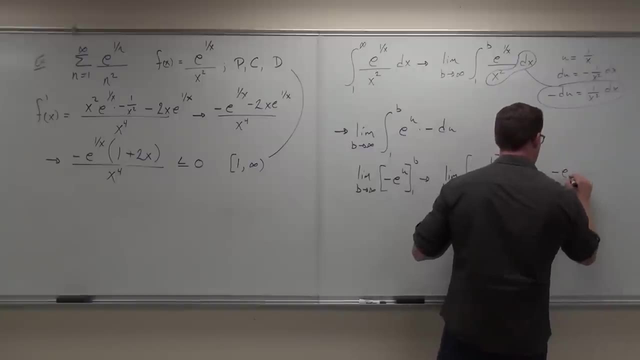 So we need to make sure we substitute back in. if we've done a substitution, Well, what that means is we've got a limit as b approaches infinity: negative e to the 1 over b, minus negative e to the 1 over 1.. 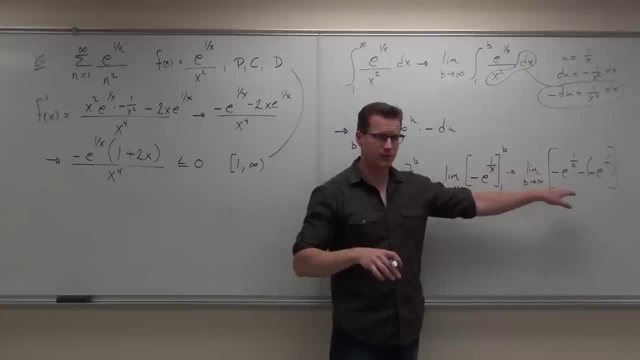 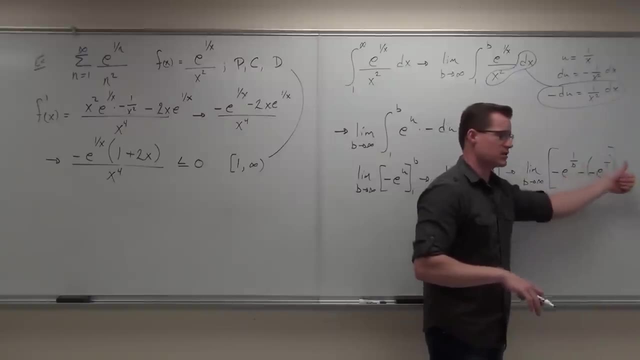 Let's see what we got. First of all, did you get the same thing as I did. Good for you, That's fantastic. How much does this all make? This is going to be plus e somehow. Well, minus negative is plus e to the first is e. 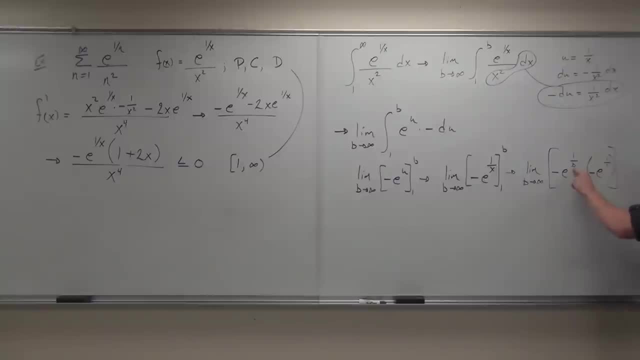 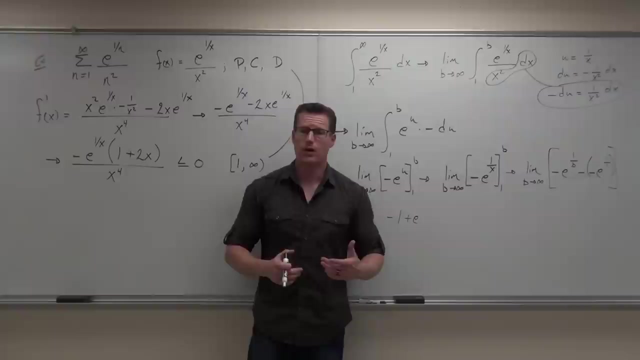 Let's do this: How much is b going towards? How much is 1 over infinity? How much is e to the 0? 1. Negative, 1. Negative. 1 plus 1 is 0. So this whole thing equals negative 1 plus or e minus 1.. 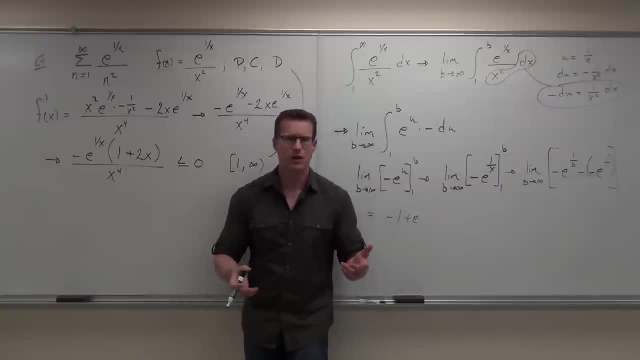 Do I care that it's negative, 1 plus e or e minus 1?? Well, not so much, because it doesn't necessarily give me my sum for my series. but what's it tell me about this limit? This limit is It equals a number? 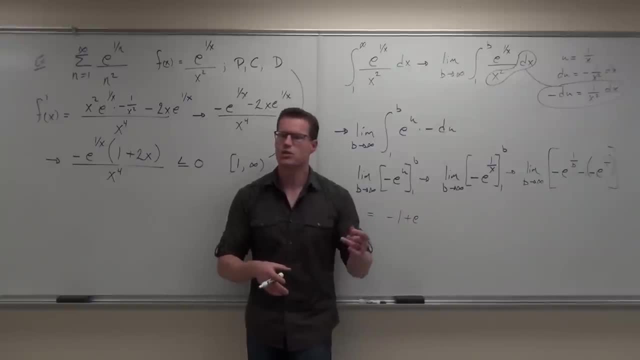 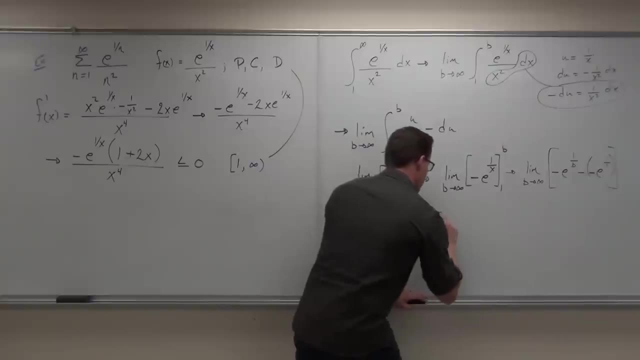 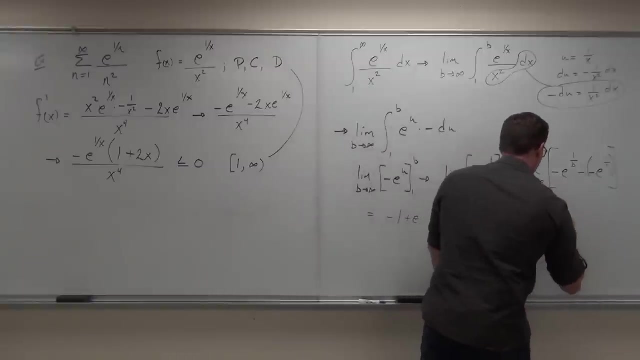 It doesn't equal infinity, It does not exist limit, It converges. So what's it? tell me about my series from where I got this? So, by the integral test, this is convergent, So this converges, So my series also converges.